So for. And gate. Good. When. Am. both inputs are high. Output will also be high because we know. When we enter the inputs in the output will also be. 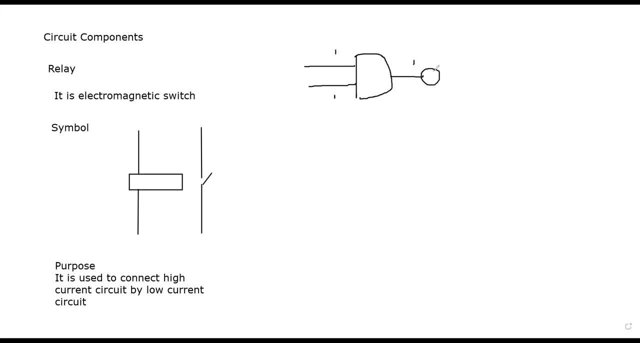 so if we connect a lamp here so what should be the state of the lamp one one is once the state of the lamp the lamp should be on but sometimes the lamp it should be 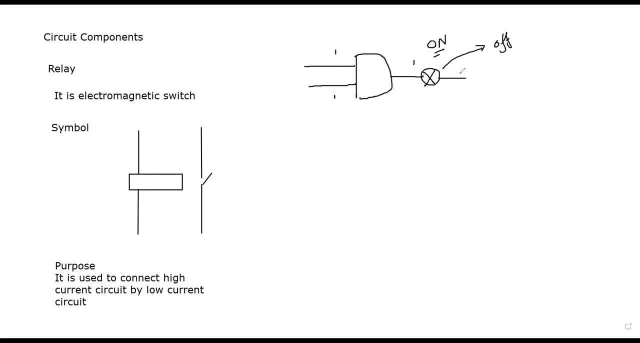 on but it remain off what is the reason why the lamp will remain off even though the output should be high like for and gate if we have an and gate when both inputs are one the output is one so lamp 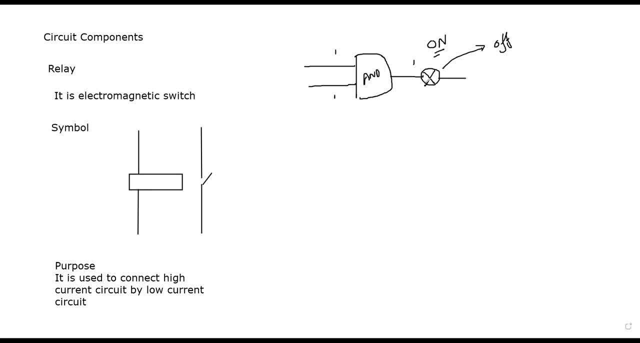 should work but even the output is high but the lamp is not working why the lamp is not working because this one is not showing the magnitude or amount of current or voltage produced maybe 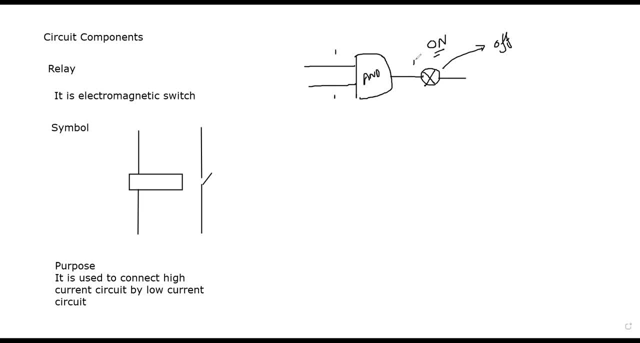 the voltage or the current which is passing through this lamp is not sufficient to light up the lamp and for and gates for logic gates normally the voltage and the current which is produced by these logic gates it's a small voltage 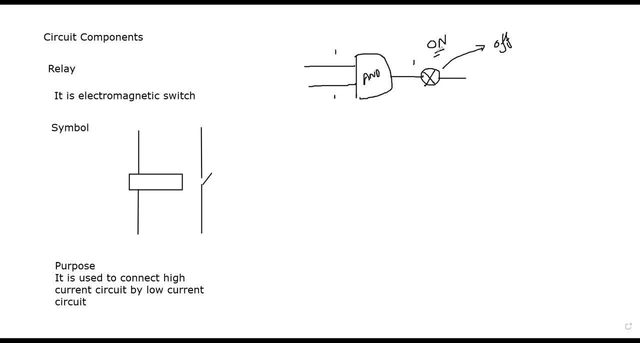 what happened one and one the output should be one so lamb should be on but what when we observe it is off why the lamp is off because the output current the output current or the voltage is not sufficient 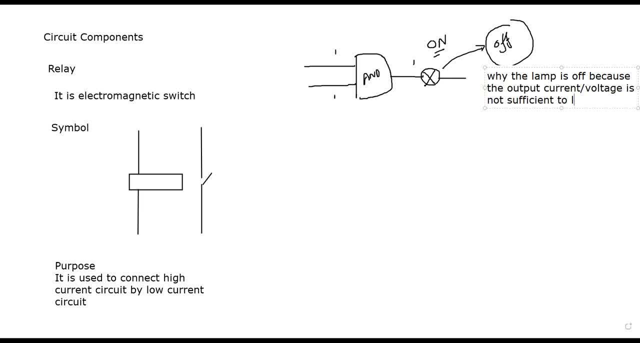 because the lamp already is off so what example are those light up is that each of the down the current of 6 items on a person to light up this lamp so in that case what we can do we can connect a relay here how we can use a relay example 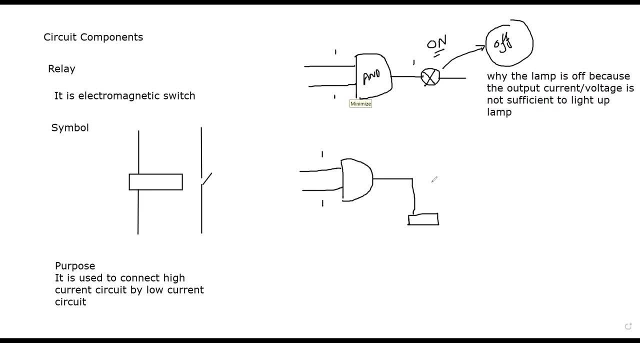 So, we have a relay electromagnetic switch. And with this second part of a relay, we connect the lamp and we connect a high voltage supply. So what happened one in one the output of the AND gate will be one. 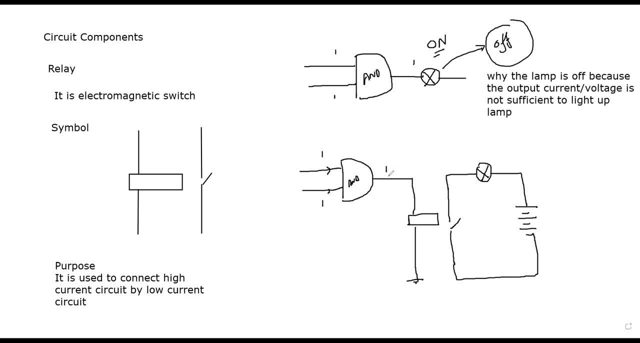 So when output is one means there will be a current which is passing or output current will be there. 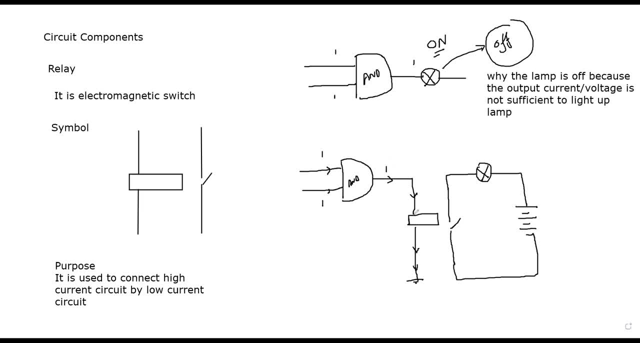 When there's an output current, what will happen? Because this is an electromagnet. Electromagnet means when the current is passing through it, it will behave like a magnet. So this electromagnet, as it is magnetized, this part of a switch is made up of iron. So it is attracted towards the electromagnet. So as it is attracted towards the electromagnet, the switch will close. As the switch will close, the high current starts to flow through the second circuit. 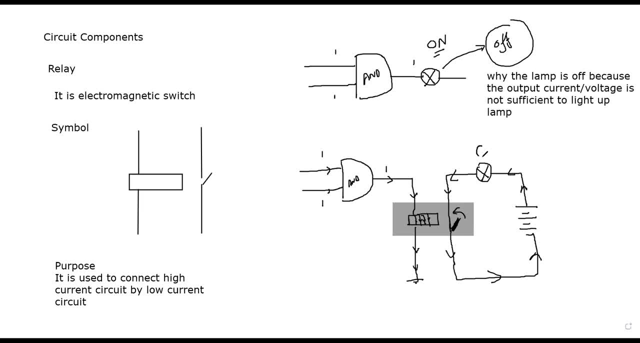 As the high current starts to flow through a second circuit, what we will observe, we'll observe this lamp will be on or this lamp will light up. 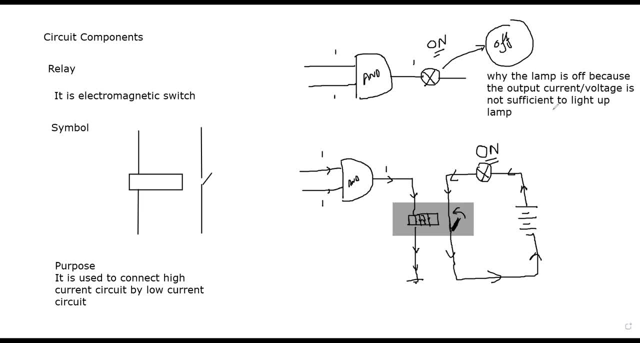 So what is the advantage of the relay? Normally when the circuits are operated at a low voltage and we want to connect a device 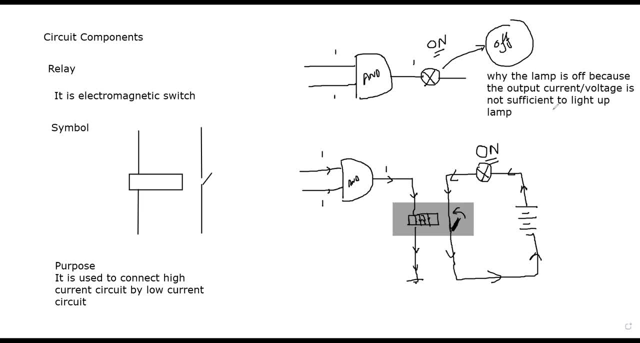 which we need a high, which required a high voltage. So how we can connect these two things together, a low voltage circuit and a high current circuit, we can. 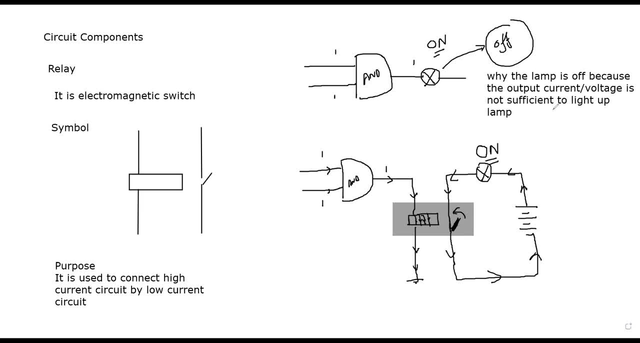 For high voltage circuit, we can connect a relay between them. So what will be the advantage of the relay or the electromagnetic switch? 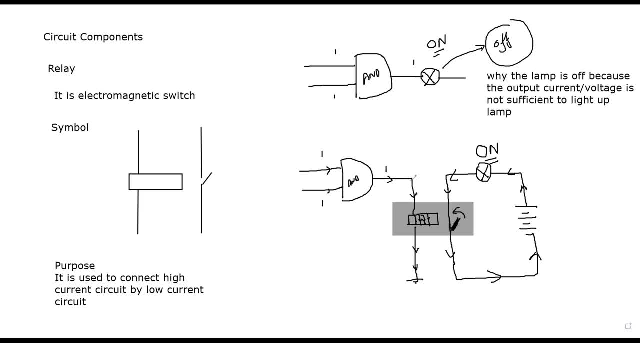 So when the current is there, when the input is high, when the output is high, the current will pass through the relay, which magnetize the relay coil. 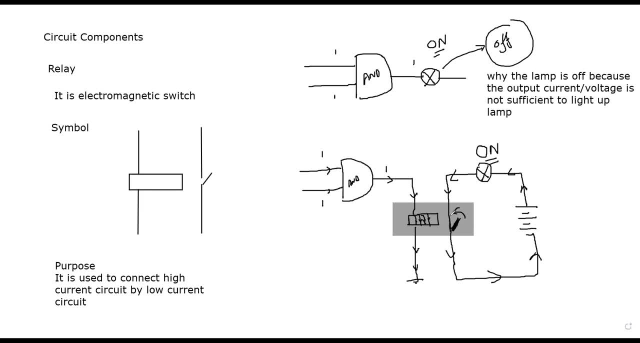 As this part is magnetized, it will attract the piece of iron which close the switch. As the switch is closed, the high current or high voltage in the second circuit will operate the device or the component which we want to work. 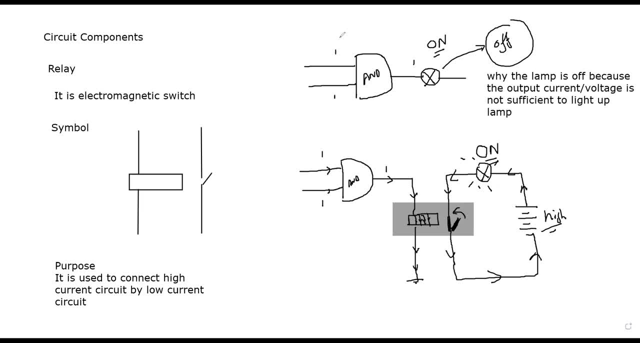 If I directly connect this lamp to AND gate when both inputs are high, the output should be high. Output is high, but that output current, this one is only showing the state like it is showing a state that it allow the current to pass. But maybe the current which was passing is too small. That is not sufficient to light up this lamp. 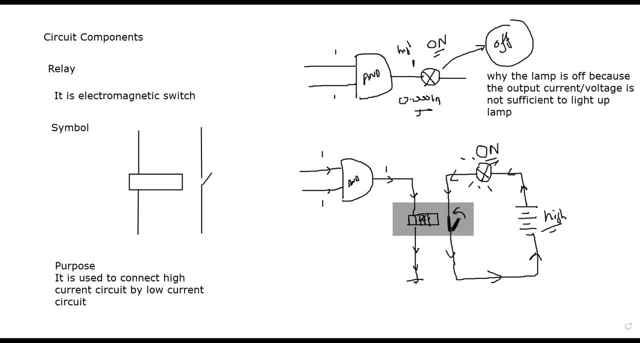 That's why what we can do, we can connect a relay. Because relay can be operated by a low current or low voltage circuit. 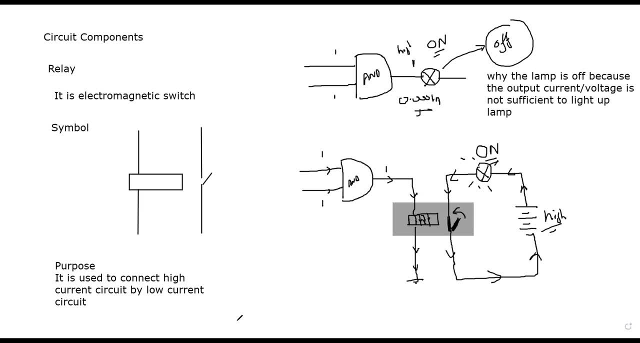 Is it clear the working of the relay? 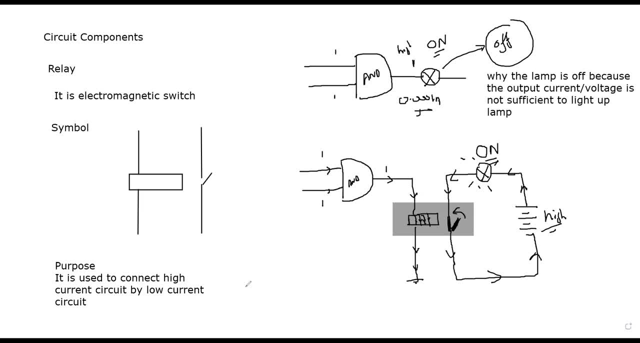 Okay, thank you very much. Thank you very much. Thank you very much. Thank you. 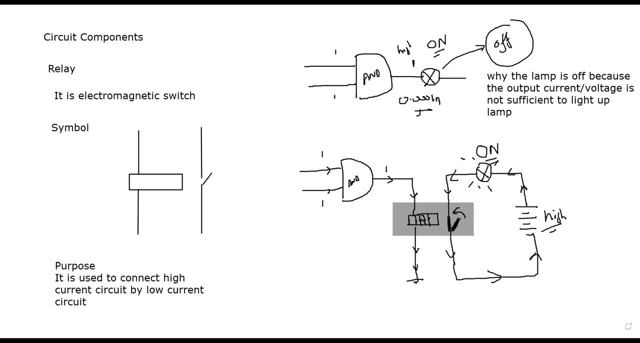 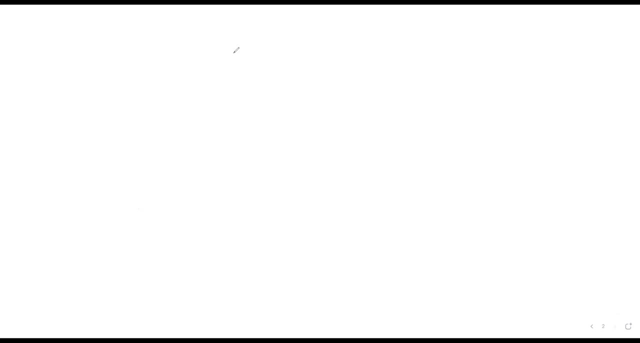 Thank you. So example, we have the OR gate. 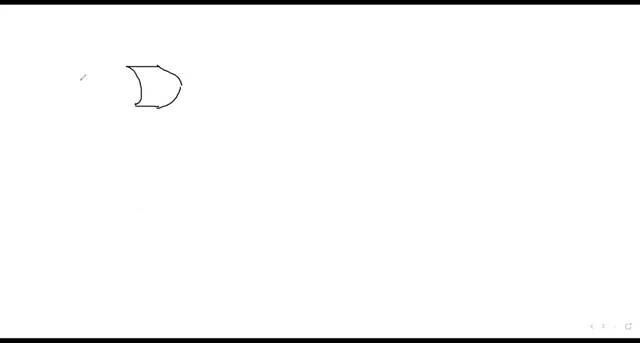 So here we have the input is 0.1 ampere and this one is 0 ampere, means one of the input is high and the other input is low. 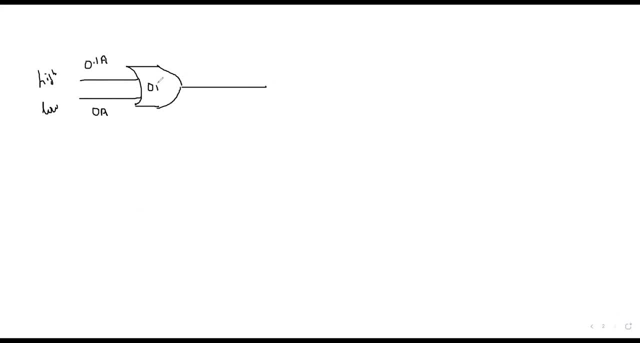 What will be the result output for OR gate? One of them is high, high means that this current is there, the other one is low, no current. What will be the output of OR gate? What will be the output of OR gate? Okay. 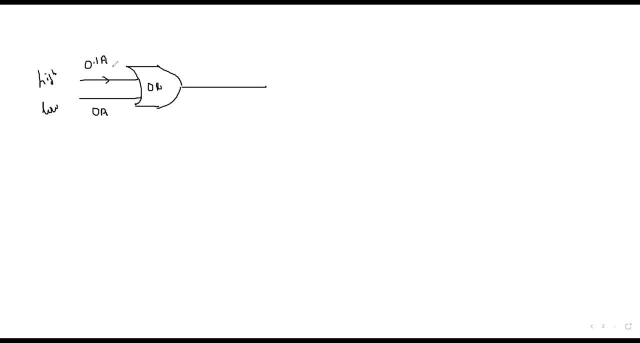 Now, when input is high and output is low, what will be the output of OR gate? So output will be high. 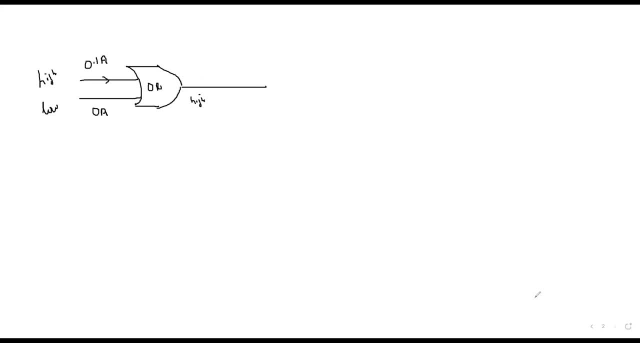 Output high means it will allow the current to pass. So it will allow, for example, 0.1 ampere to pass. But as I connect a lamp here, so this lamp should be on. Okay. 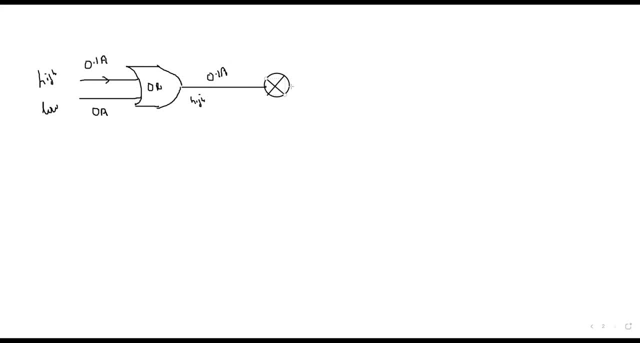 on. So if this lamp should be on, but when we observe this, it remain off. So as it remain off what it shows, it shows that this 0.1 ampere is not sufficient to light up the lamp. 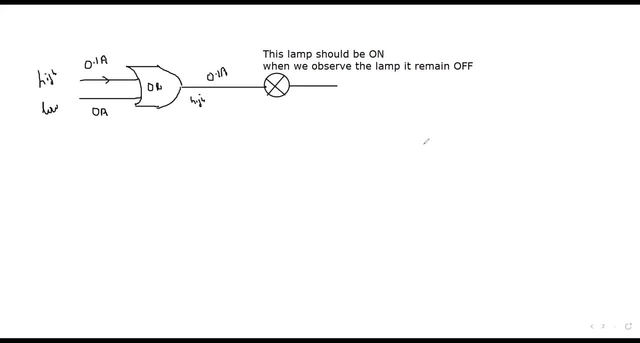 It need a more voltage or greater current to work. The current is too low. So what we can do instead of directly connecting this lamp to the output of the OR gate, we can connect a relay and connect a high voltage supply. Like here it is 0.1 ampere. So one of the input is high and the other input is low for OR gate. So the output example is 0.1 ampere. It's high. We connect a relay coil. So when 0.1 ampere is there, this will magnetize because current is having a magnetic effect as well. So this will magnetize this relay. 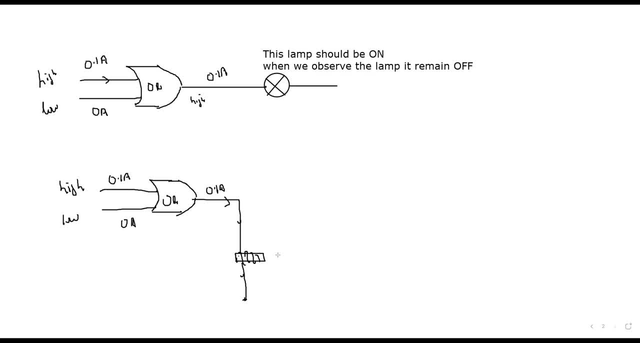 This will magnetize the relay coil. So a switch, the part of the switch is attracted towards the relay coil. And when you have this lamp connected to the high voltage supply, like for example, say a 20 volt supply or a 40 or 220 volt supply is there, which can give you a more current, greater amount of current. So as a relay magnetize, this magnetic field attract the piece of iron. This is made up of iron. So as iron is also a magnetic material as well as a conductor. So it will close the switch as it will close the switch, the voltage or the current is higher. Example, it is producing a three ampere. So this three ampere is sufficient to light up this lamp. So what will happen? This lamp will be on. If you use a button, it means you have to operate like you have to switch on and off by yourself. It will automatically according to the circuit, it will not work. Then you have to be there next to the circuit. And when you see the output of our gate is high, then you will close the switch. And if output of our gate is low, you will open the switch. So then you have to operate. It is electromagnetic switch. If there is a current in the circuit, the other switch, the other circuit will also work. Is it clear? The working of the relay electromagnetic switch. Any doubt in this part? 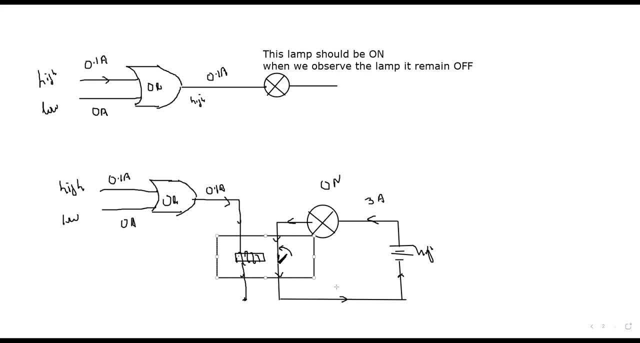 This is electromagnet. Electromagnet means when there is a current. No, this is not the change in the magnetic field. Okay. Okay. 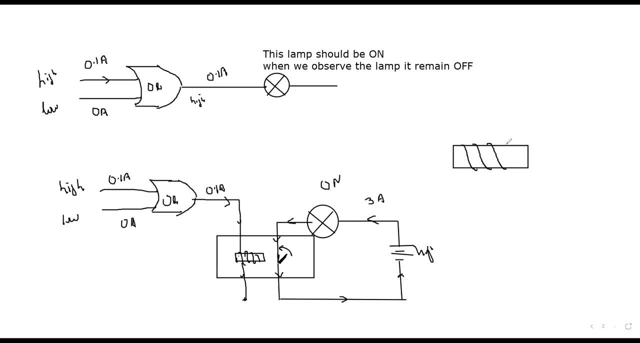 Look, you have a wire which is turned around. This is the relay coil. So as there is a current passing through this coil. So what will happen using a right hand grip rule, you can identify the magnetic pole. When you catch the wire in the direction of the current, your finger shows the direction of the current and the thumb will represent north. So north is towards right. 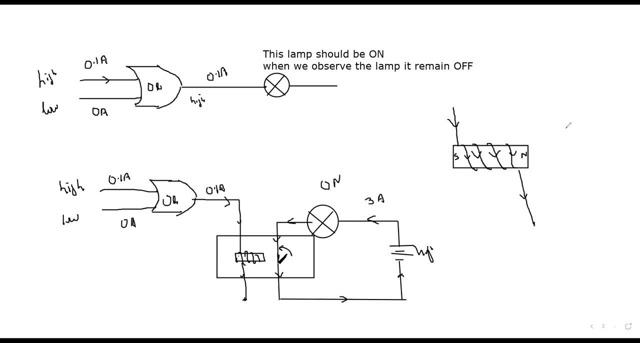 And south is towards left. So this part is behaving like a magnet. And what you have the other part is a switch. And this switch, the component, one part of the switch is made up of iron. So as it is made up of iron, if you have a magnet and there's a piece of iron, so what happened? That piece of iron is attracted towards the magnet. So as this piece of iron is attracted towards the magnet. It will close the switch. And as it will close the switch, the current start to flow in the other circuit due to the other battery is there. So the device or the component will work. Sir, I just entered. 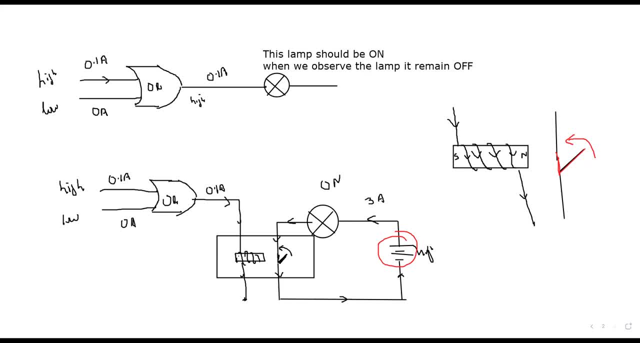 This is a relay, the electromagnetic switch. 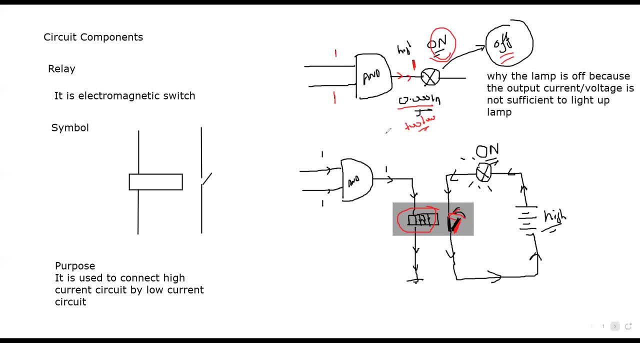 So theí This is a relay, the electromagnetic switch. Okay. 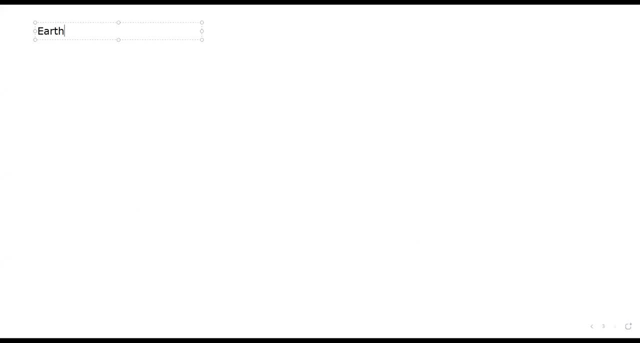 It will go around the switch. Then we also use earthing. The earthing is mainly used to avoid electric shock or electrocution. 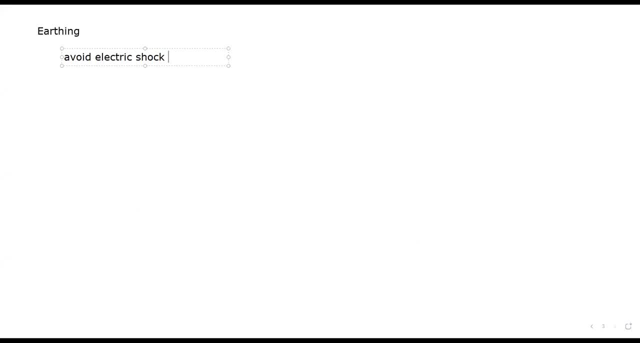 The symbol which is used for the electric shock is the adiabatic shock. Okay. 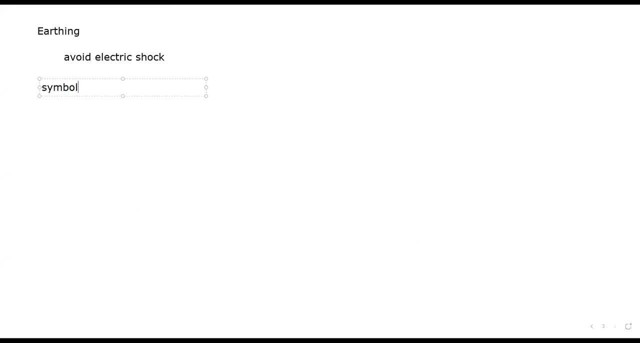 So the electric shock is used. we use for earthing a wire then horizontal lines this is a circuit symbol for earthing 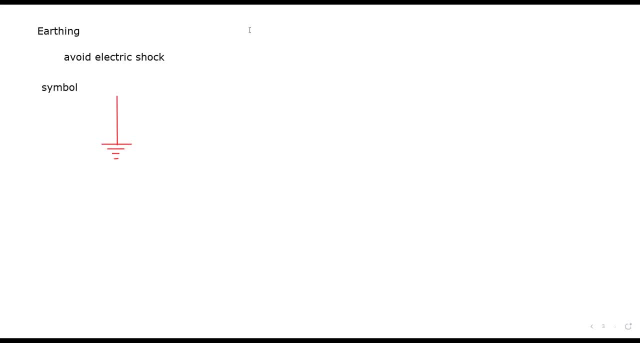 example and this is earthing is normally used for the devices which are having a metal body or the metal case because if the appliance or the device is having a plastic body plastic is insulated does not conduct electricity so a person will not get an electric shock example 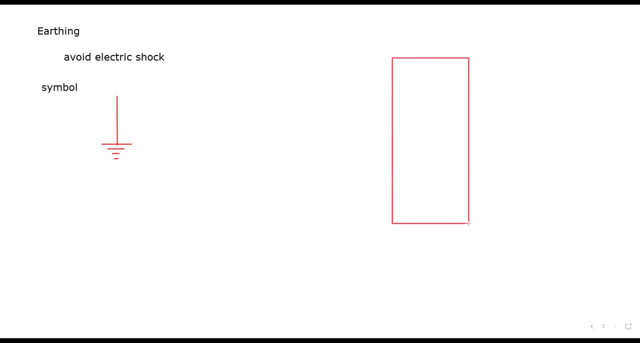 you are using a refrigerator so this is a refrigerator and it's having a metallic body so what you have to operate for working 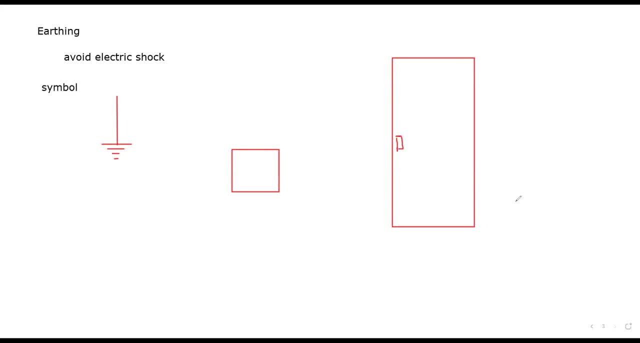 so example you have the live wire and the neutral wire so as you plug in you have the live wire and the neutral wire so as you plug in the charges start to flow the refrigerator is working this internal circuit as well for refrigerator 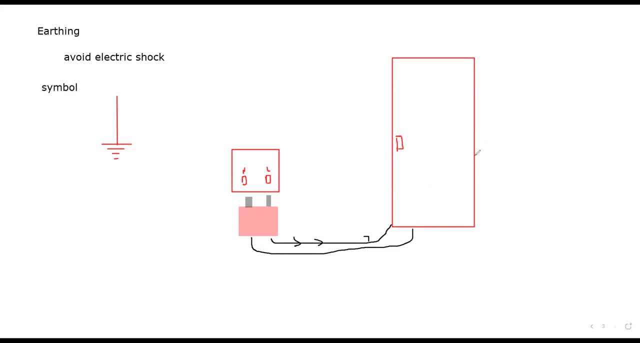 i am not drawing that now if a person will touch so what will happen the person will get an electric shock so what will happen the person will get an electric shock 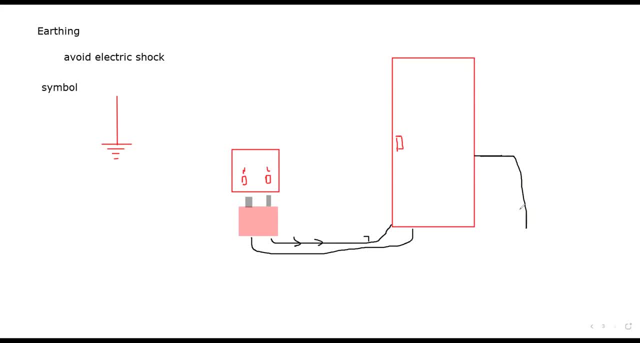 so what will happen the person will get an electric shock because so what will happen the person will get an electric shock because so what will happen the person will get an electric shock because now he is a part of the circuit so the now he is a part of the circuit so the now he is a part of the circuit so the current can flow current can flow current can flow if the live wire is touching the metal if the live wire is touching the metal if the live wire is touching the metal body body body so the charges can flow through that so the charges can flow through that so the charges can flow through that metal body metal body metal body and then passes through the least 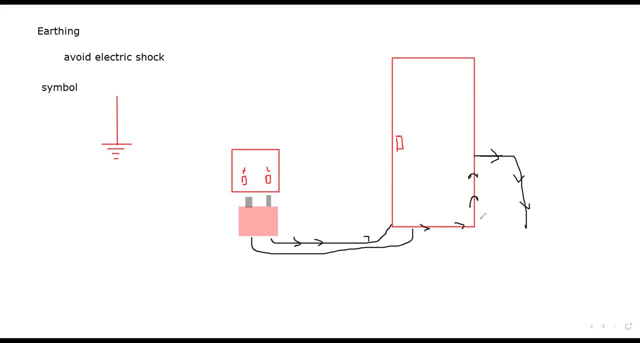 and then passes through the least and then passes through the least resistive path resistive path resistive path which is the body the human body as well which is the body the human body as well 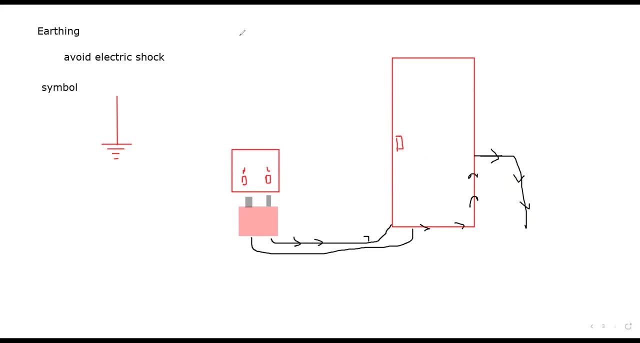 so to avoid this electric shock what we can do we can connect an earthing 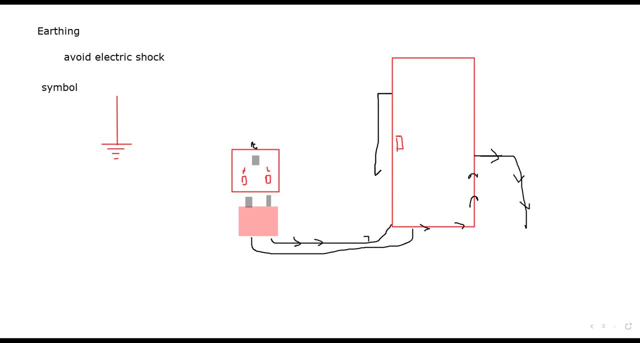 so there is also another wire which is connected 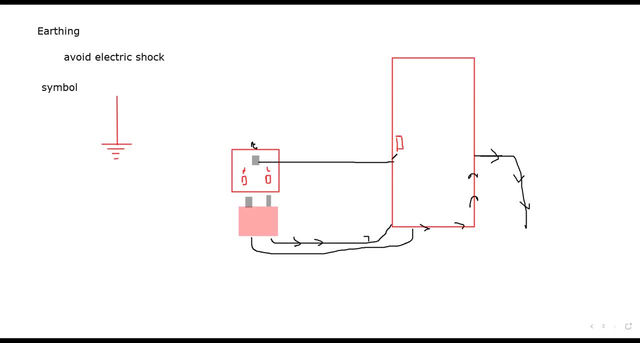 to the metal body and that's known as the earthing wire so what happens if there is a current in the live wire because two possibilities are there one is the human body through which the current can pass and another one is the copper wire copper is a good conductor as compared to human body so what happened almost all of the current or most of the current will pass through a copper wire which is connected to the earth as compared to the human body so to avoid an electric shock we use this earthing wire is it clear 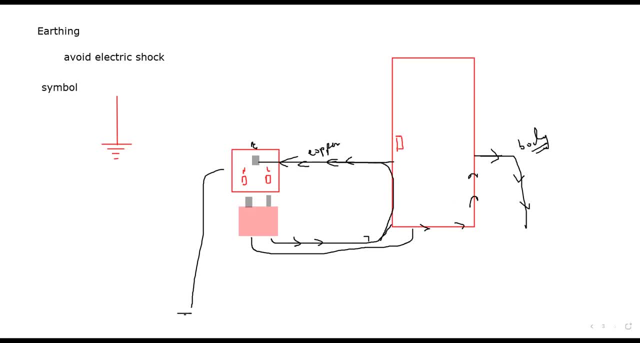 this already i discussed with you the reason just it's also a part of the circuit component that is why i discuss this again 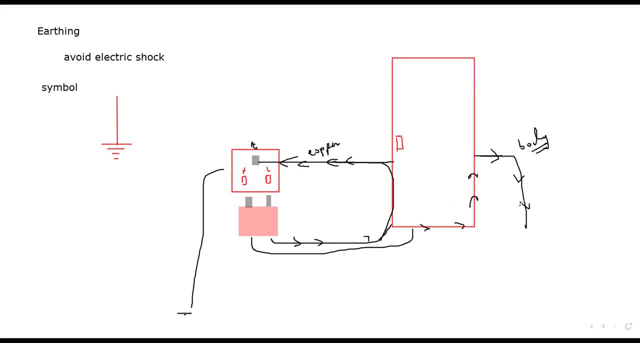 this is a refrigerator which is having a metal body so what happens if the live wire is in contact with a metal body so a person as a person touch he will get an electric shock so to avoid this there's another wire which is connected to the earth and we call this as the earthing wire and this earthing wire is connected to the metal body so when there is a current in the live wire which is the current in the live wire which is touching the metal body so that current will flow from metal body to the earthing wire so if a person is touching the metal body he will not get in Electric shock. Is it clear now? 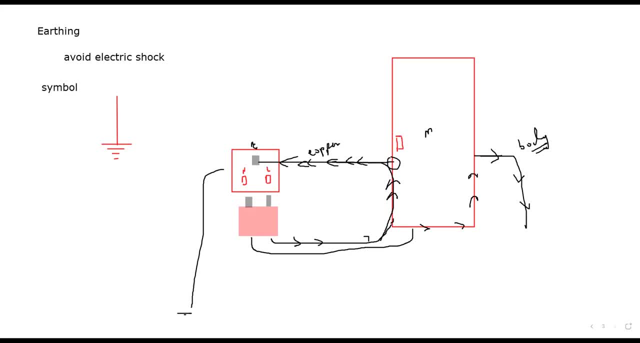 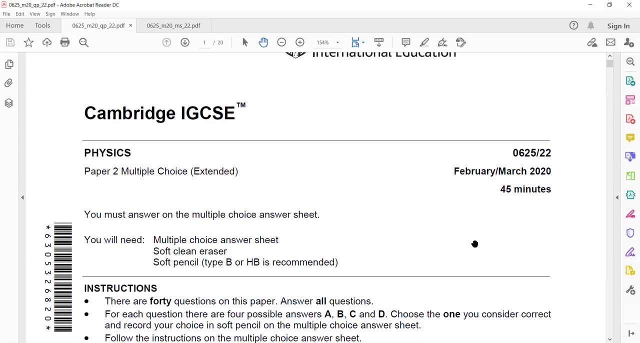 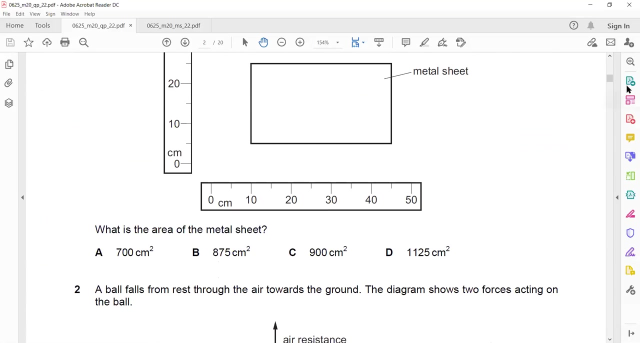 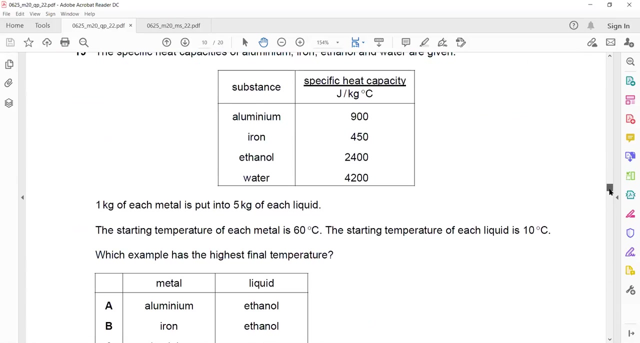 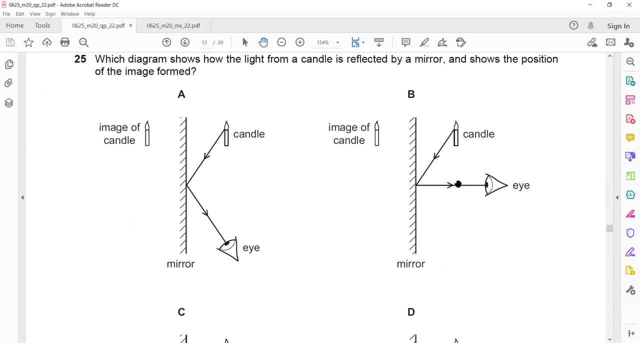 Now, some questions related to electricity. This is February, March 2020 paper. Electricity and magnetism mainly, I will discuss with you. Normally, from question 25 or 26 onwards, you will find electricity and magnetism. 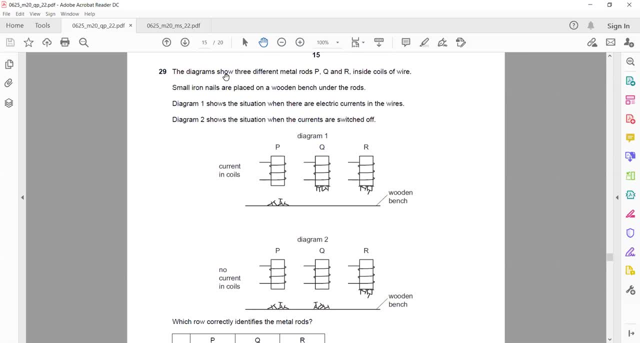 Okay, in this question, the diagram shows three different magnetisms. Metal rods P, Q and R and inside a coil of a wire. 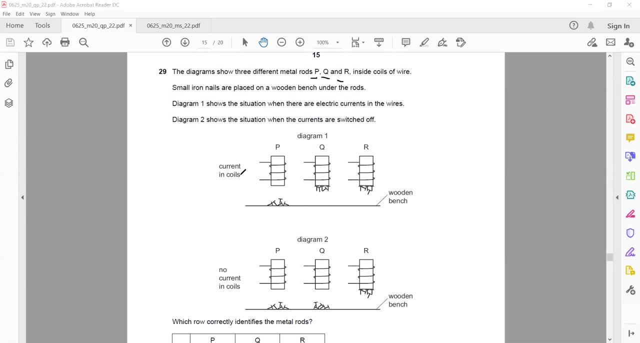 Small iron nails are placed on a wooden bench. You can see small iron nails are placed on the wooden bench. 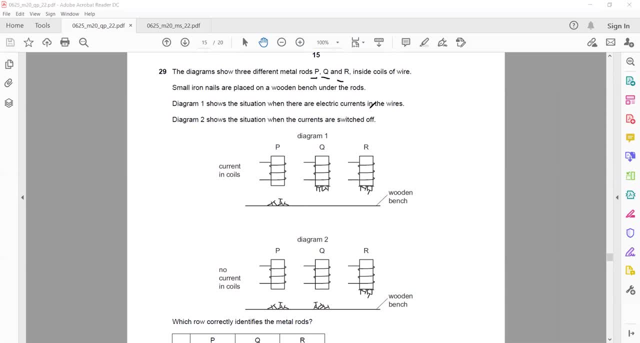 The diagram shows the situation when there is an electric current. So, it means when we are passing a current, that is diagram 1. 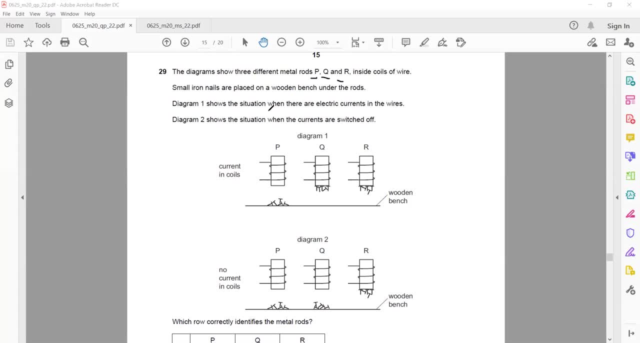 The diagram 2 shows the situation when the current is switched off. So, when the current is switched off, still the nails remain in contact with R. 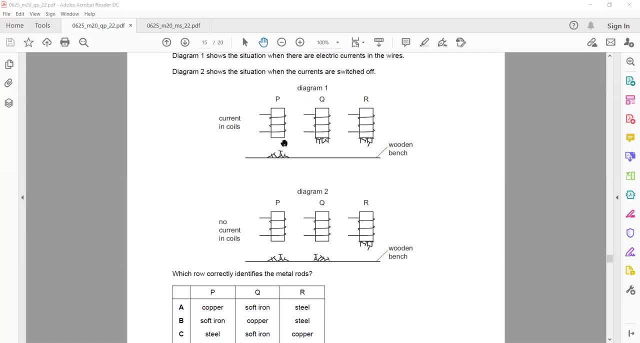 Which row correctly identify the metal rods? What is the right answer here? Which row correctly identify the metal rods? 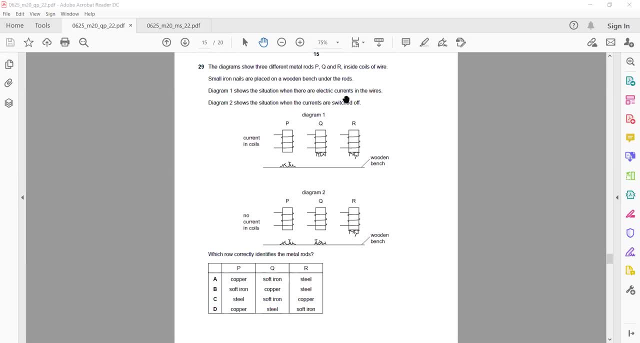 Look, for first one, when you are passing a current, and if you are not passing a current, this material does not behave like a magnet. 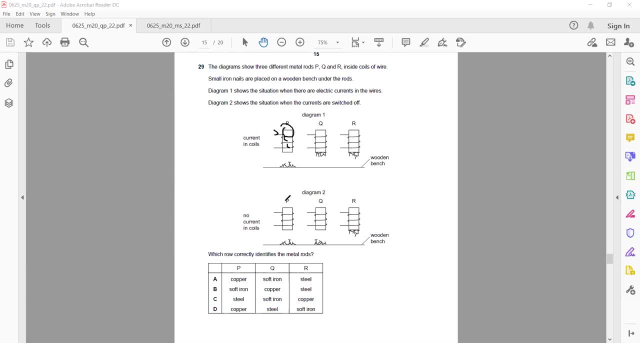 So, if the material does not behave like a magnet, it means the P should be a non-magnetic material. 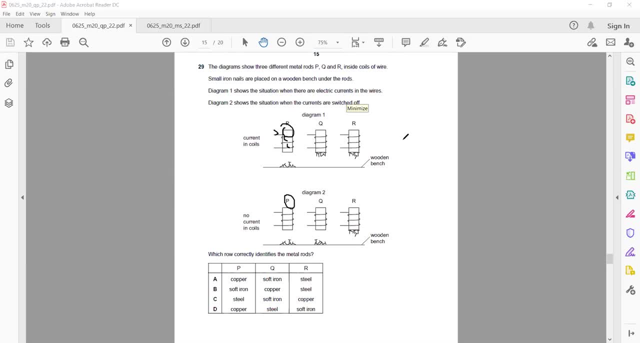 Steel is a permanent magnet. Iron is a temporary magnet. 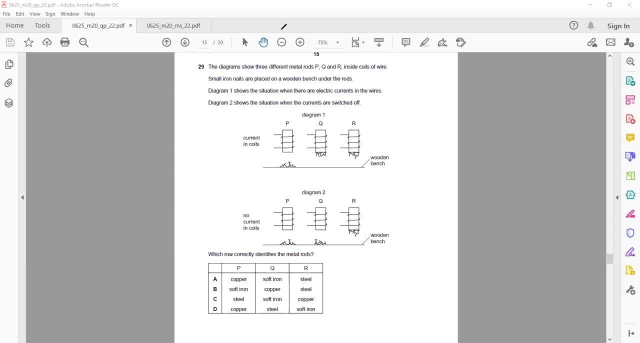 So, when you check the first one, I want participation from everyone. 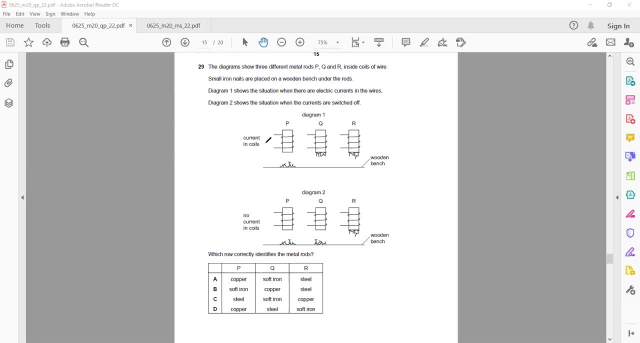 So, for first one, when you are passing the current, if you are not passing a current, it means the material, like when you are passing a current, there is a current, 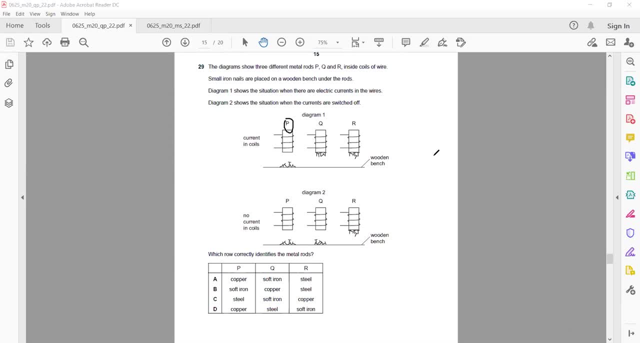 If this material does not behave like a magnet, it means it is a non-magnetic material. 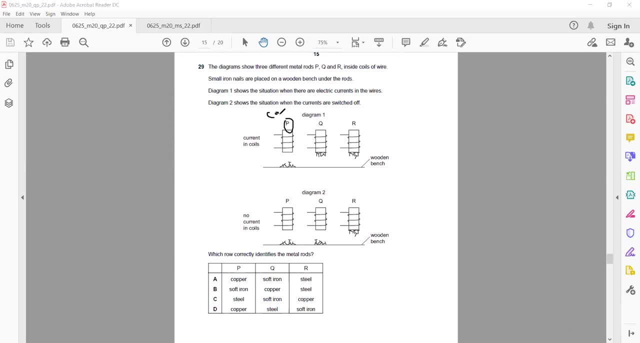 So, it means, this should be copper. Because copper is a non-magnetic material. 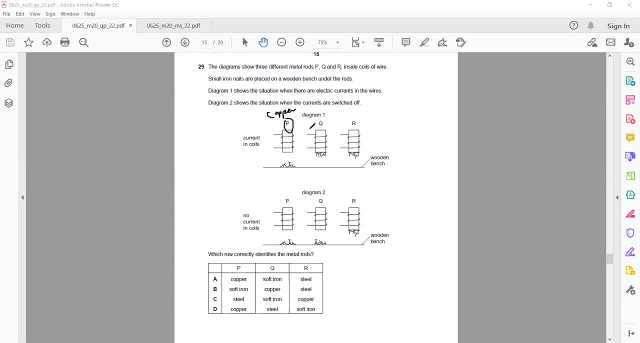 Iron, steel, nickel, cobalt, these are the magnetic material. 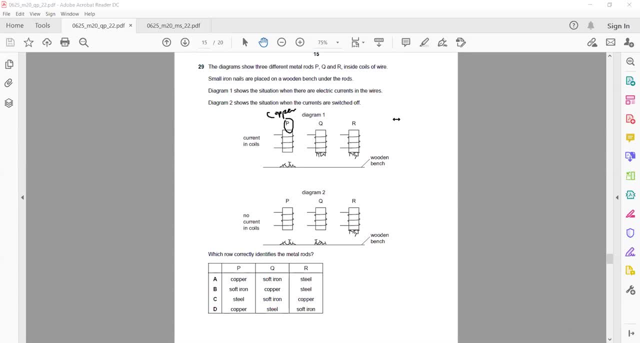 When you pass, the current is having a magnetic effect, but that current is not able to magnetize this material. That's why the material is not attracting the iron nails. 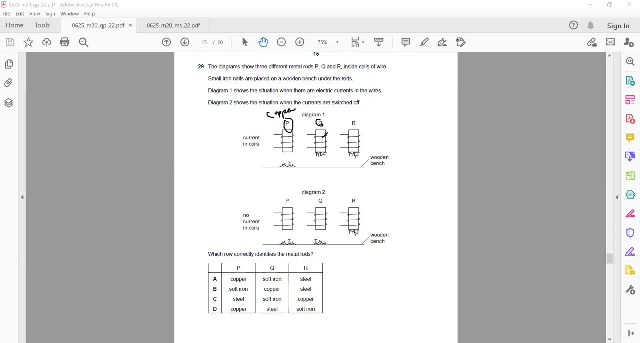 But for Q, when you are passing a current, it is behaving like a magnet. That's why it attracts the iron nails. For R, when you are passing a current, it is behaving like a magnet. That's why it is not attracting the iron nails. That's why it is attracting the iron nails. So, Q and R are the magnetic material. Then, what about the nature of the magnetic material? As you switch off, this material is demagnetized. So, which material is a temporary magnet? Iron or soft iron? 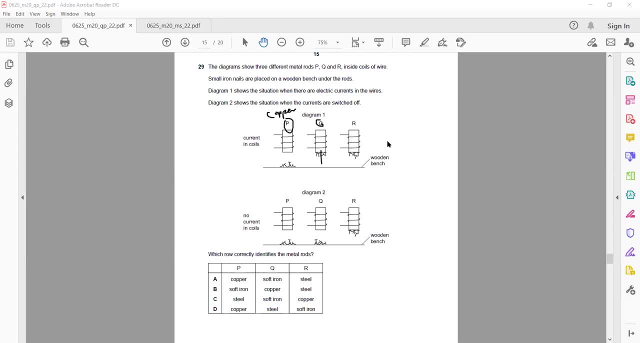 We can say, it's a temporary magnet, where steel is a permanent magnet. 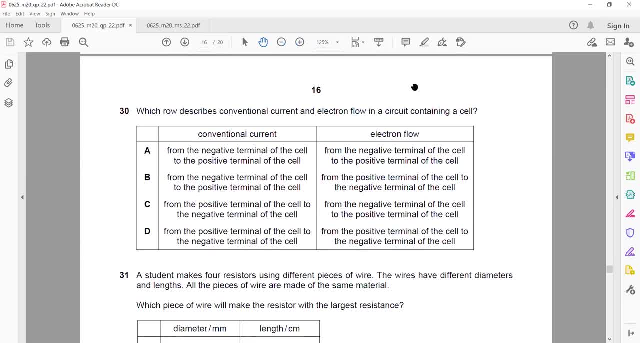 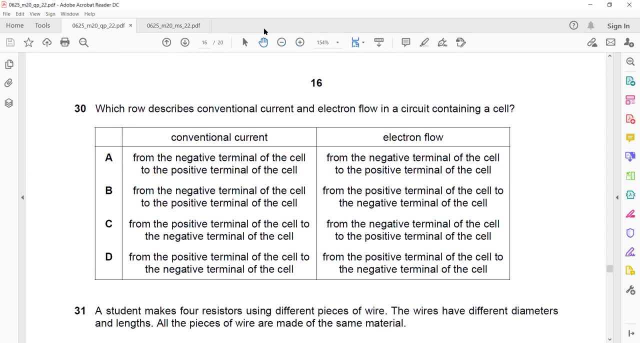 Which row describes the conventional current and the electron flow? Which row describes the conventional current and the electron flow? Yeah, that's right. C is the correct answer. The conventional current, because the conventional current assumption is that it's from positive to negative. 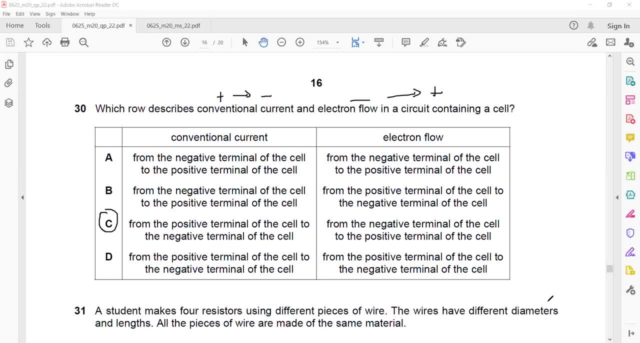 In reality, electrons are moving from negative to positive. But in exam, if they say show the direction of the current, they always mean the conventional current. 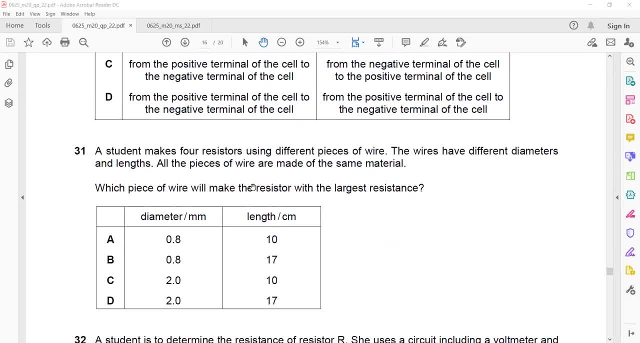 Until unless they ask in the question that mention which one is, like mention the electron flow. 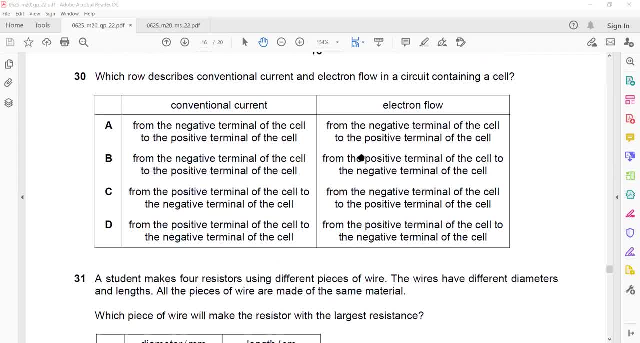 Sir, in electrolysis, the electrons move from positive to negative. In electrolysis? No, no. 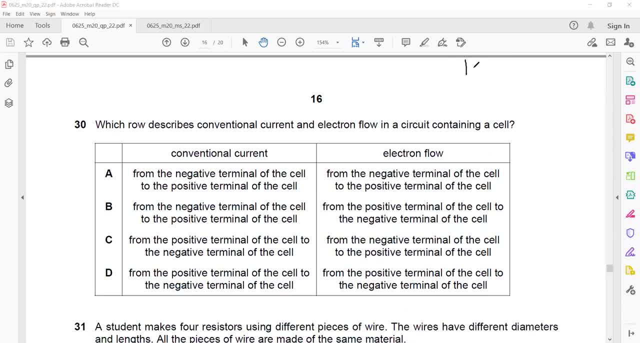 In electrolysis as well, basically, in electrolysis, like example, you have a positive and the negative terminal and you connect two electrodes. 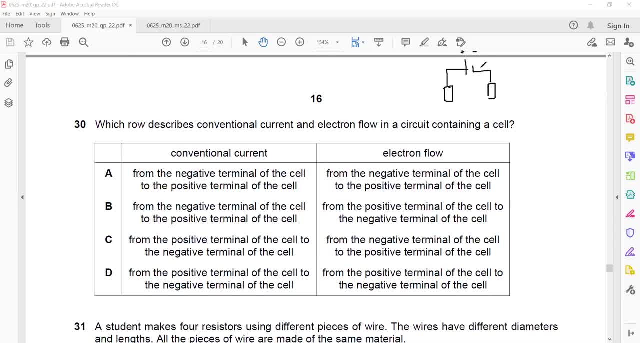 So, then from the negative terminal, electrons are coming out and towards the positive terminal, electrons are moving. 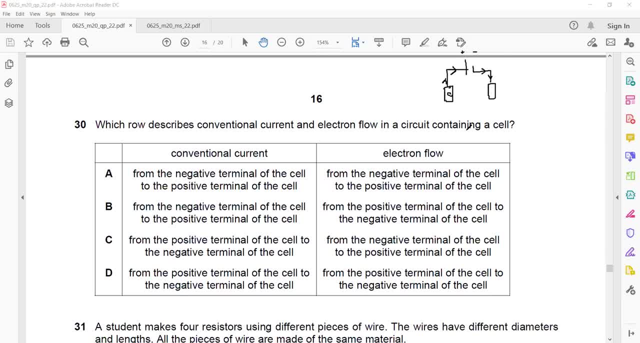 Electrons are attracted towards the positive and going out from negative. So, it's the same thing. 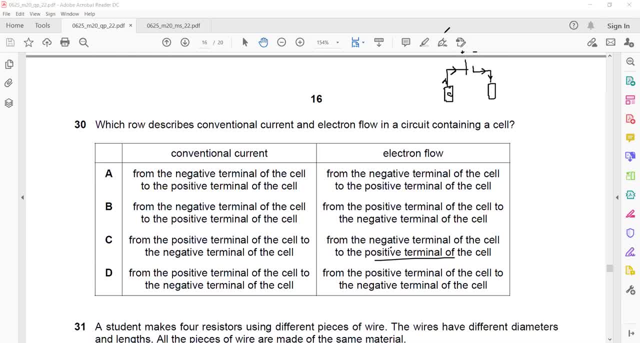 From negative terminal, it's out and towards the positive terminal, it's in. It does not change. 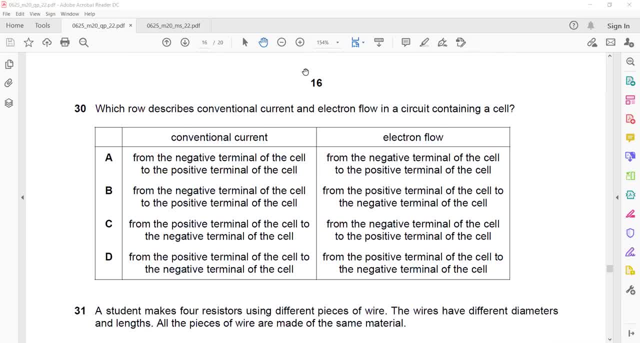 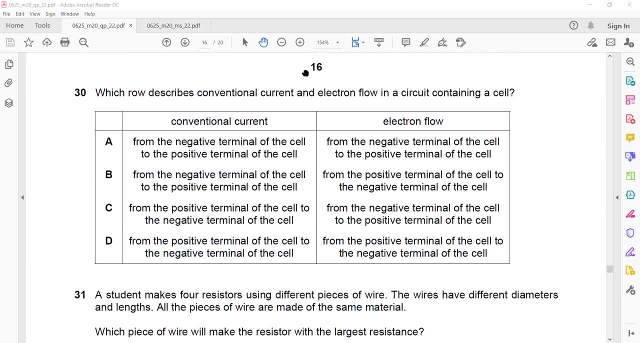 Why still we are using? Look, the reason is that why conventional current is used till now, not the electron flow, even though conventional current is nothing, but because most of these laws in electricity are derived on assumption that the current is a movement from positive 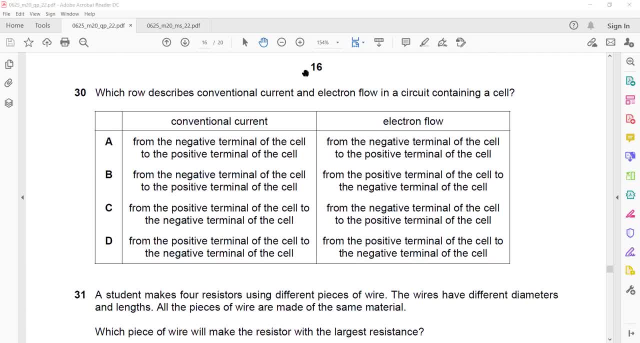 to negative. That is why they did not change the sign convention of the law. So, still following those laws because the statement of the law is correct. The only difference is the direction. So, all of these laws of electricity are derived for positive to negative. 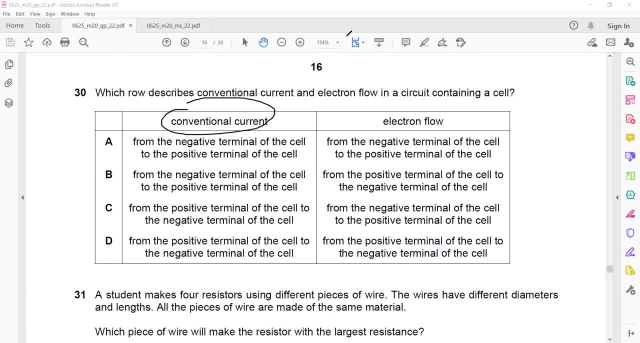 That's why still we are using this conventional current. 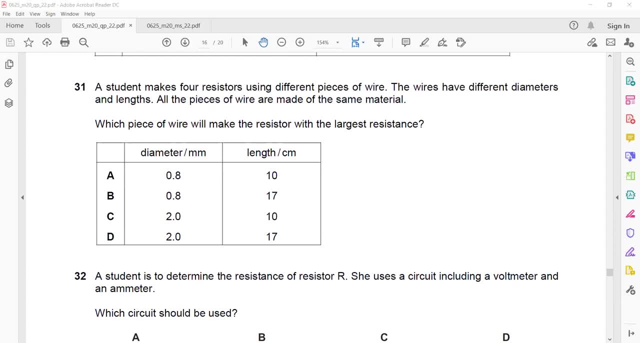 The student makes four resistors using a different piece of wire. The wires have different diameters and length. 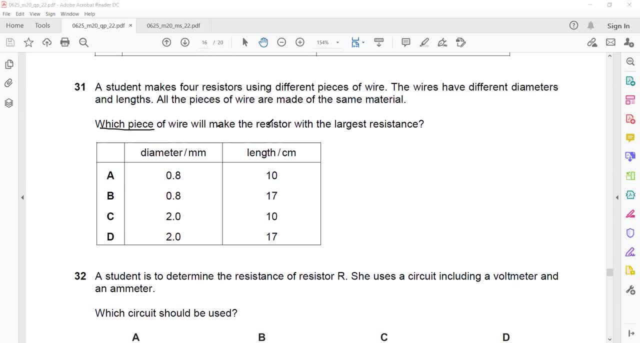 All pieces of wire are made up of same material. Which piece will make the resistance largest? 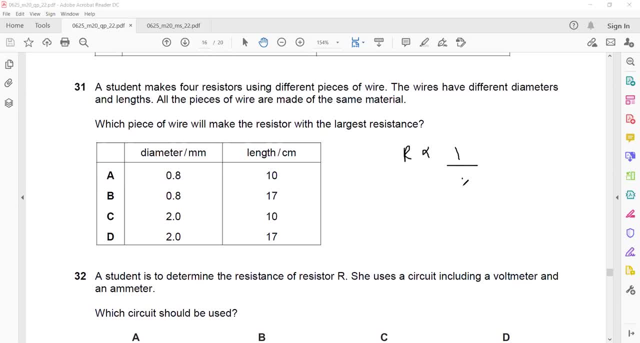 Keep in mind, resistance is inversely proportional to area or diameter square 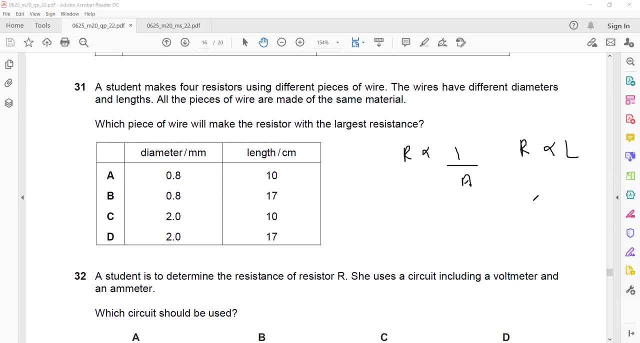 and resistance is directly proportional to length. So, if you increase the diameter, it means you will increase the area. 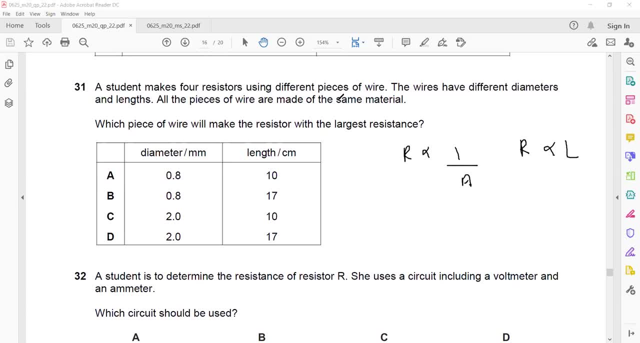 If you decrease the diameter, you will decrease the. So, longer wires have more resistance and thinner wires have more resistance. 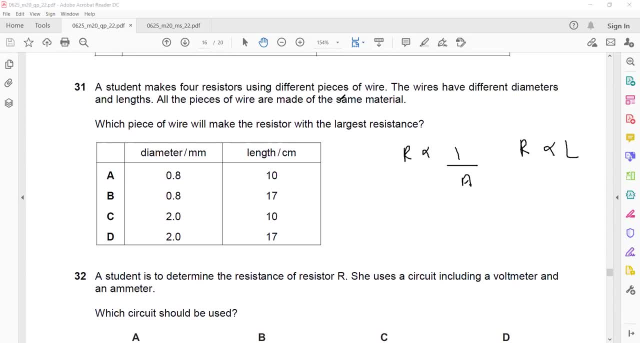 So, which combination will give the largest resistance? So, this one is the largest. This one is the biggest. This one is the largest. 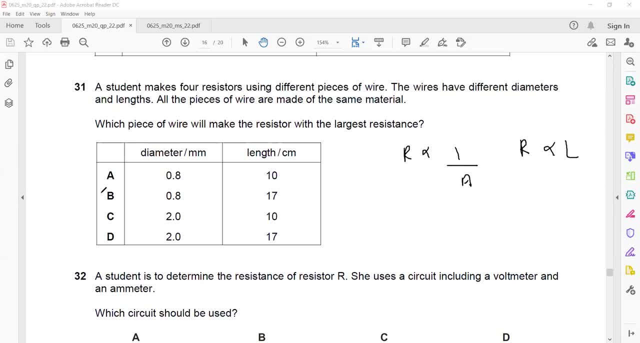 so b is the right answer because when you decrease the diameter means you decrease the area so resistance increases if you use a longer wire the resistance will also increase 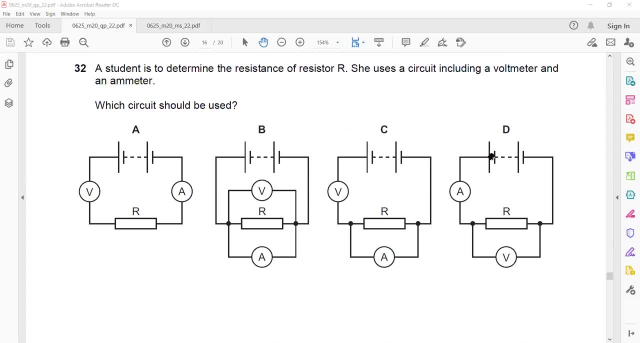 a student is to determine the resistance r she uses a circuit include a volt meter and m meter 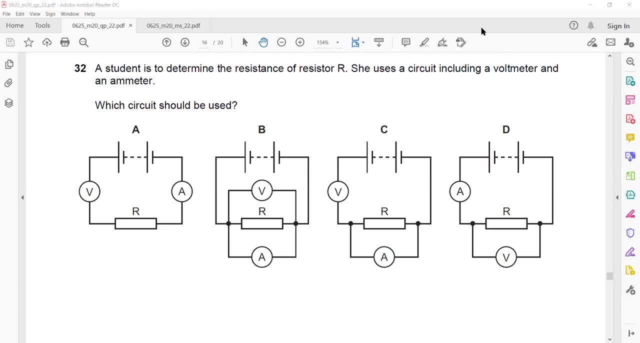 which circuit should be used volt meter are always connected in parallel because in parallel the voltage is same and m meters are always connected in series because in series the current is same so which circuit should be used to get the resistance basically by voltage 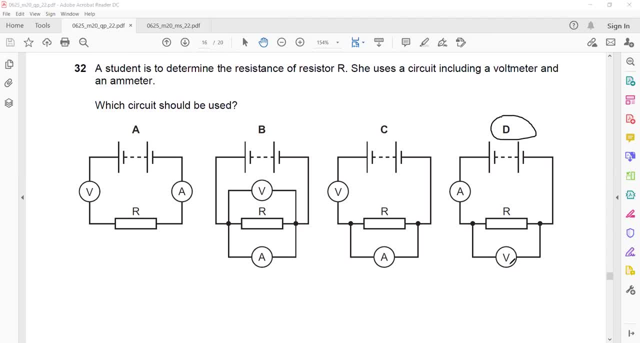 so d is the right answer you can see volt meter is in parallel to a component which we want to resistance and m meter is in series so practically you 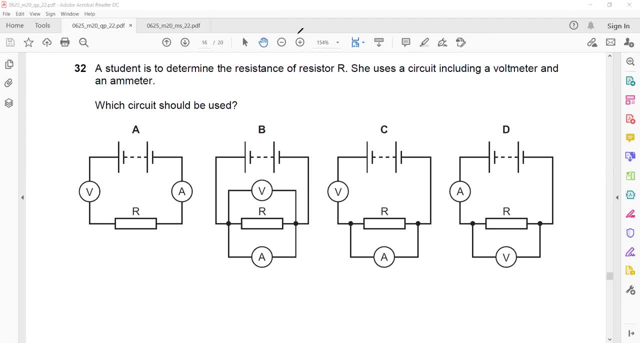 If we have any kind of circuit, like example, if I say, so if I say I have three resistors connected in series, so I have three resistors connected in series and I want to find the 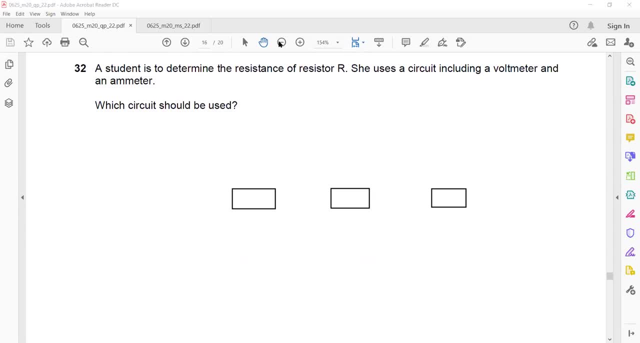 resistance of this circuit. So to get the resistance of the circuit, I need the total voltage and I need the total current. So to get the current, I will connect an ammeter and to get the voltage, I will connect a voltmeter in parallel to this series combination. That 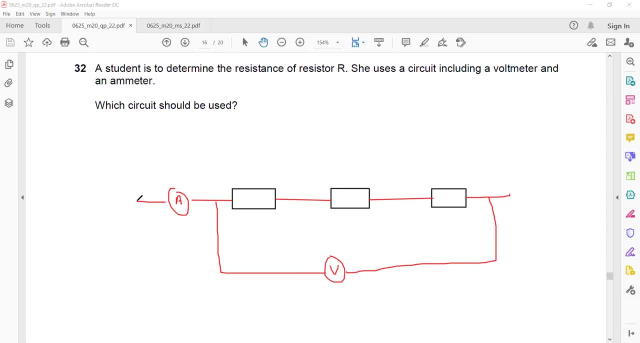 will give me the total voltage of this combination and voltage divided by k. 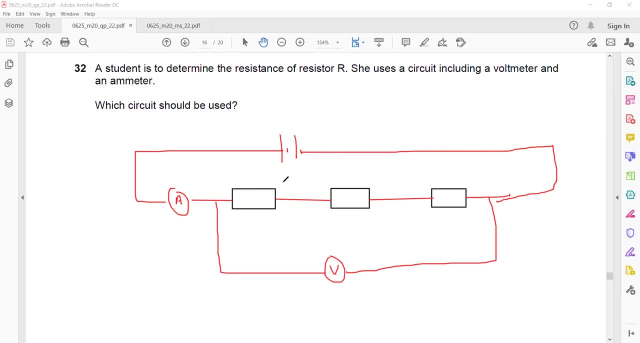 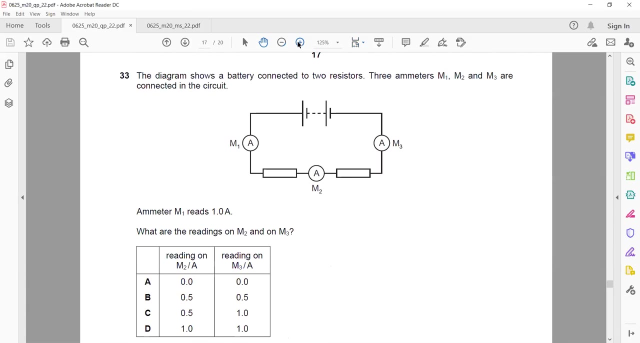 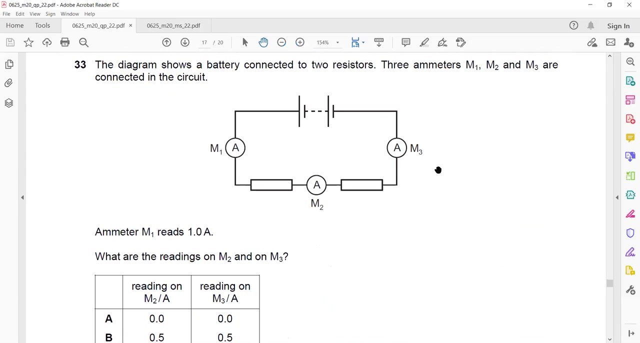 So to get the current, what we will get? We will get the resistance. So this is a practical way of finding the resistance of the circuit, is the voltage divided by current. The diagram shows a battery connected to two resistors. The three ammeters, M1, M2 and M3 are connected 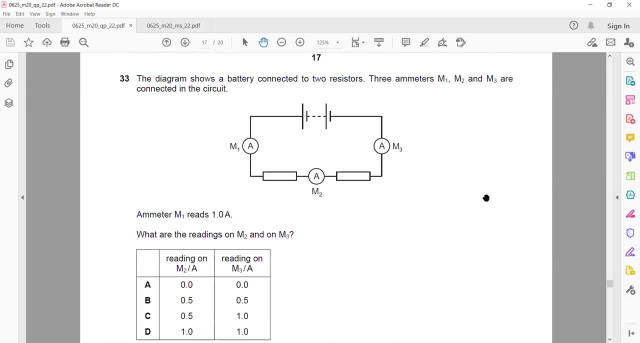 in the circuit. Ammeter M1 reads. 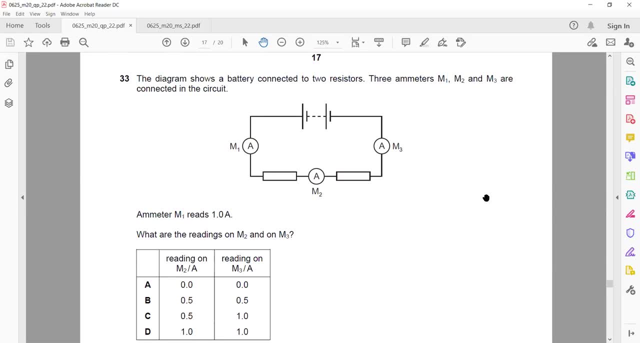 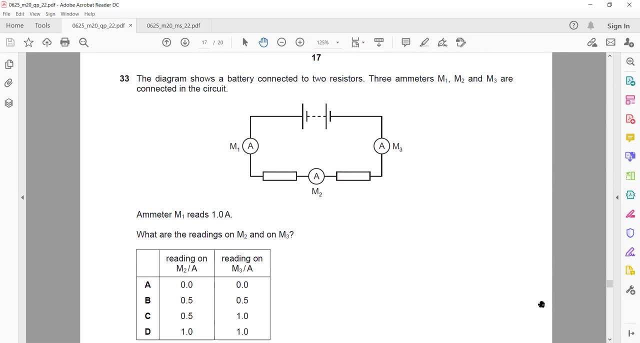 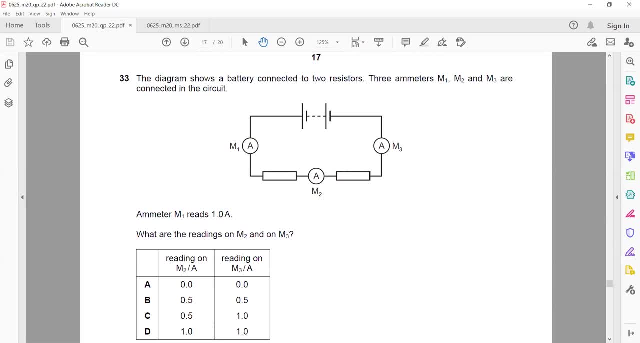 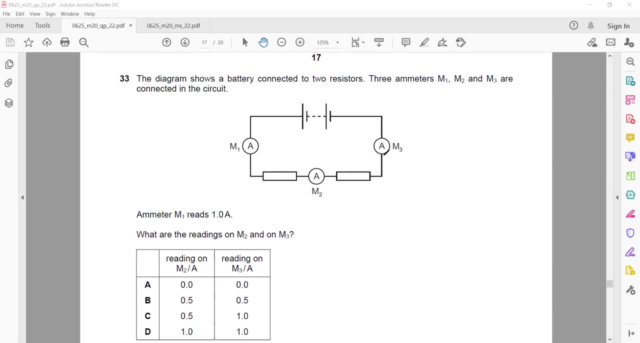 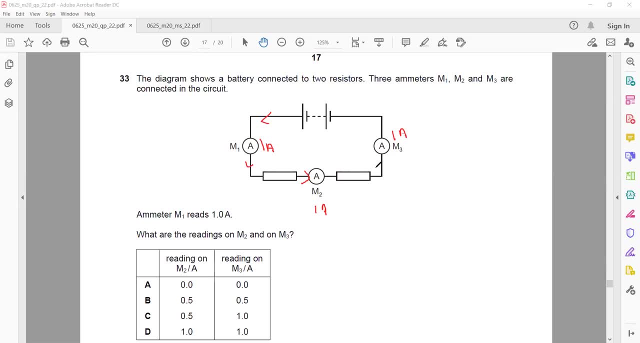 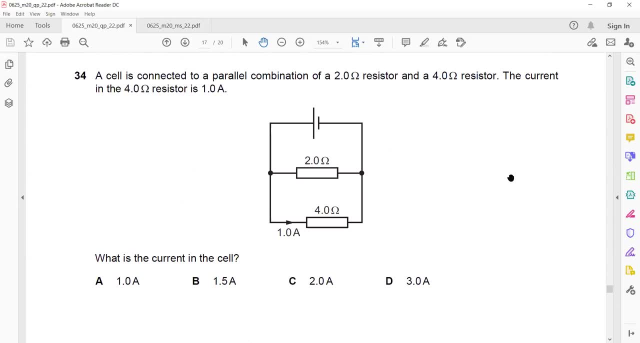 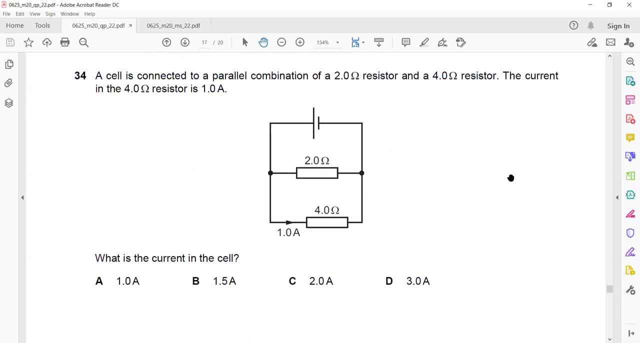 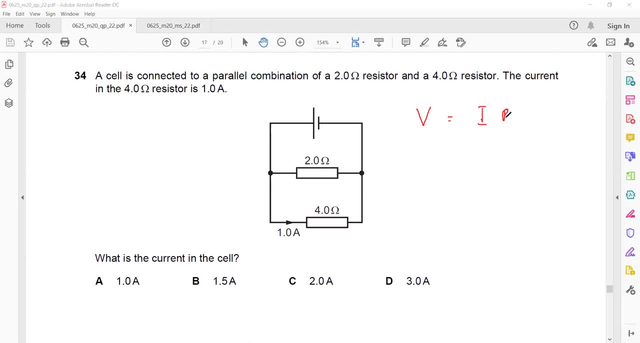 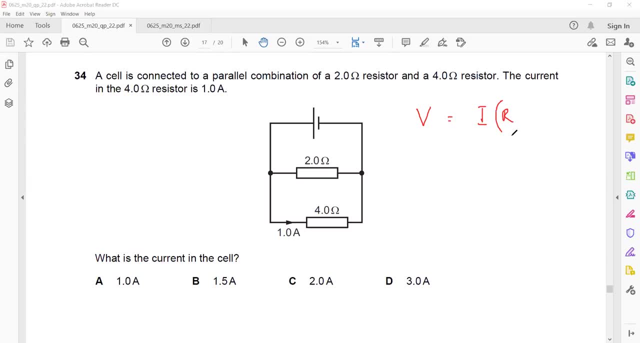 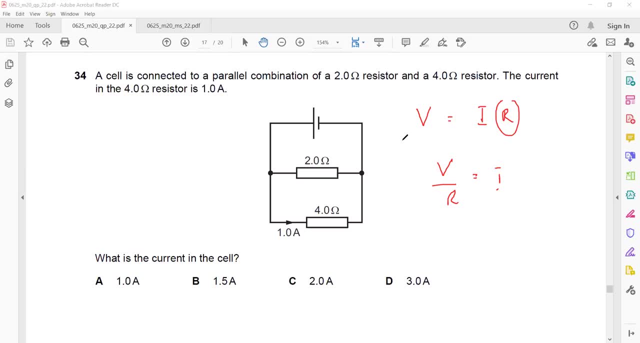 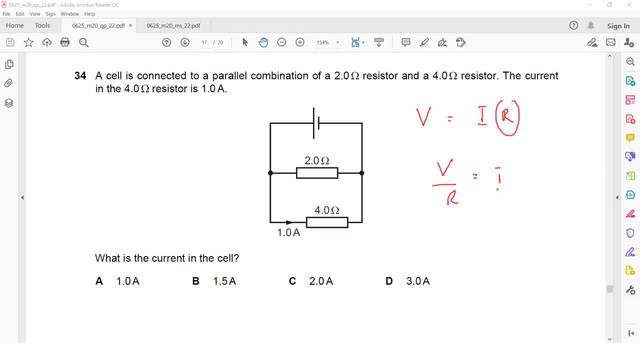 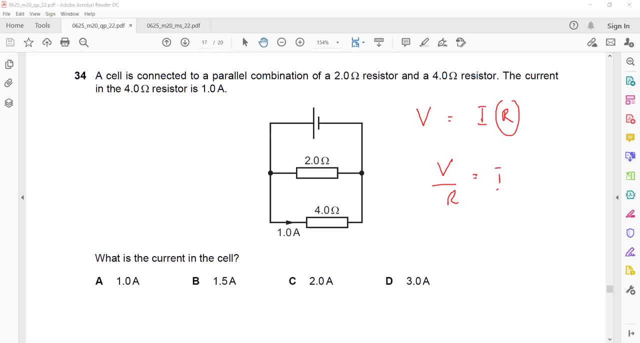 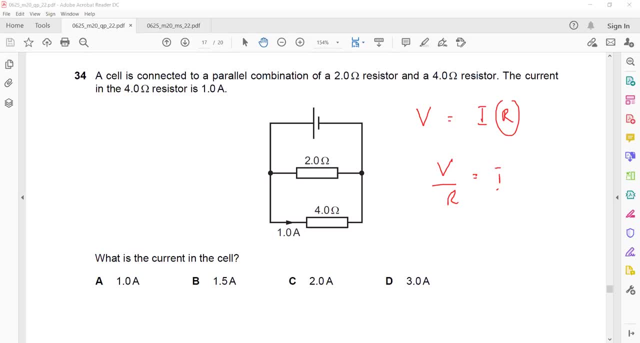 Ammeter M1 reads. you can also do another thing because they are in parallel so what we will do first we'll find the voltage here how to get the voltage here so v is equals to ir i is the current and r is the resistance of 1 multiplied by 4 that's equal to 4 volt so this resistor is having 4 volt because they are in parallel so this will also have 4 volts so both of them will have 4 volts now what about the current in this resistor so how i can find the current current is equals to volt v is equals to ir so current is voltage divided by resistance voltage is 4 and the resistance is 2 4 divided by 2 that's equal to 2 ampere so 2 ampere is passing through the 2 ohm resistor and 1 ampere is passing through 4 ohm resistor so what is the total current enter from the cell the total current in the cell if in one branch it is 2 ampere the other branch it is 1 ampere so what is the total current so 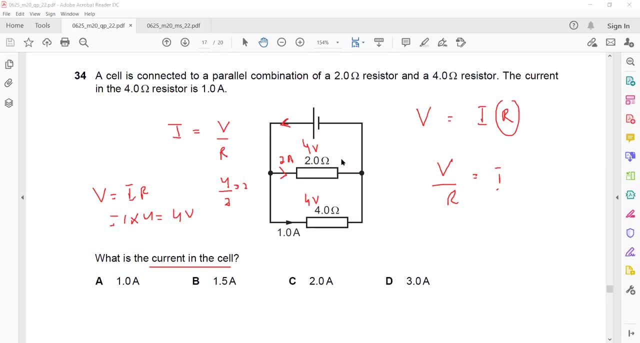 of your molecule 3 right so to the total current this is headquarters 3 ampere because the 3 ampere is passing. That's why D is a right answer. 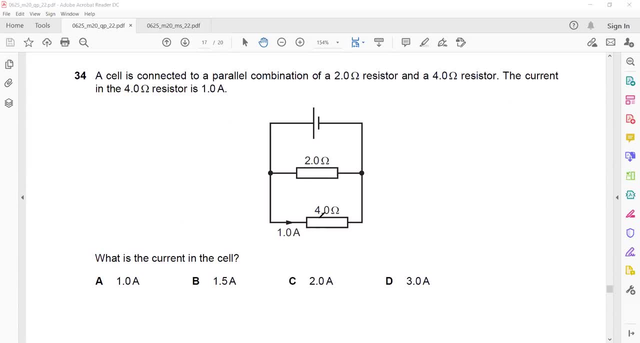 There's also another way to get this answer like after getting the voltage here is 4 volts so we identify the voltage of this one is also 4 and the voltage of the battery is also 4 because all are in parallel. 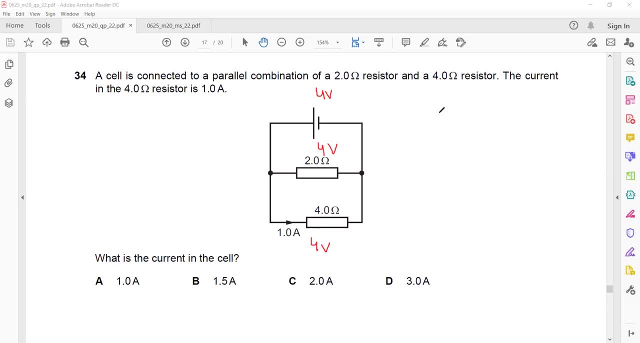 Now what about the total circuit resistance? So what is the total circuit resistance? 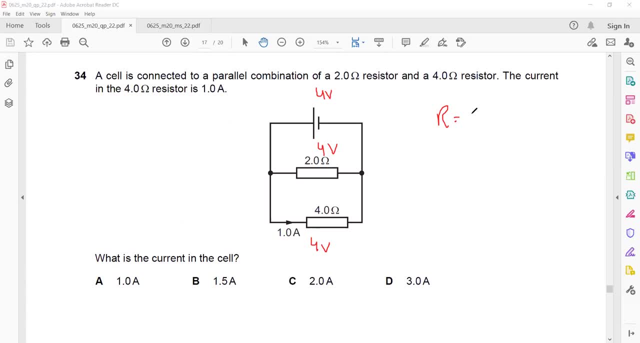 It is product because they are in parallel. So if they are in parallel it's product divided by sum. So 4 multiplied by 2 divided by 4 plus 2. So 4 multiplied by 2 is 8. 4 plus 2 that's equal to 6. 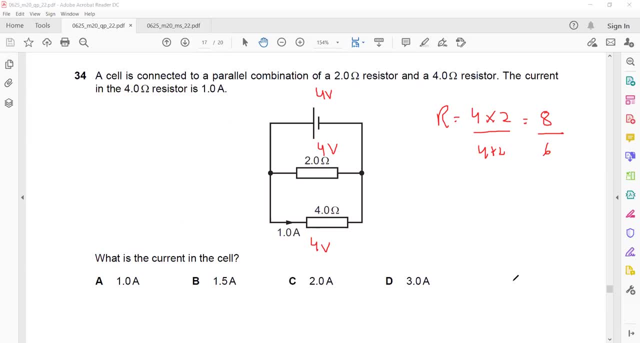 So that will be equal to 8 divided by 6. 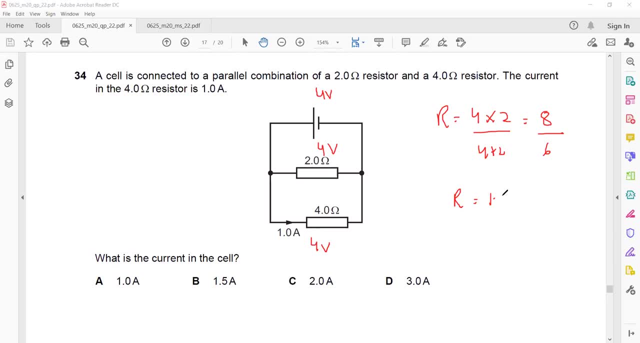 1.33 So 1.33 ohm is the total resistance of the circuit. You have 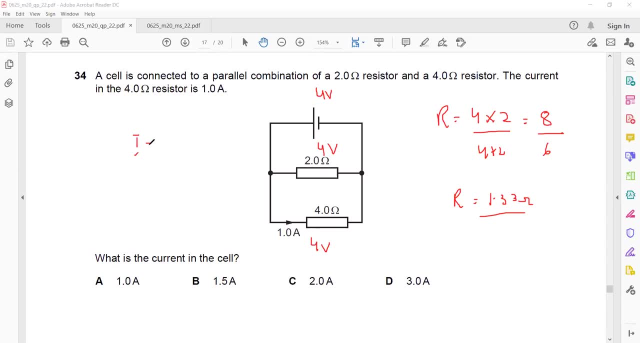 the voltage so you can find the current. Current is voltage divided by resistance 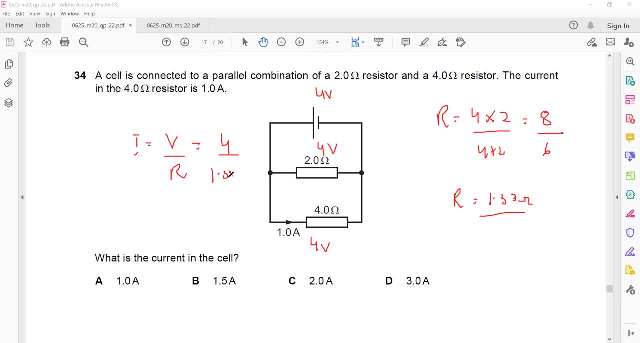 so it will be 4 divided by 1.33 when you divide you will approximately get 3 ampere. So this is the second way of getting the answer. 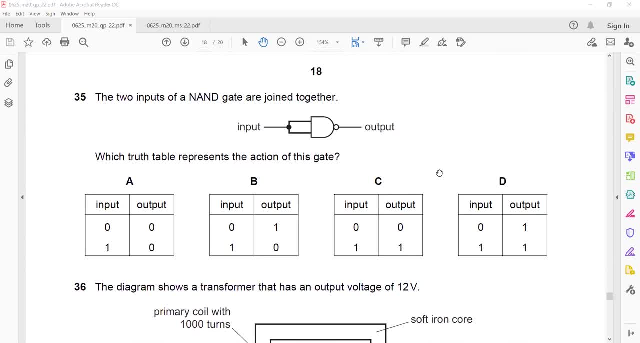 Question 35 Two inputs of NAND gate are joined together. 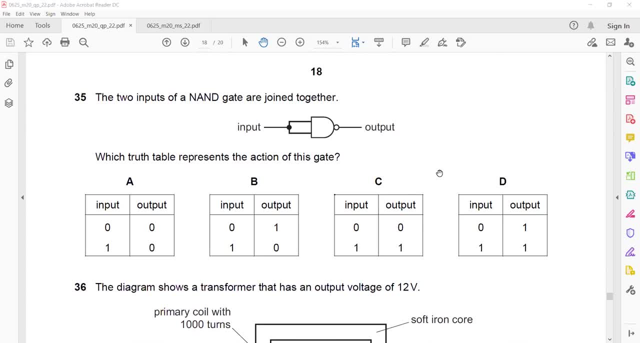 Which truth table represent the action of this gate? NAND gate means the output of NAND is inverted. 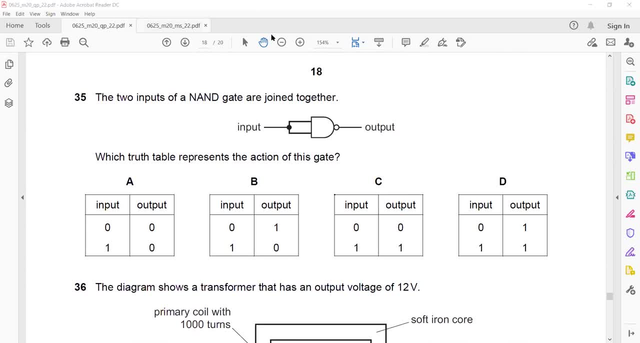 So if we join, basically if we join the two input it means, like example if this is 0, this will be 0 and this is also 0. So 0 0 for NAND gate it is 0. When it passes through inverter it will make 1. So if input is 0 the output will be 1. 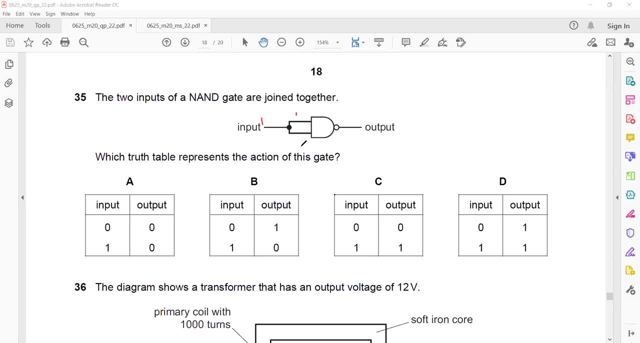 And opposite if input is 1. So this is 1 and 1. 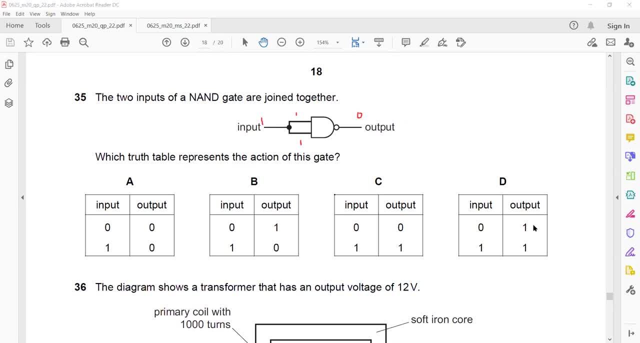 1 1 is 1 but passes through inverter it will make it 0. So basically it will behave like a NOT gate. So when 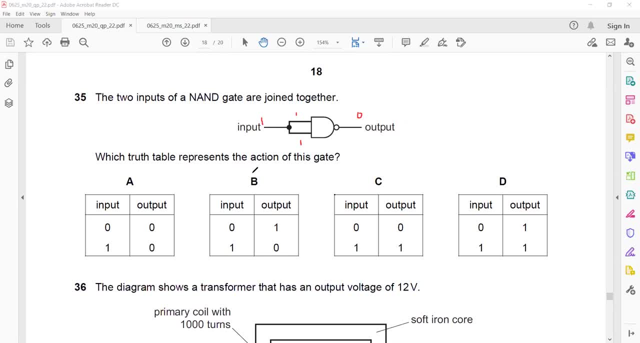 NAND gate both inputs are joined together it is acting like a NOT gate. When input is 0 the output is 1. When input is 1 the output is 0. 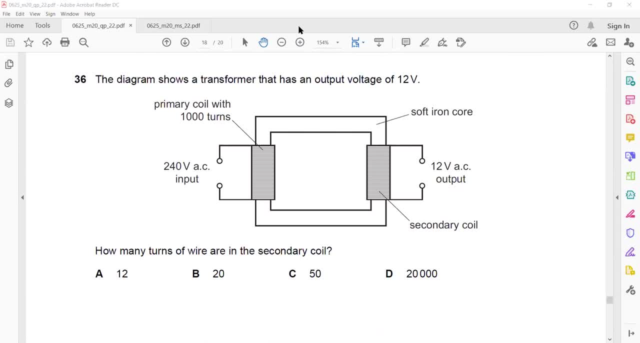 The diagram shows a transformer that has an output voltage of 12 volts. So this output voltage of 12 volts the input is 240. 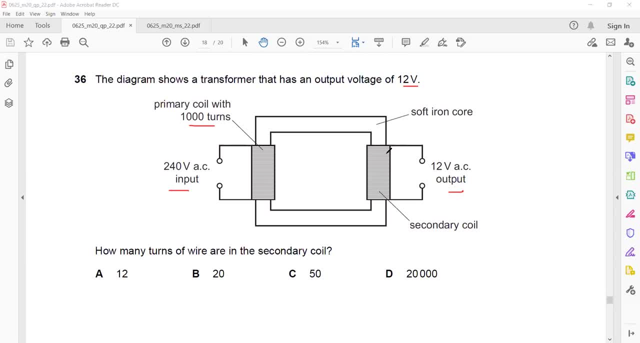 Primary is having 1000. We need a number of turns of secondary. So use the formula Vs over Vs. 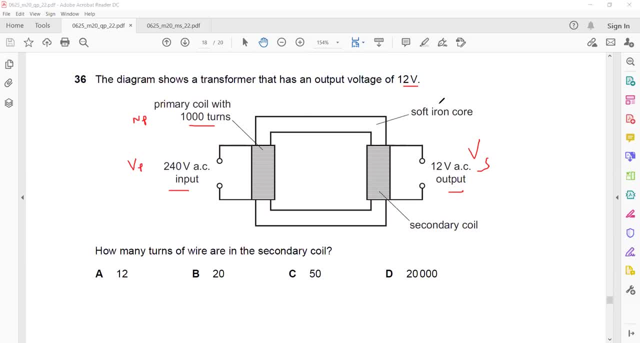 Vp is equals to Ns over Np. 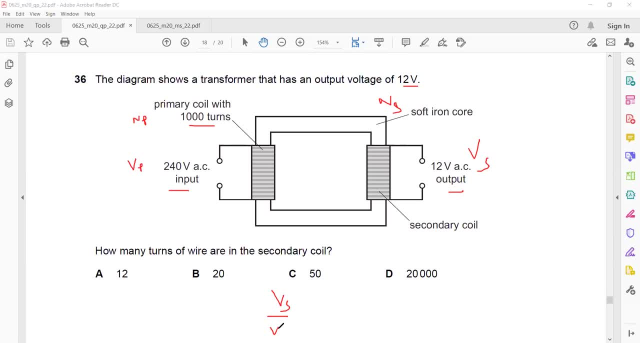 So what's the answer? Correct answer after substituting the values. 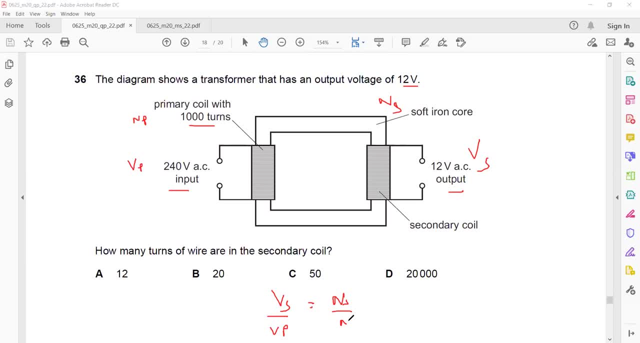 Vs over Vp is equals to Ns over Np. 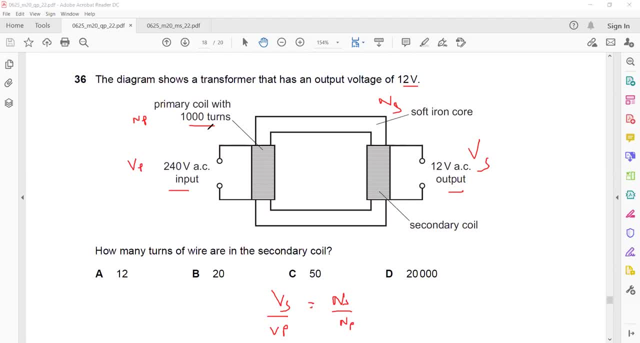 And first thing you can identify it's look it's a step down transformer because input is having 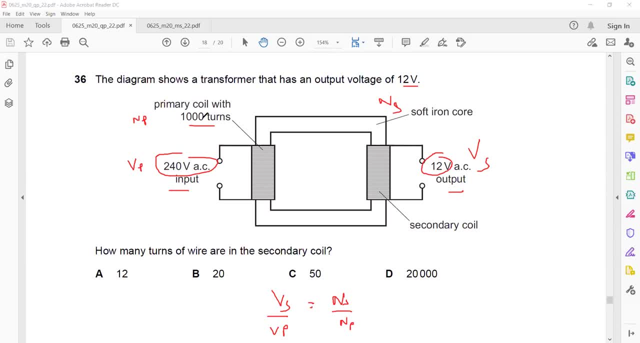 240 and output is only 12. So the number of turns of secondary should be less than number of turns of primary. So if primary is having 1000 so 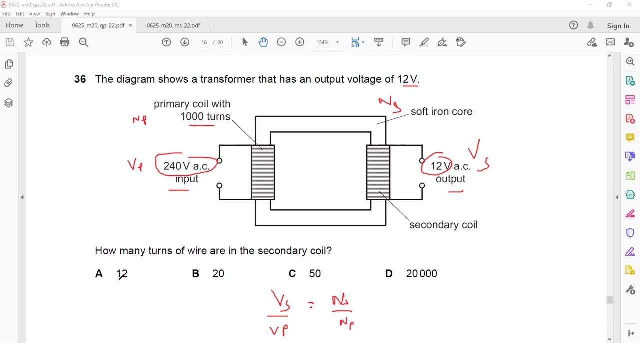 secondary should have less than 1000. So either A can be answered B or C. It cannot be D because D is 20000. So that's totally wrong. 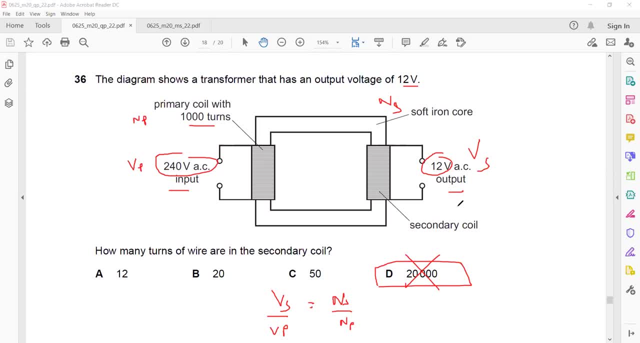 So when you substitute so three answers are there like 12, 20, and 50. Now which one is correct? You have to check by substituting the value Vs over Vp is equals to Ns over Np. 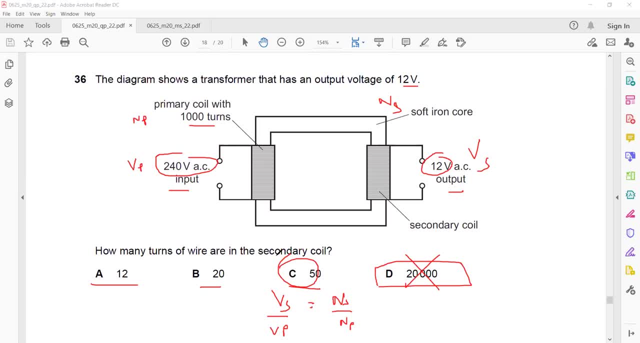 So when you substitute the value you will find that C is the right answer. 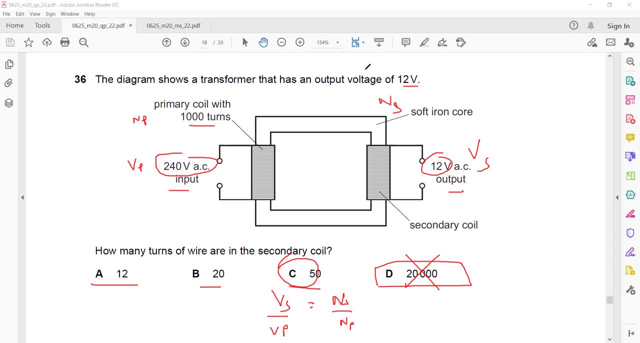 Three of them are possibility that it can be right. But one of them is a correct answer. D is totally wrong according to the working answer. So let's look at the equation of this transformer. 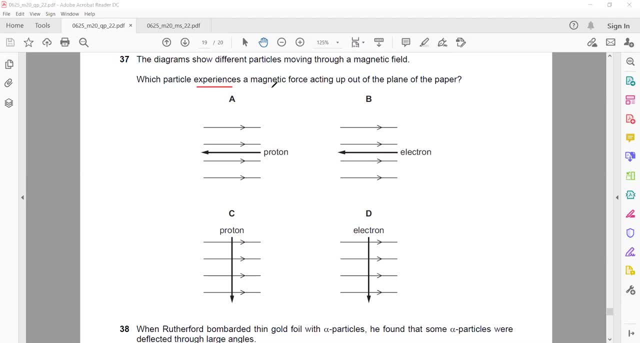 The diagram shows different particles moving through a magnetic field. 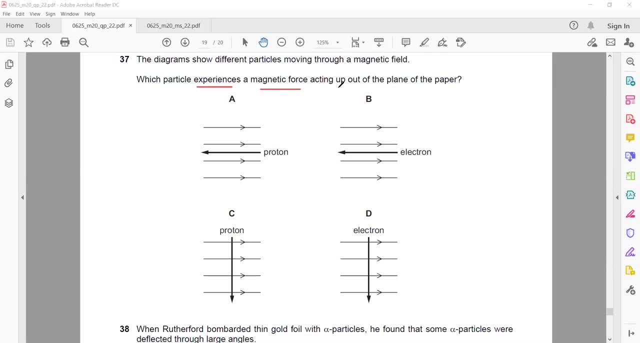 Which particle experience a magnetic force acting 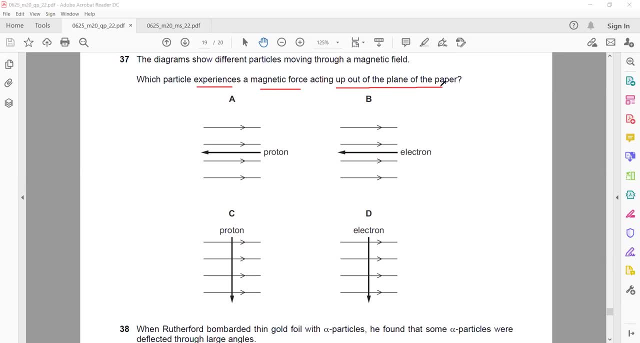 out of the plane of the paper. So what you have to do for positive particle, for positive particle, use left hand. If you want to find the force on the positive particle in a magnetic field, use left hand. And for negative particle, you will use right hand. 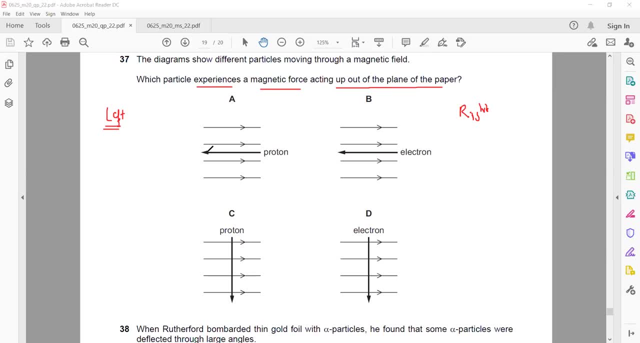 But the thing is, when the particles are moving parallel to the magnetic field, they will not experience force. 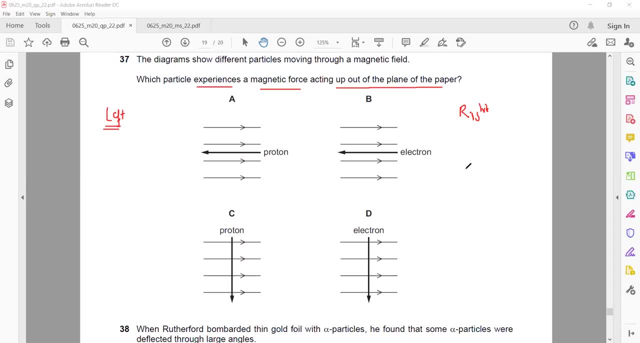 They should move perpendicular or 90 degree. Parallel or anti-parallel, 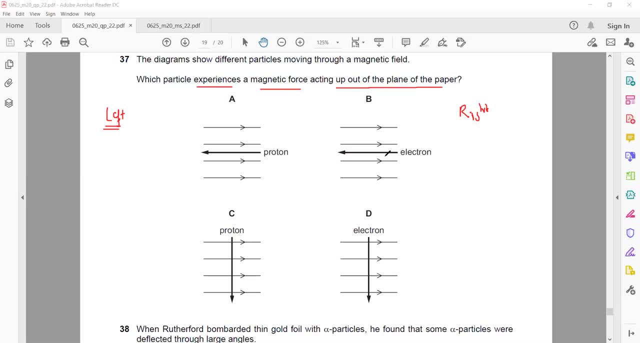 it will not experience. Like example, if this is a magnetic field, and the particle is moving parallel to the magnetic field, and the particle is moving parallel or anti-parallel, like this is parallel to the magnetic field, this is anti-parallel. In both cases, the particle will not experience 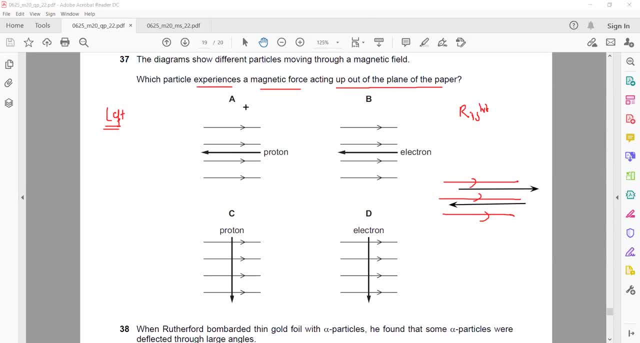 any force because it should cut the magnetic field. So how it can cut the magnetic field? By moving perpendicular to the magnetic field. 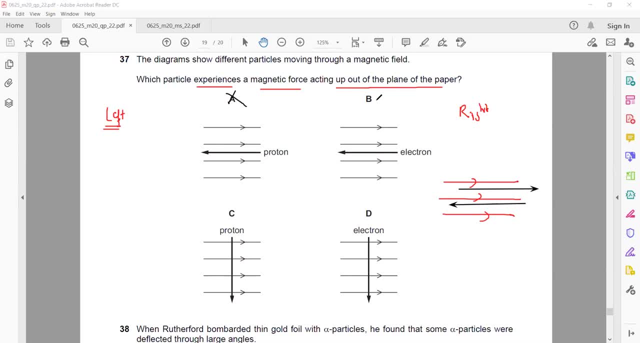 So first, A and B cannot be an answer. A and B are totally wrong. Like it does not support that experiencing a force. So you are left with, yeah, the Fleming rule you have to use. 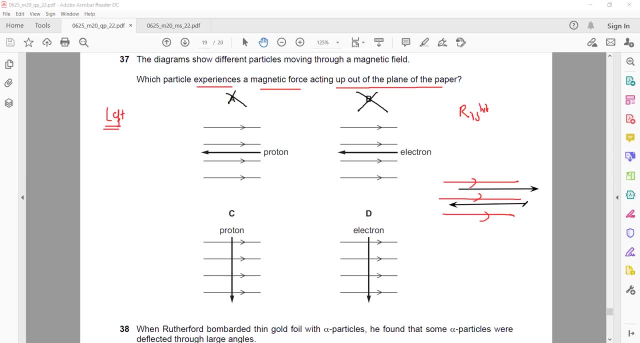 If you are finding the force on the positive particle, you will use left hand. 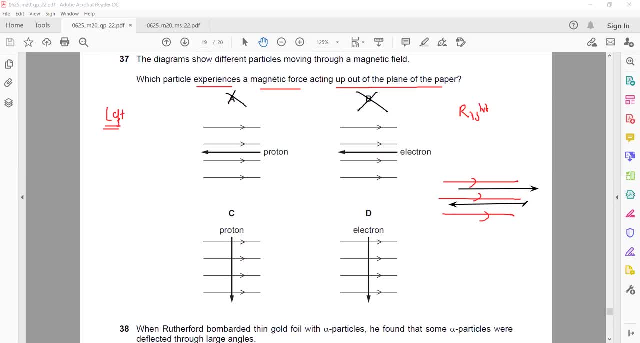 If you are finding force on the negative particle, you will use right hand. 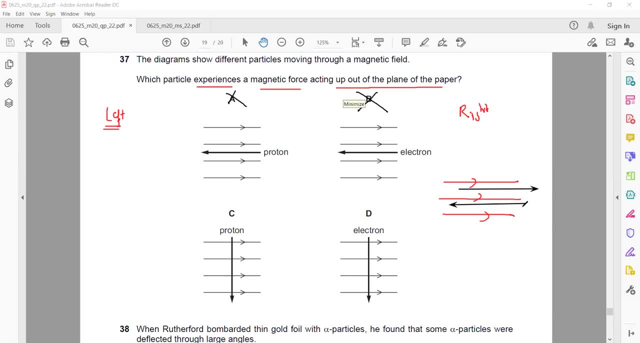 This part, actually, this force on the particle in a magnetic field is also, you will study in last topic which is atomic physics. 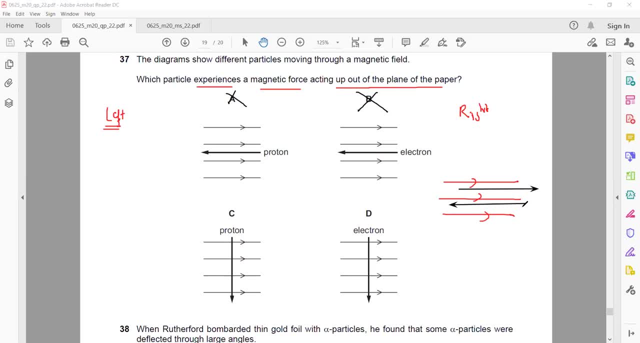 So this question is from atomic physics. But already you took, already you studied that the Fleming left hand rule. So you can work out. 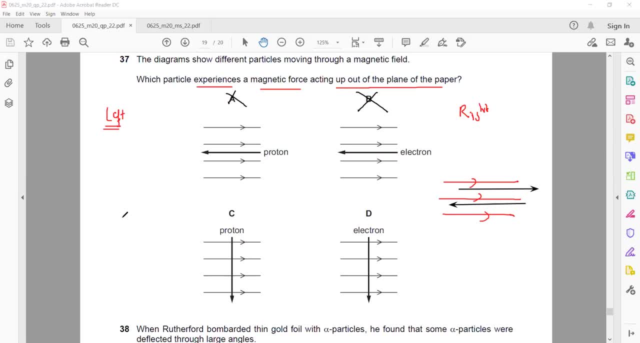 So according to Fleming left hand rule, your first finger should point towards the magnetic field. 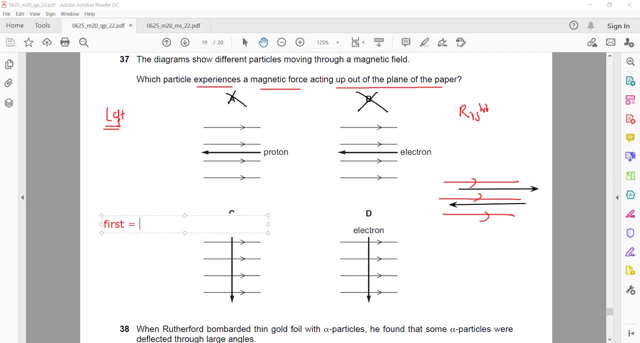 So in this case, when you apply the rule, your first finger should point towards right hand side. 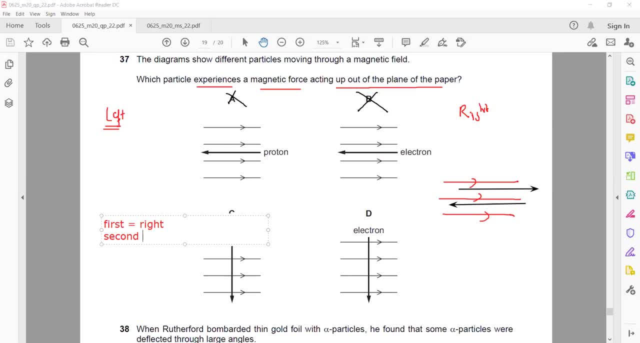 Your second finger should show the direction of the particle, in which direction the particle is moving. So your second finger should point down. 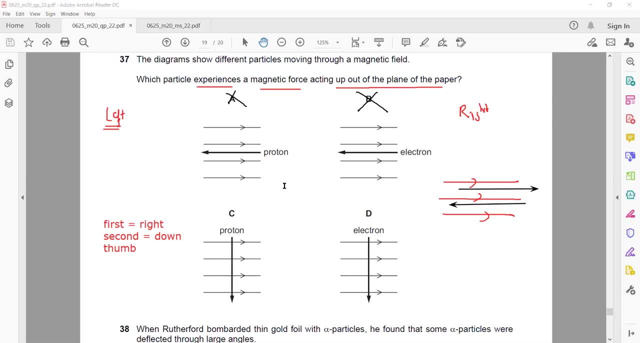 So where your thumb is pointing when you apply the rule. So first finger represent towards right. 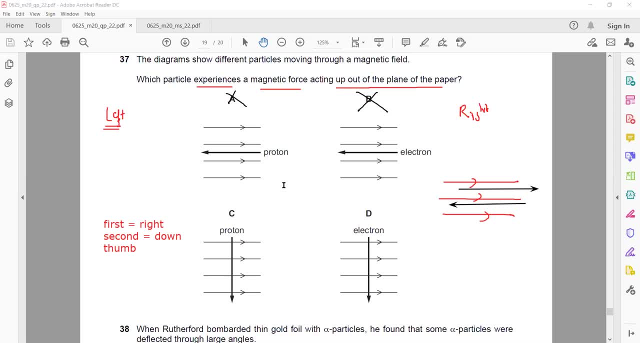 Second represent direction of the particle which is down. And thumb is pointing, which direction your thumb is pointing. 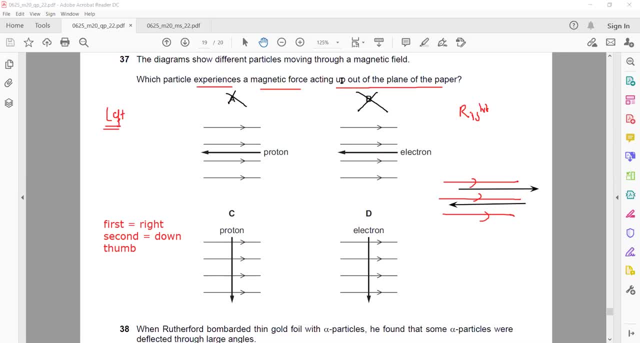 So thumb is pointing outward. Yet towards yourself. So if thumb is pointing towards you, 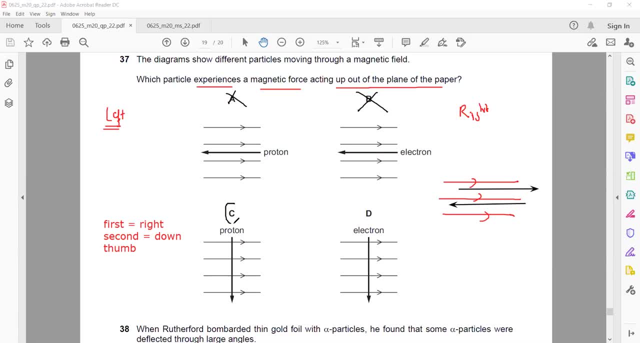 what it shows? It shows that it is out. Like, because you are out of the paper. 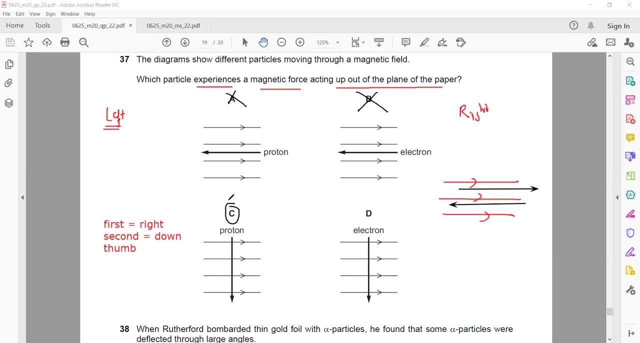 So when thumb is pointing towards you, it means it is out of the paper. 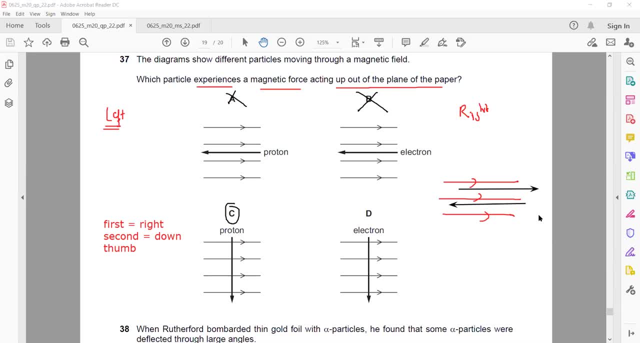 But when you apply a right hand, because electron is 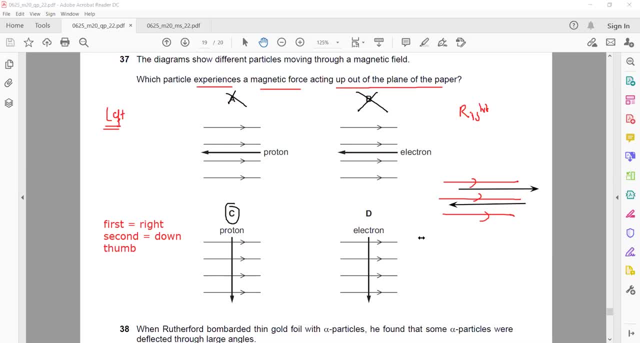 Because electron is a negative particle. So same rule is there, but 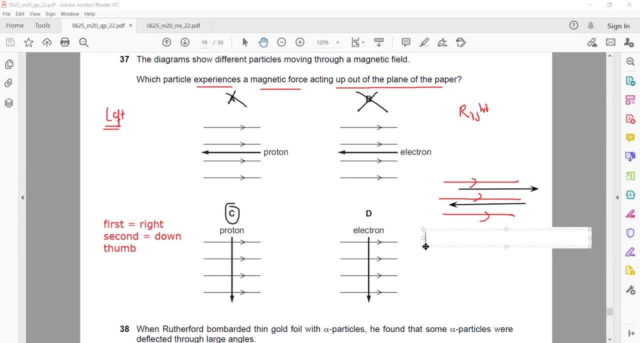 instead of left hand, you will use a right hand. So again, the first finger 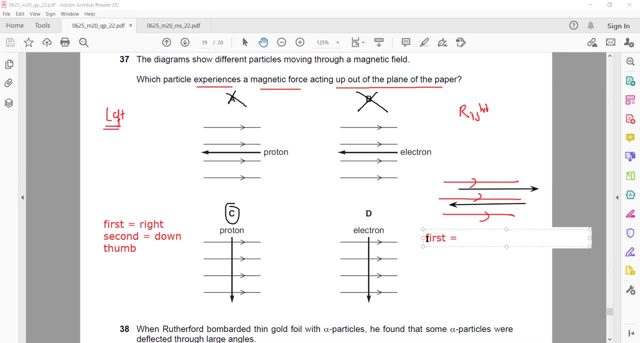 But your right hand, your right hand first finger should point towards the magnetic field. 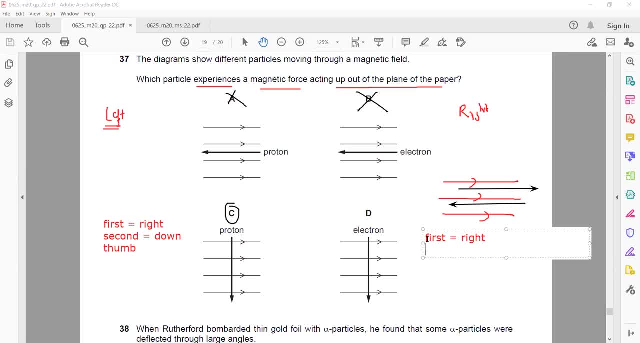 So that should point towards right side. Your second finger of the right hand should point towards the direction of the particle which is down. And where your thumb is pointing, 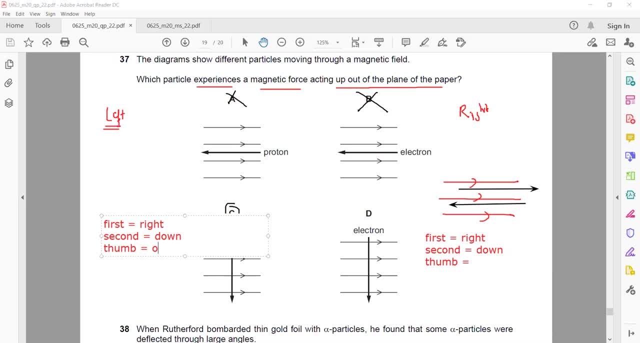 In the previous example, the thumb is pointing outwards. 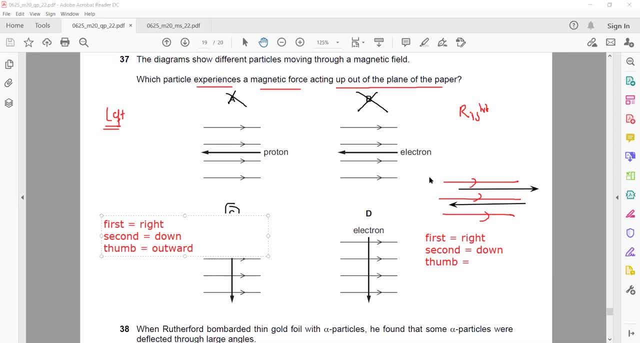 Your thumb, you apply a Fleming's You will apply a right hand rule. 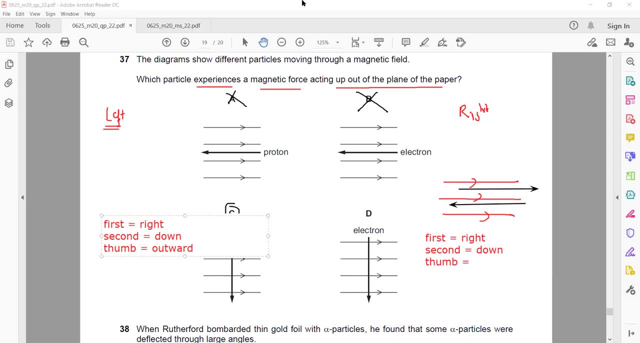 Your first finger should point towards All should be 90 degree to each other. 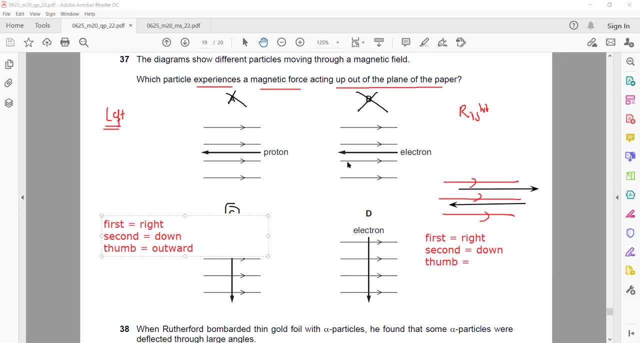 It's not It's a similar But instead of left hand, use the right hand. All should be 90 degree to each other. 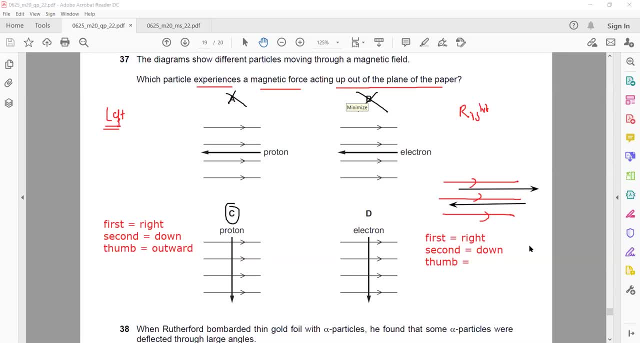 So with direction, your thumb is pointing into the plane or out of the plane. When you are applying a right hand rule. 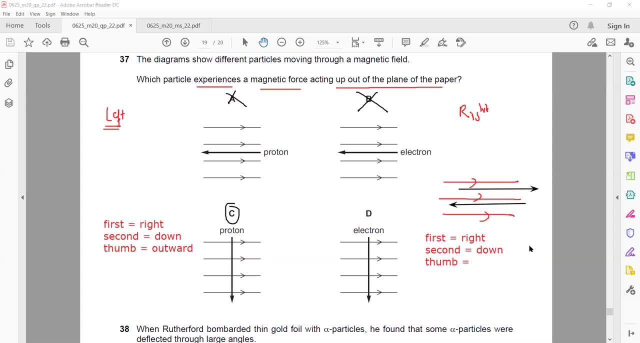 The same right hand rule like same way you use the left hand rule for the force. Yes, Salman. Sir, small confusion, sir. 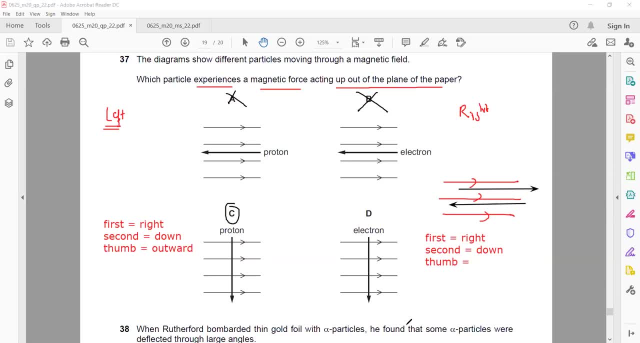 Last time we studied about south pole and north pole. 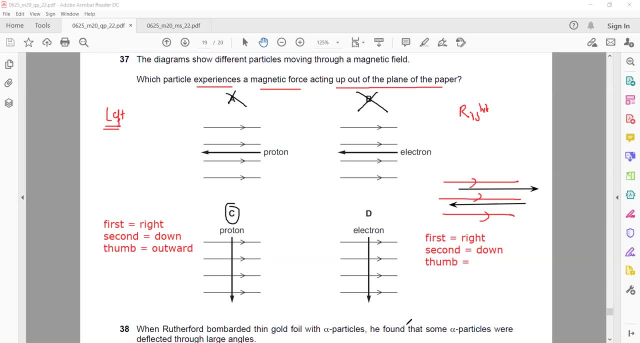 That was about the magnetic effect of current. What is the magnetic effect of current? Means when a current is passing through a wire and if you need a direction of the magnetic field, you can use that rule. 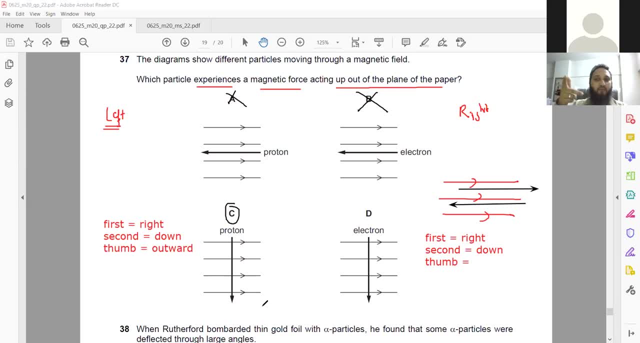 So for left and right hand like example, this was left hand rule. When you are finding a force on the wire or force on the particle in a magnetic field, you are using this left hand rule. First finger 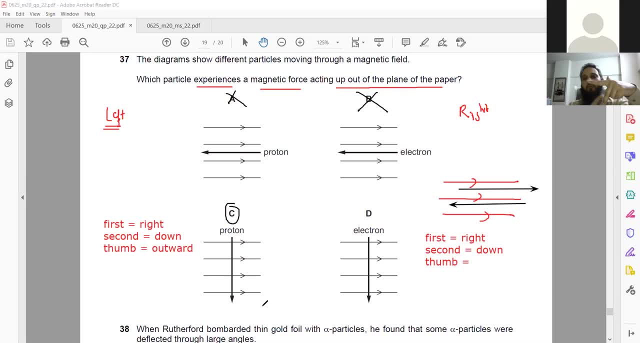 point towards the direction of magnetic field. Second represent direction of the particle and thumb is pointing in the direction of the force. 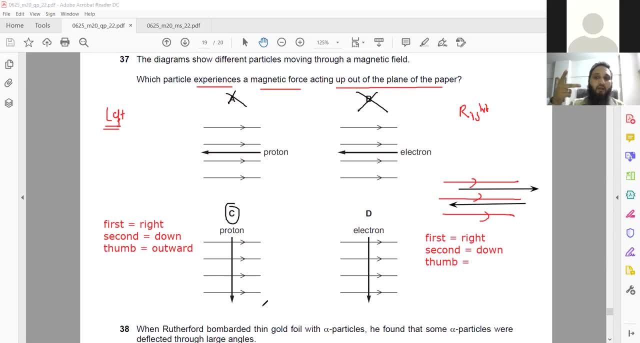 When you are finding a force on the particle in a magnetic field, you will use right hand rule in the same manner 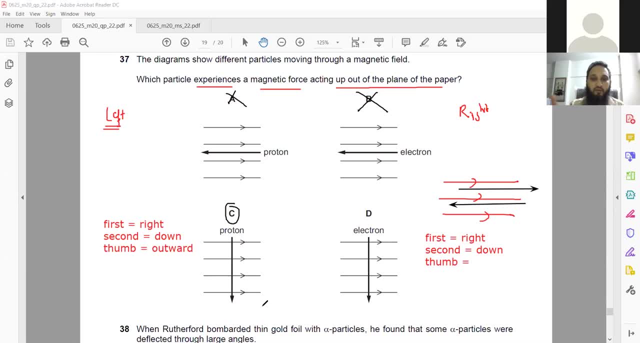 as left hand rule. This part you will study in atomic physics but because already you studied the rule that's why I am discussing this question. 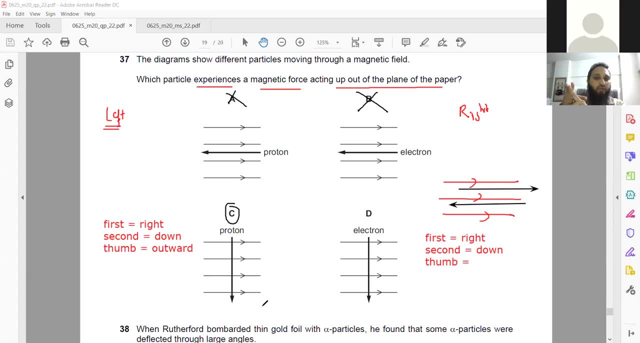 So first in this case for a right hand rule, your first finger should point towards south for a negative particle. So first finger is pointing towards the south which is towards right or the direction of a magnetic field. My second finger should point in the direction of the particle. The particle is moving downward. Where my thumb is pointing? 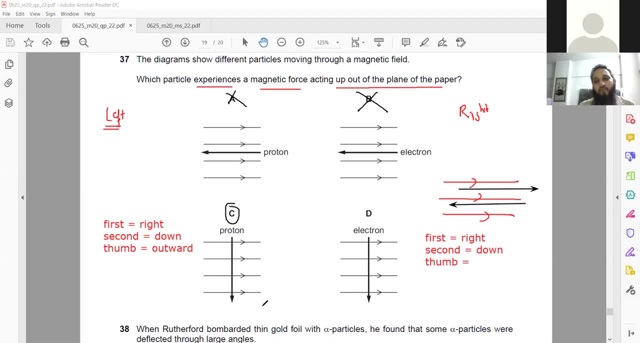 Which direction my thumb is pointing? So that is into the paper. 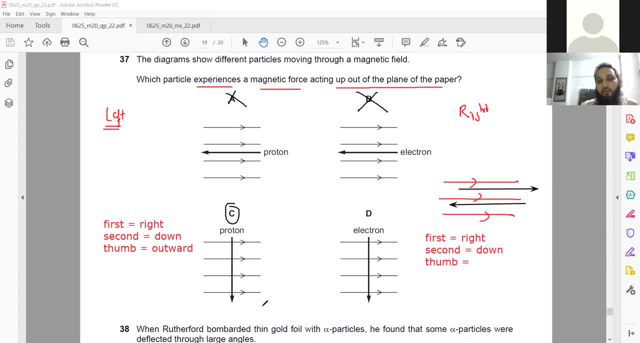 So if it is pointing into the paper if you apply a yeah it is this is called into like when I apply a right hand rule for a negative particle it is into. When I apply a left hand rule for a positive particle it is out of. So basically this proton will experience outward force and this electron will experience inward force or into the So which direction it will experience? So the question was which particle experience 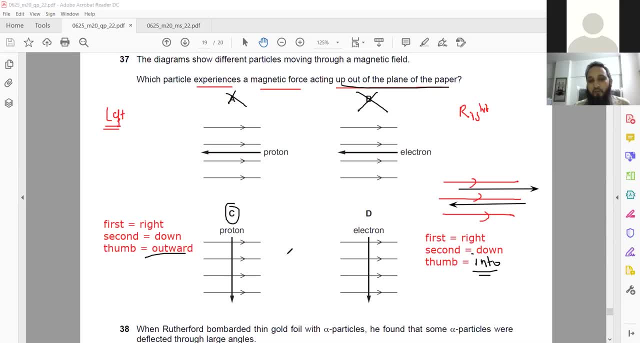 a magnetic force acting up out of the plane of the paper? 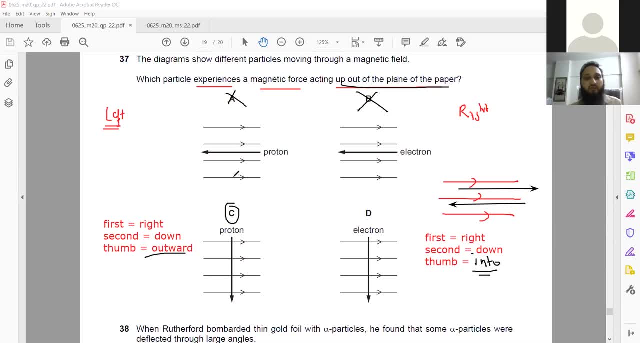 So which of them is acting out of the plane of the paper? So in case of C 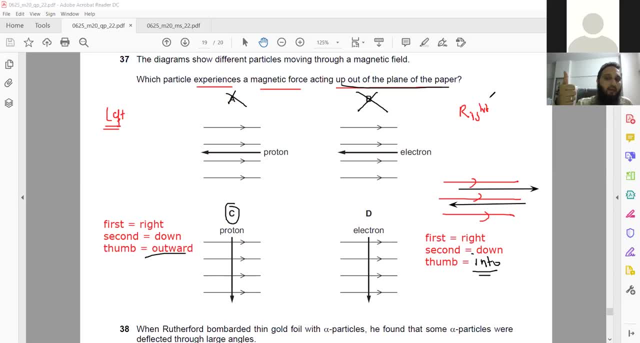 it is pointing out of the plane of a paper. This right hand rule grip rule is used to find the direction of the magnetic field due to a current carrying conductor. Is it clear? Sir. Yes. 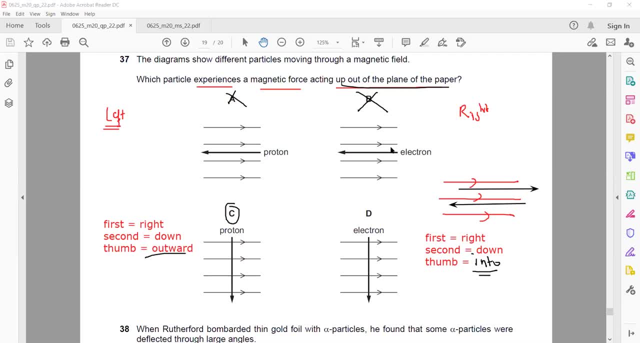 Where is the magnetic field and like where is the north and south? Where is the north and south? 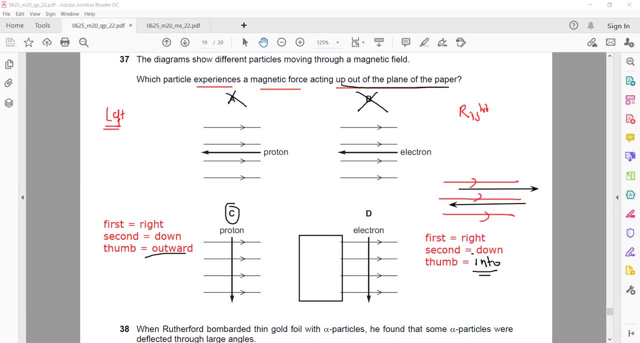 The direction of the magnetic field is from north to south. So basically on the left hand side you have north and on the right hand side you have south. They did not show that they just represent the direction. 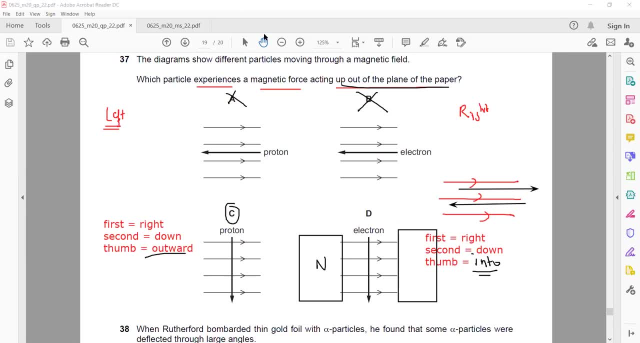 They did not show the poles but the direction of the magnetic field is from north to south. So this is a magnetic field and the particle is moving perpendicular to the magnetic field. So you are finding the force which is experienced by the particles. So 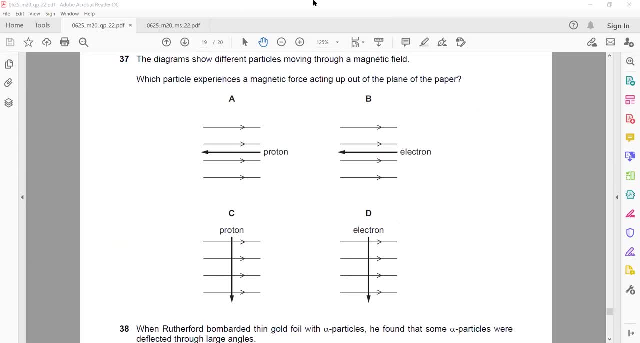 the rules look you have different rules. Sir so. Yes. 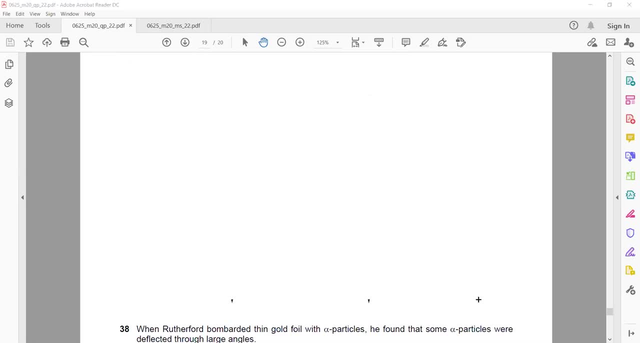 Continue. Sir we will not find okay now sir it's confusing. I think I understand. 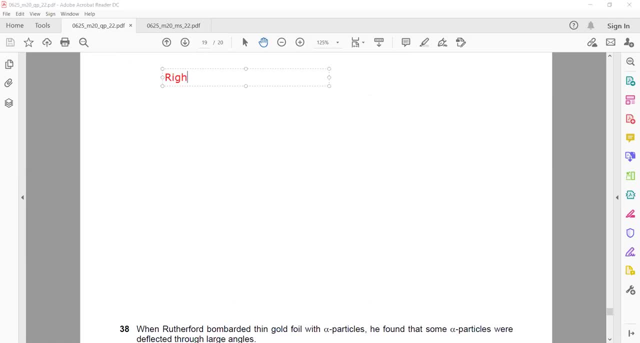 Look the rules are first one is a right hand grip rule. 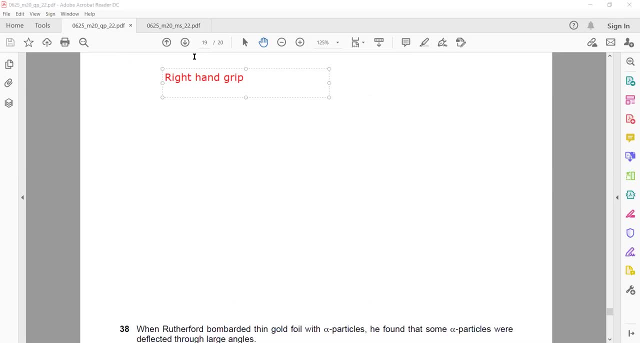 Right hand grip rule where we use it is used 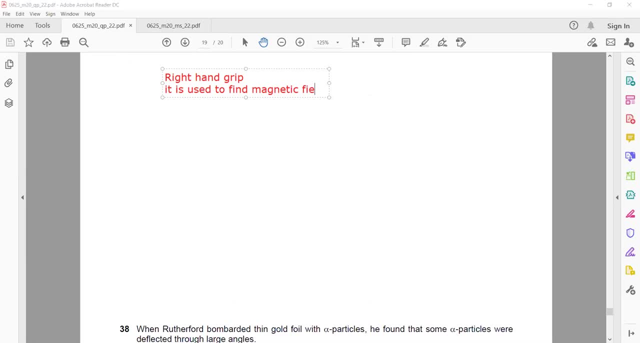 magnetic field produced due to current carrying conductors like the wires. 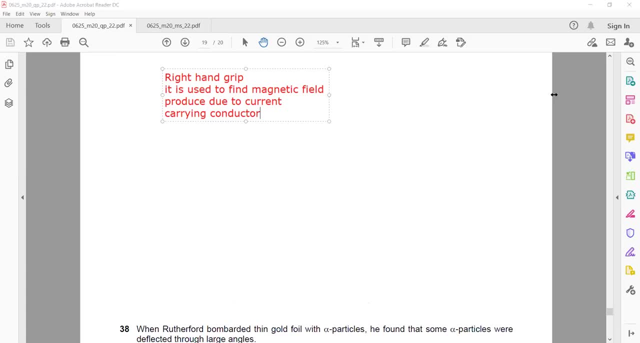 So the magnetic field if you want to find the magnetic field produced by the current carrying conductor we use a right hand grip rule and this right hand grip rule is divided into two parts 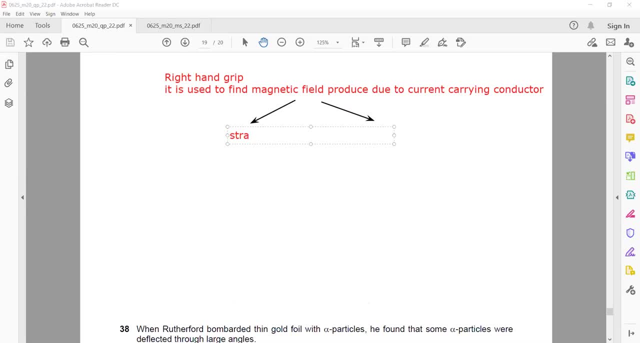 it can be a straight wire or it can be a circular wire or a coil or a solenoid. 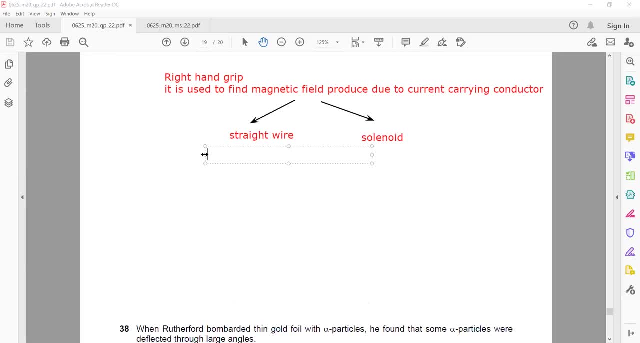 So for a straight wire if the wire is straight our thumb will represent the current 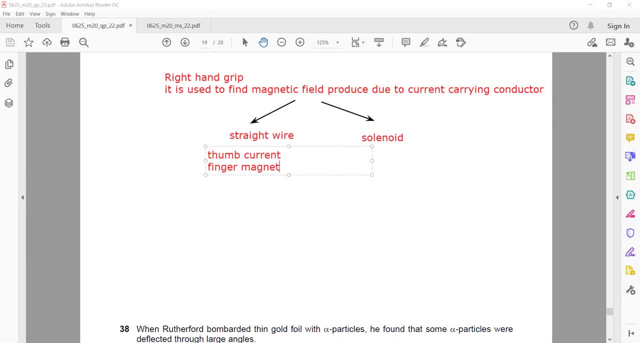 and fingers will turn in the direction of magnetic field. 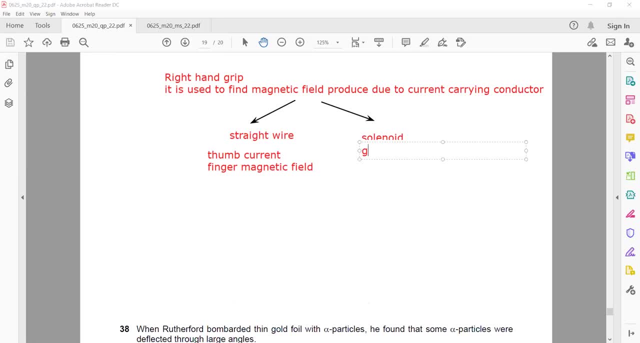 But if it is a solenoid or a circular wire our fingers will turn in the direction of the current magnetic note. 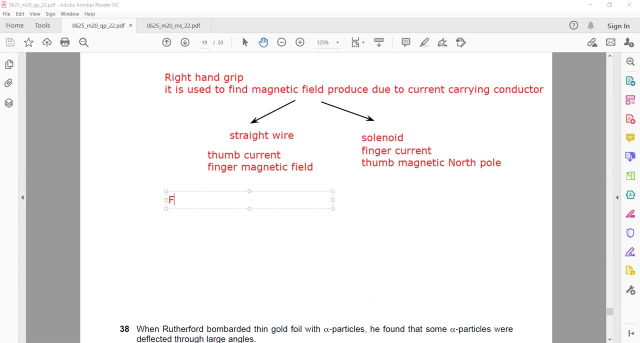 Then there is a Fleming's left hand rule. 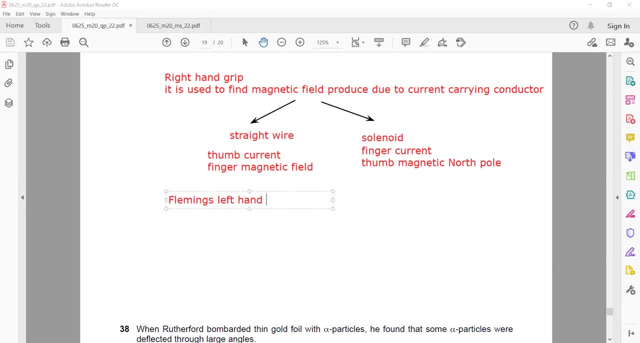 The Fleming's left hand rule it is where we use it is used to find 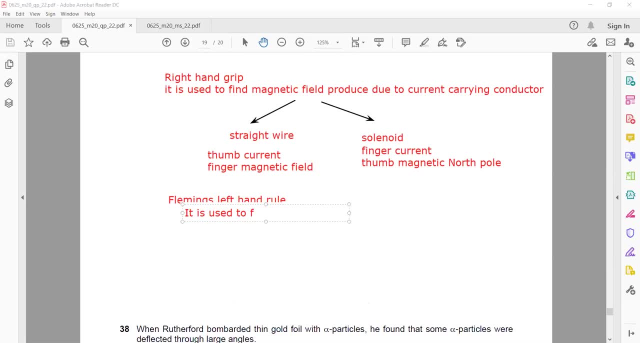 force on wire or positive charge moving perpendicular or perpendicular to the current perpendicular or 90 degree to magnetic field. 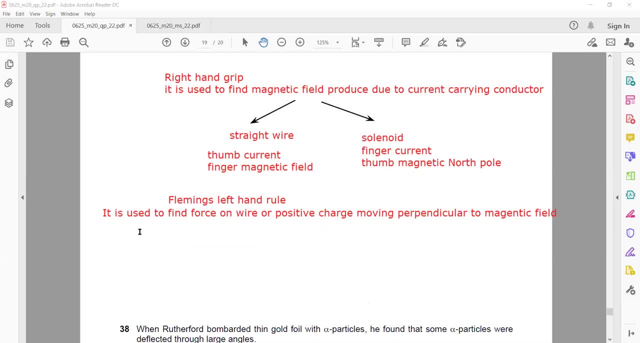 So it is used to find force on wire or positive charge moving perpendicular to the magnetic field and in this case the first finger the first finger the first finger represent magnetic field or pointing towards south. 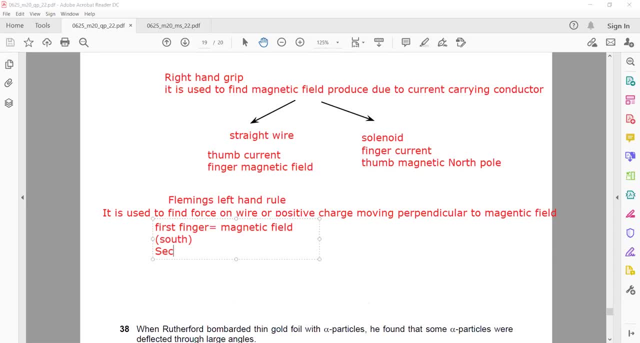 The second finger shows the direction of the conventional current or particle. And the right hand rule in this case will be represented by a ofейств fragrance . 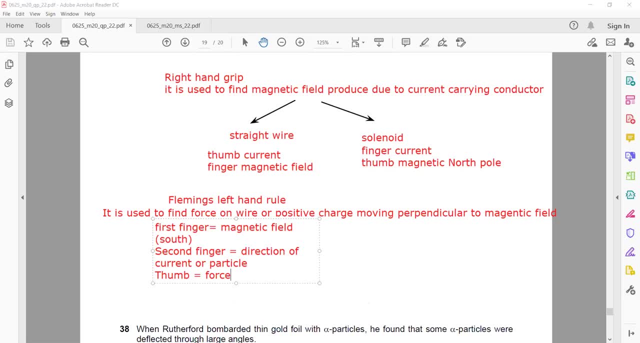 And the thumb will represent the force. 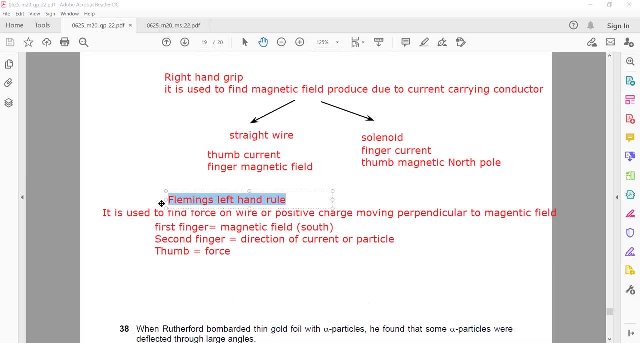 Then there is another rule which is known as right hand rule then this right hand rule can be used to find two things it can be used to find the direction of the current produced due to change in magnetic field or it can also be used to find the direction of the force so there are two ways which we can use 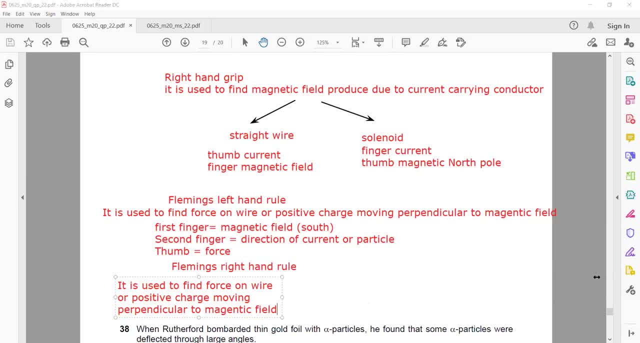 it is used to find the force on negative charge which is moving perpendicular to the magnetic field or it is used to find 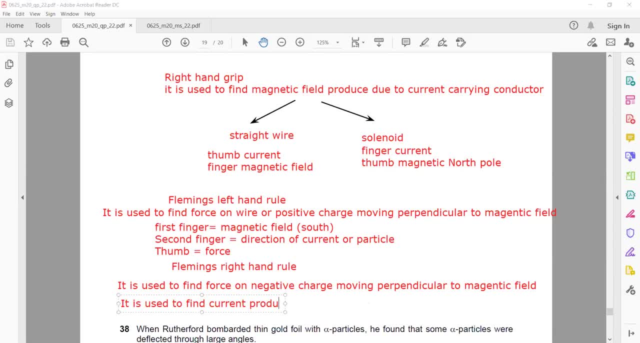 current produced or the direction of the current produced due to change 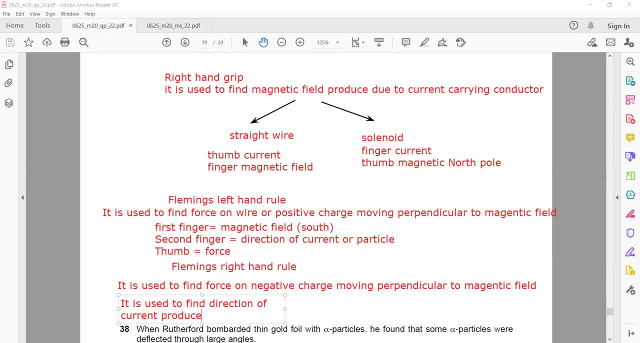 change in magnetic field this is a revision part but for each rule i will make one session in which i will discuss each rule 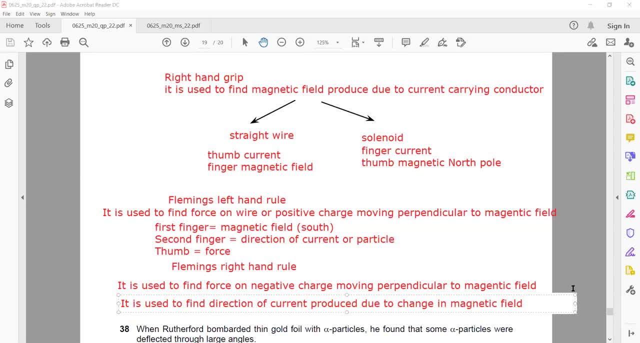 so you can have examples related to each i will in but this is just an overview because i'm discussing the mcqs right now so i'm not going in detail but next session for each rule i will give you example as well so you can have notes of that so these are the rules which you have to keep in mind for magnetism and electricity the right hand grip rule fleming's left hand rule and fleming's 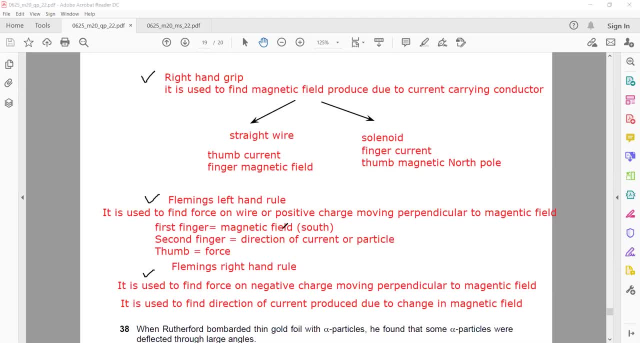 right hand rule and then according to this right hand also first finger represent magnetic field second represent the direction of induced current and thumb is a movement of the wire or the force 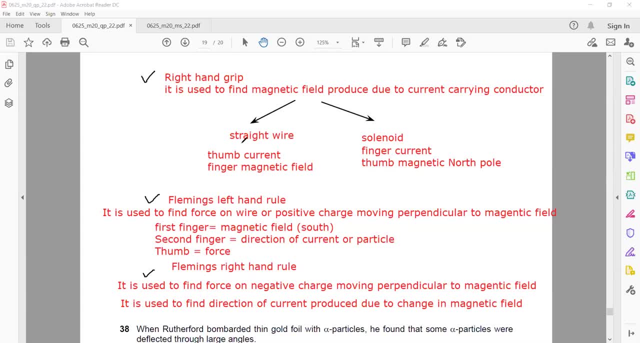 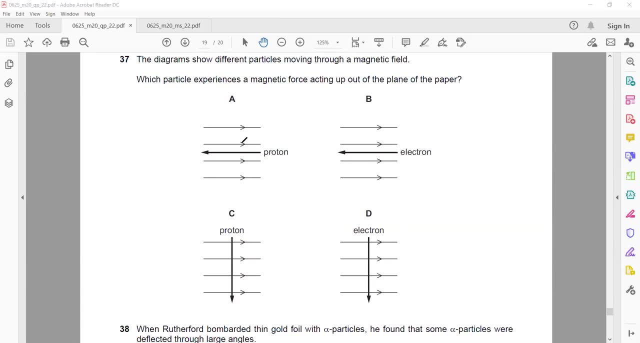 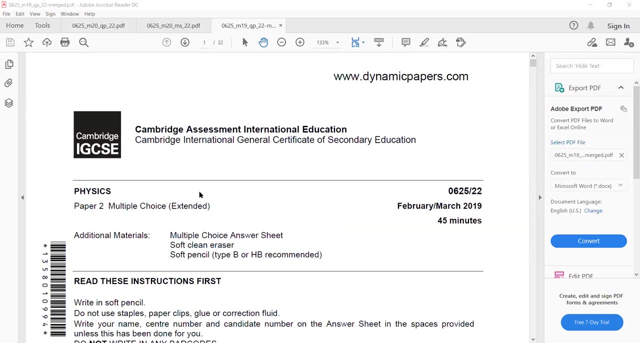 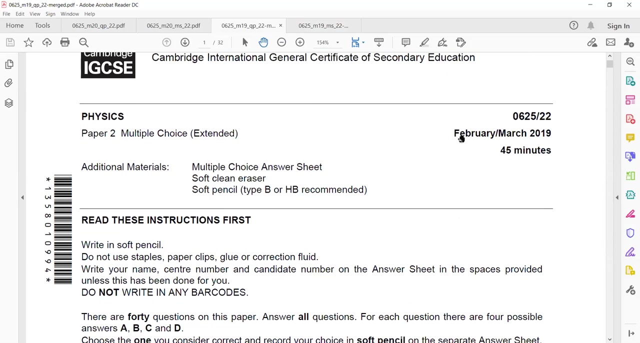 this is february march 2019 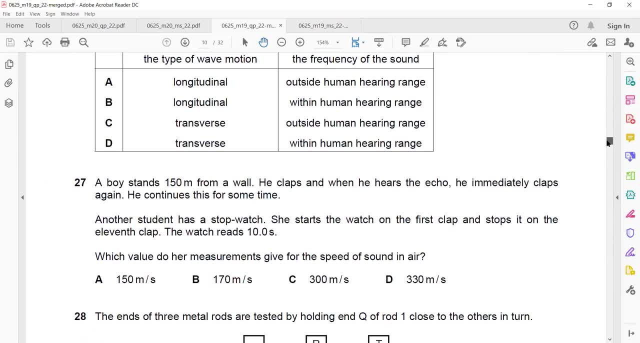 and i'll discuss electricity and magnetism questions with you question 28 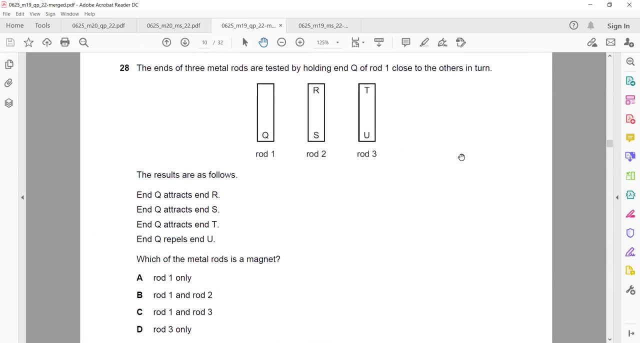 the end of three metal rods are tested by holding nq of a rod close to other ends so nq of a rod is placed close to the other rods as well when nq place near end r it is attracted when it is placed at end s it is also attracted but when nq is placed at t it is attractive attracted and when it is placed near u it is repel which of the metal rods are magnets 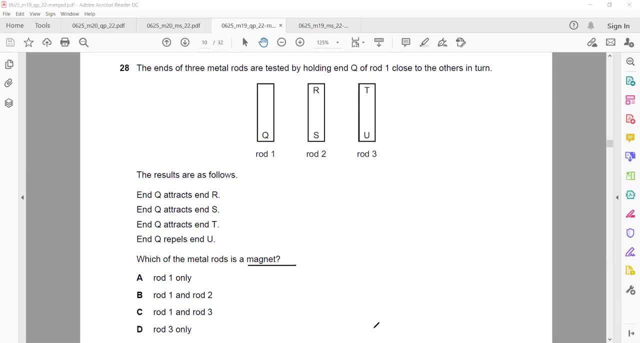 m which of the metal rods are magnets 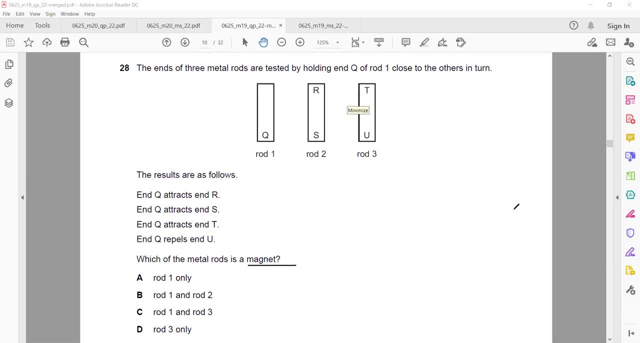 so for magnets like poles repel and unlike poles attract. So 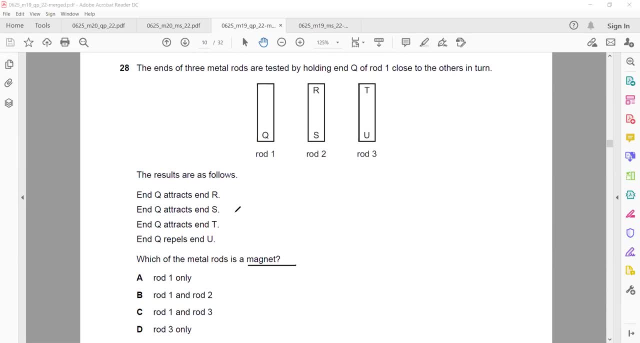 rod 1 and 3 rod 1 and 3 but what about rod 2? Rod 2 is made up of magnetic material but it's not a magnet because it is induced magnetism opposite pole will induce and it is always attracted. That's why rod 1 and 3 are the magnets. 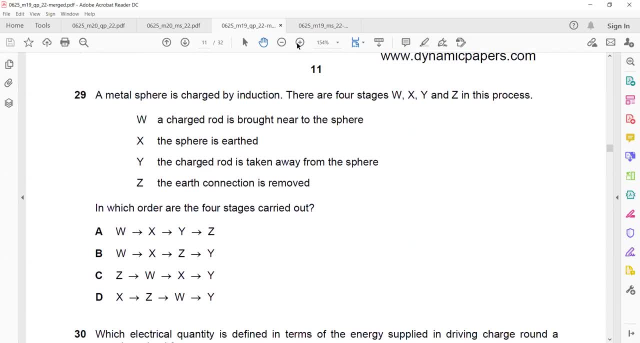 The metal sphere is charged by induction. Induction means just a quick revision what happened in induction if we have a material we want to make it charged. So we use a charge rod. So this charge rod will create a distribution. 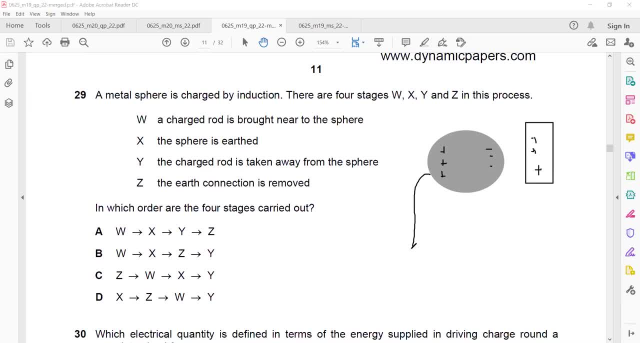 Electrons can move. Positive charges cannot move. Then we connect an earthing wire which allow the charges to flow in or out according to the what charge we bring and then we do another process which 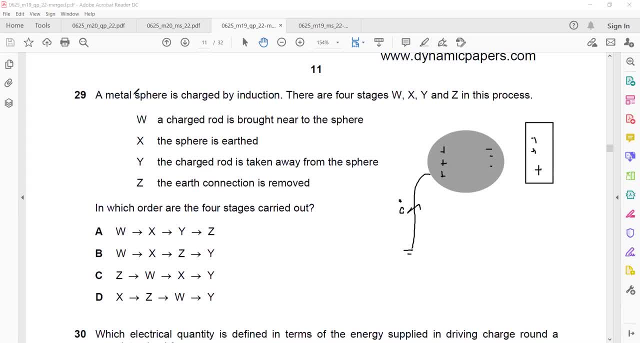 will make it permanent charge. So in the question basically an object is charged by the help of another charge object we call that as induction. 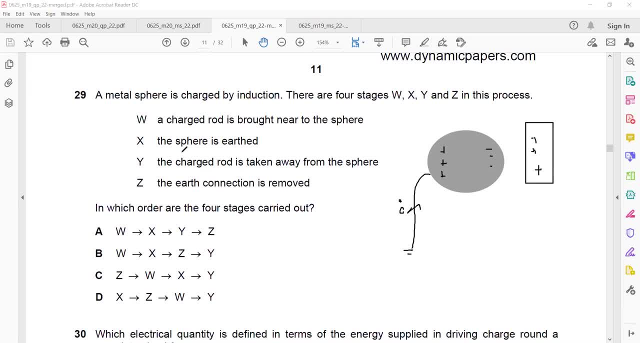 So there are four stages W, X, Y and Z in this process. In which order are the four stages carried out? A. 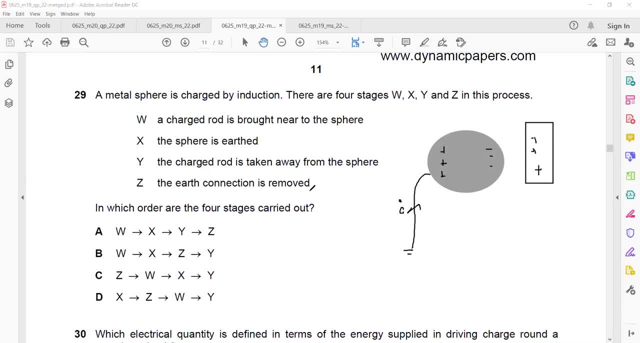 2012. 12. 13. 14. 15. 16. 17. 18. 19. 20. 21. 22. 24. 25. 26. 26. 27. 28. 29. 30. 23. 24. 27. 30. 31. 35. 31. 24. 32. 26. 39. 33. 34. 35. 34. 35. 36. 37. 38. 39. 40. 42. 42. 43. 44. 45. 42. 54. 45. 46. 46. 46. 47. 51. 48. For question 29. 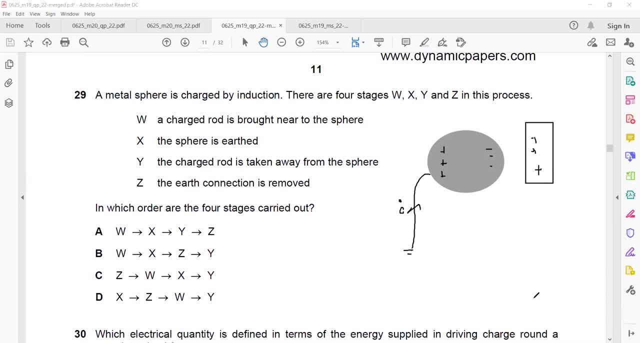 Salman, you have a question. You raise hand. No, sir. I may be forgot. Okay. Raise hand. Sorry. 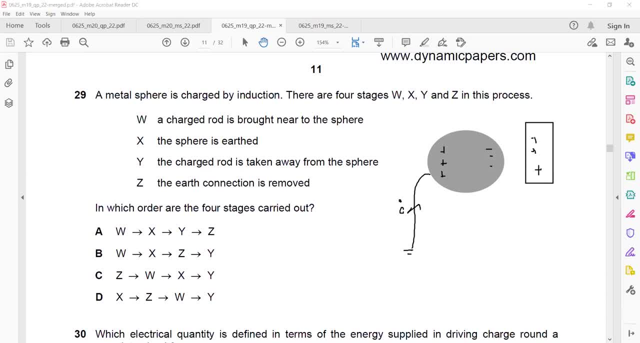 So what is the right order? I want participation from everyone. Okay. 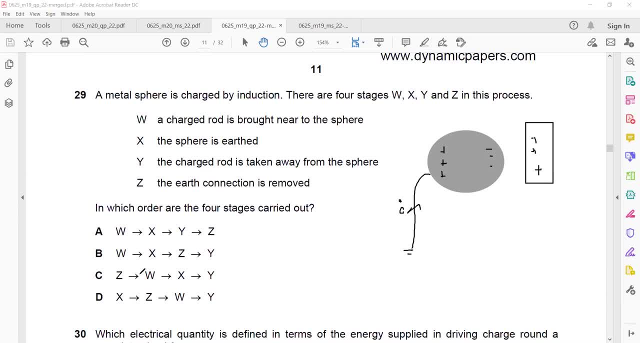 So in which order the four stages are carried out? 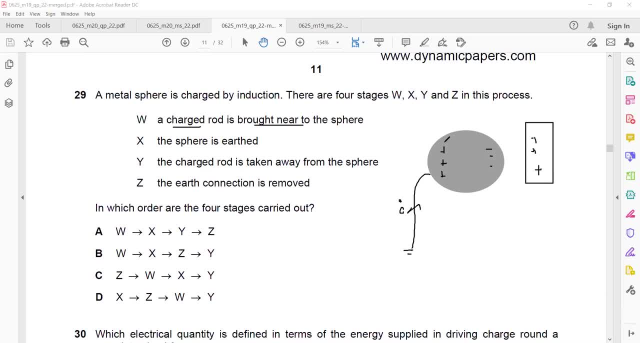 A charge rod is brought near the sphere. So first we'll bring a charge rod. 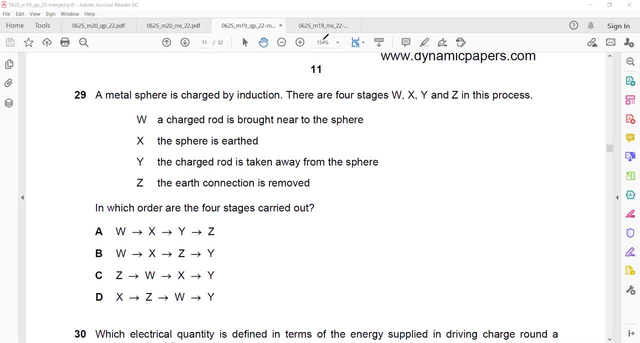 So first we'll bring a charge rod because that's first we want to create a distribution of the charge. So to create a distribution of the charge, we should bring the charge rod. 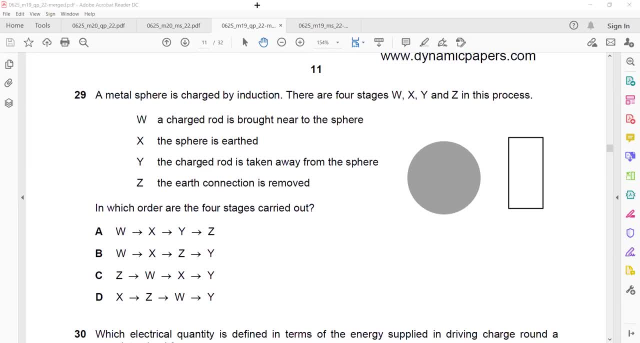 So when we bring the charge rod, what it created to create a distribution of charges. 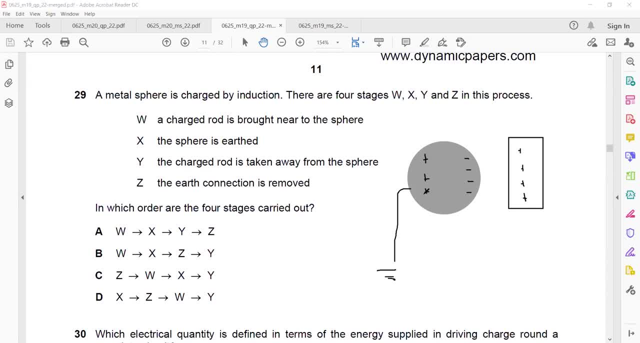 Then we connect an earthing wire. So when we connect an earthing wire, the charges will flow in. So there will be positive charges, but majority of them will be negative. 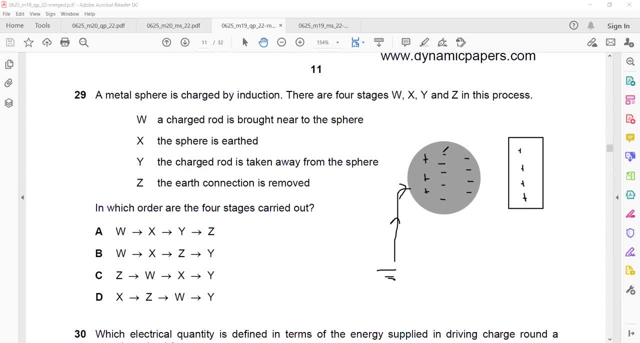 And if you want to make it permanent charge, then because we don't want the charges to flow back. If you remove the charge rod away. 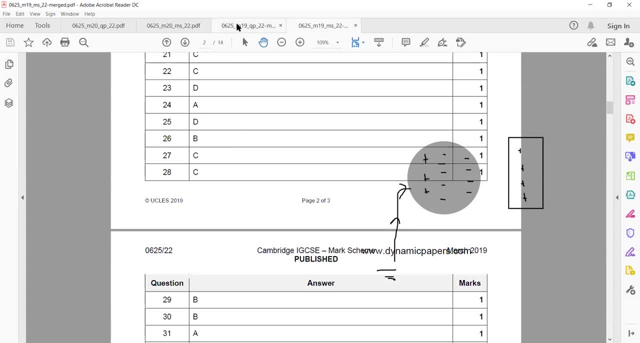 You can see for question 29. B is given. Why B is given? As you can see in the question. Because if we remove. For question 29, why B is given here? Yeah. 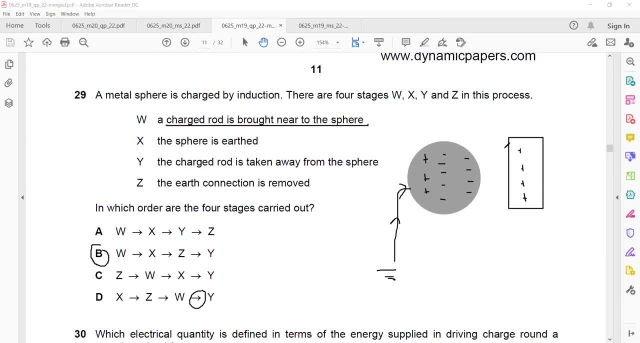 First, the charge rod is brought near the sphere. That's we did first. Clear. Then we connect an earthing wire. When we connect an earthing wire. So the charges will flow in. 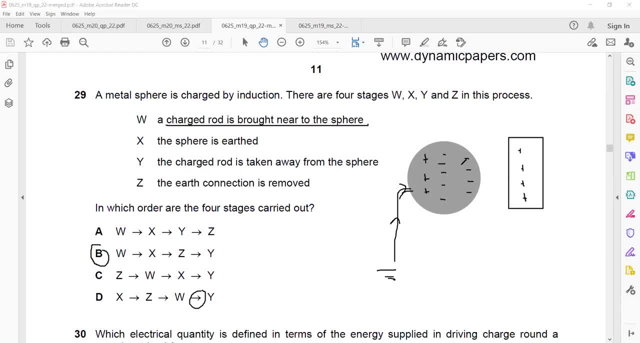 So majority of them will be opposite charge. Then which one we should remove first. 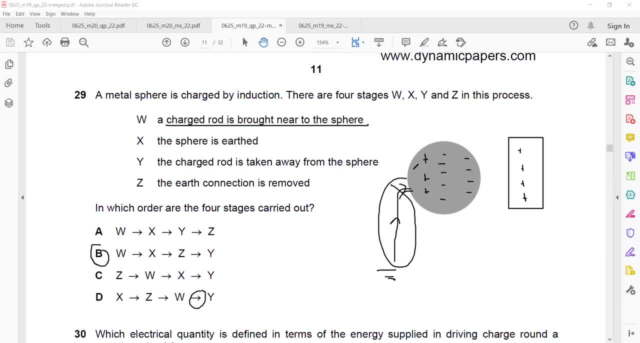 We should remove the earthing wire first. Because when I remove the earthing wire first, the charges cannot return back to the earth. 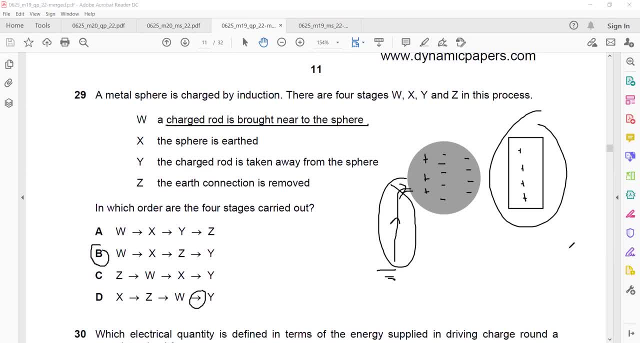 And then at the last, we will remove the charge sphere. 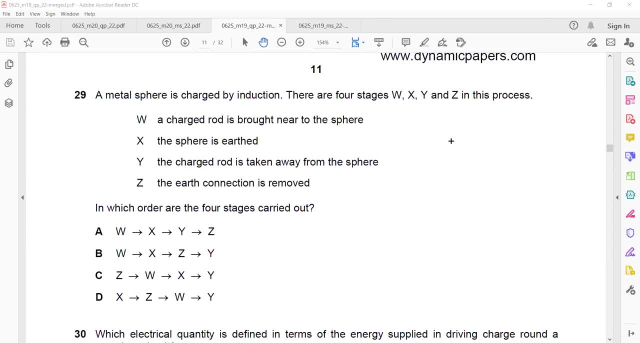 If you remove the earthing at the last, it will not be permanently charged. 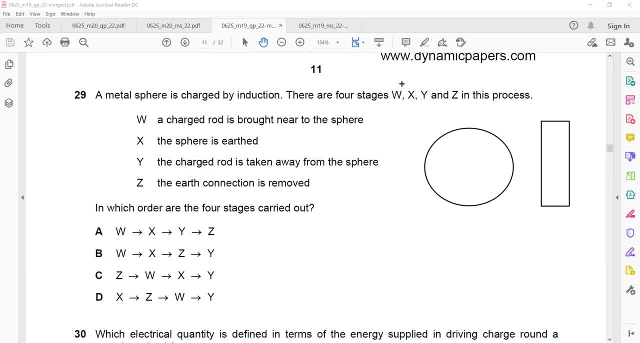 Why it will not be permanently charged? By example. You have a positive charge or you can bring negative as well. 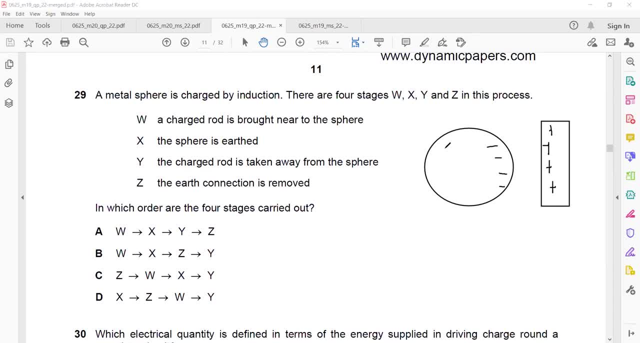 If you bring a positive charge or it create a distribution of the charges, negative one side and the positive other side. 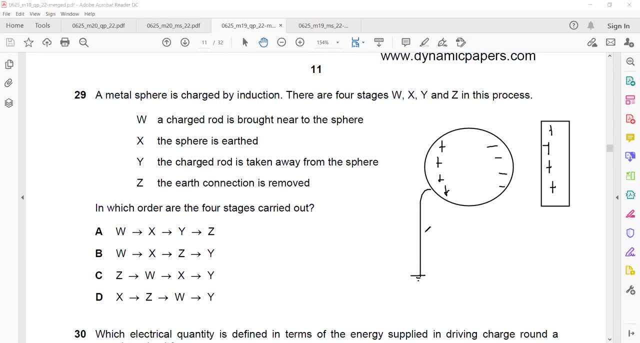 If I connect an earthing wire. So when I connect an earthing wire, because the positive attract the negative charges. So majority of them will be negative. There are positive, but most of them are negative. 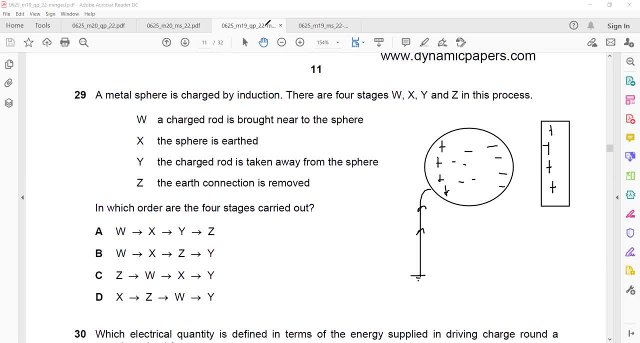 Now, if I remove this charge rod first. So if I remove this charge rod first, the light charges because majority of them are negative. So light charges repel. 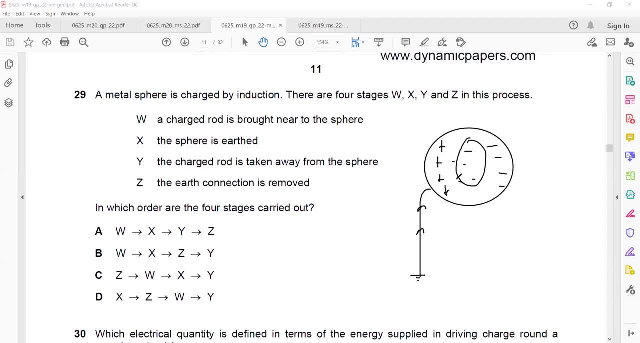 So what it cause it cause a negative charges to flow back to the earth. 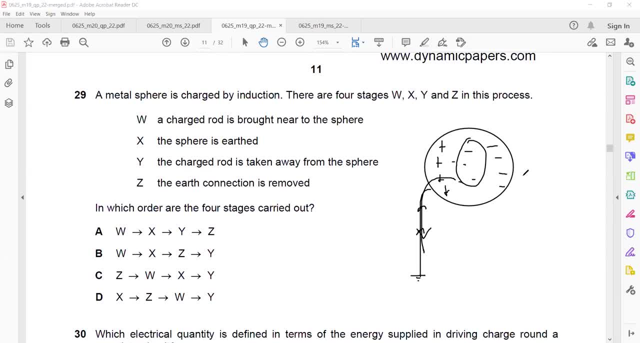 So as the negative charges will flow back to the earth again, this is sphere will be neutral. So it will not be effective technique. So what should be the order first W means a charge rod brought near to the sphere. Then X the we connect the earthing wire. Then we should remove the earthing wire so that the charge cannot return and at the last we remove the charge rod. Is it clear now? Yes. 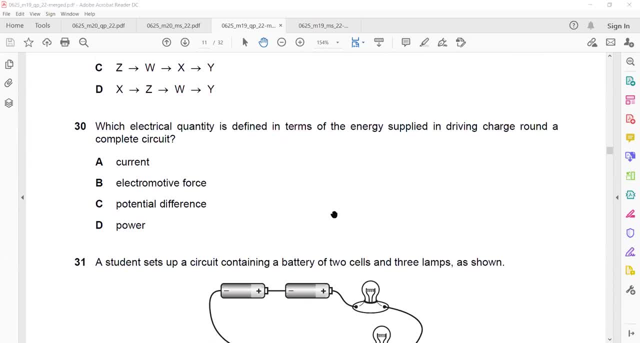 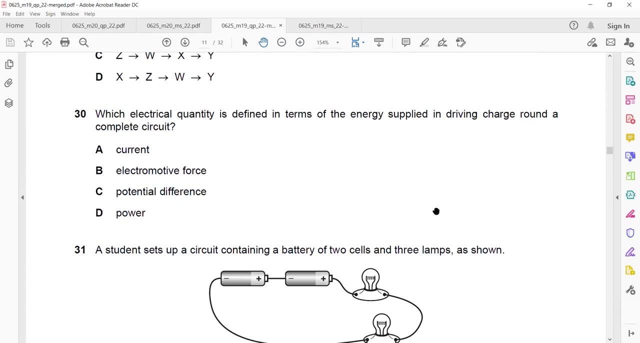 Question 30 which electrical quantity is defined in terms of energy supplied in driving the charge around the complete circuit? Energy. 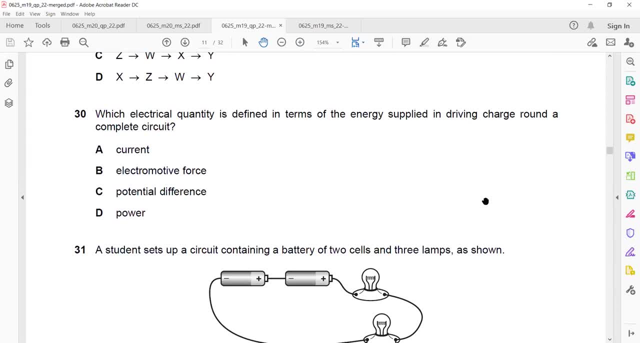 required to drive the charge to move the charge around the circuit that's the definition of emf electromotive force potential difference is how much work done by the charge or how much energy transfer by the charge both of them have a units volts but the only difference this one is how in the charge get energy from the battery that's known as the emf and potential difference is how much charge transfer energy when passing through a circuit 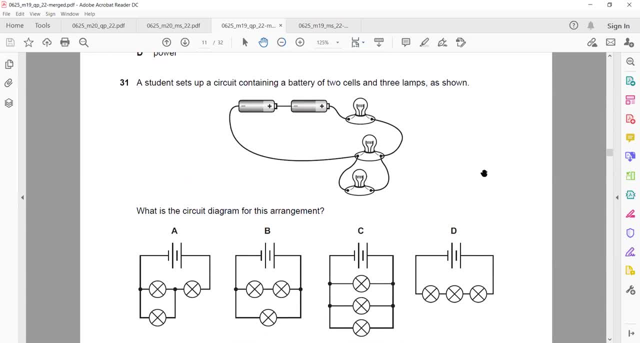 that's known as potential difference question 31 a student set up a circuit containing a battery 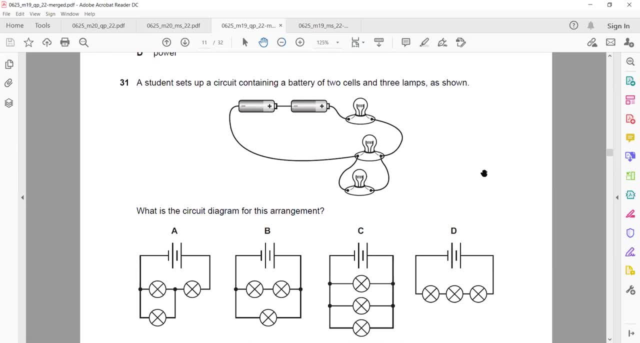 of two cells and three lamps which diagram represent what is the circuit diagram for this arrangement 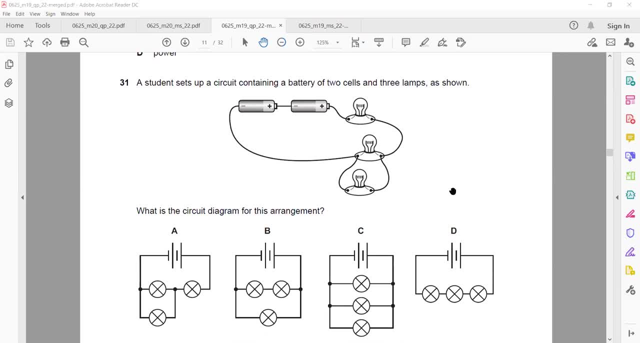 so to understand the circuit diagram just a small thing what you will do you will replace these components by the symbols like first I have a cell then also I have a cell makes a battery then this is connected to a lamp and the other part of the lamp is connected to another lamp and there's another lamp in parallel and then the circuit complete so it means the two lamps are parallel and one of them is next to them is series so which one is a correct circuit diagram so in this case a is a correct so the simple way to understand like when which circuit diagram is correct just replace the component by the symbols and you can identify the correct circuit diagram because this is the same thing like one lamp and 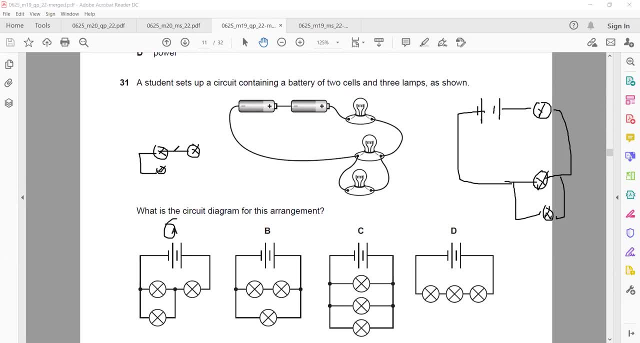 then the second lamp is the two lamps are in parallel to each other then connected to a battery or combination of the cells which make a battery 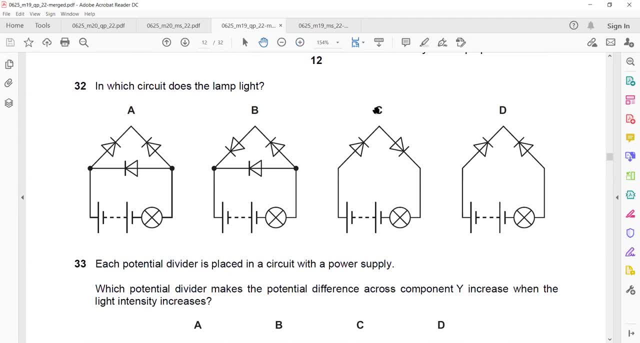 in which circuit does the lamp lights yesterday we discussed the function of a diode I will just recall that this is how let's call it the diode there's a diodeslight there's another diodeslight for the dys Convention circuit but let's say if the diode if the current is passing from the side of the play the diode allow that but if the current is passing from the side of the pause the diode will block so which of the circuit allow the land does the lamp light up basically which of the circuit conduct electricity in that circuit the lamp lighter C. I will here that's the right answer C is the correct answer Yeah. 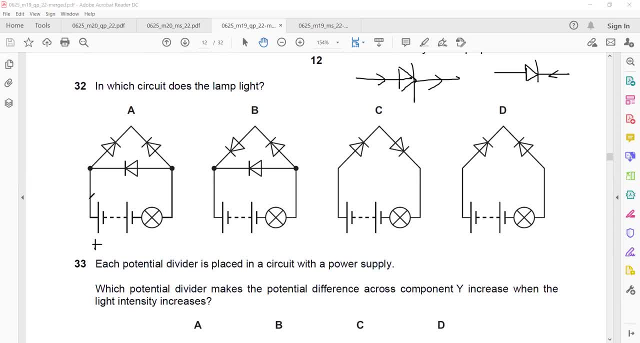 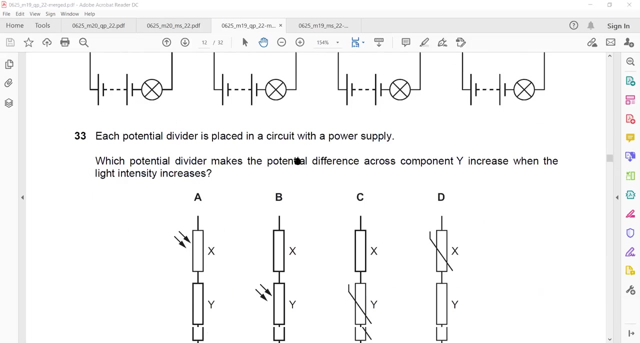 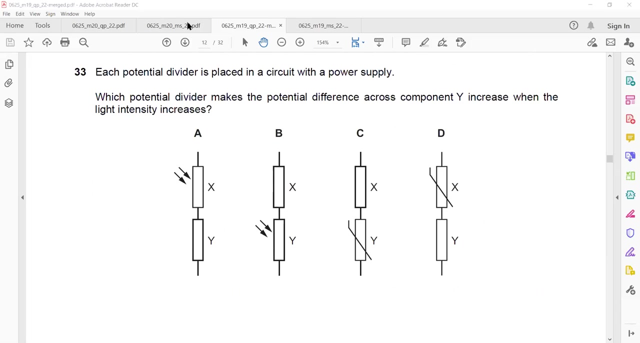 why not the other one look if you check the conventional current so this will block this first diode will allow but the second diode will block so there is no current in a for the second one when you check this diode both of the diodes will block see the answer but what about d when the current is coming the first diode allow but the second diode block so the lamp will be off but when you check see both of the diodes the direction of the current is from the side of the play so they allow and the lamp will light up okay each potential divider yesterday i told what is the meaning of potential divider it means when two resistors are connected in series they divide the voltage we call them as potential divider circuit two in in each potential divider is placed in a circuit with a power supply there is a power supply or 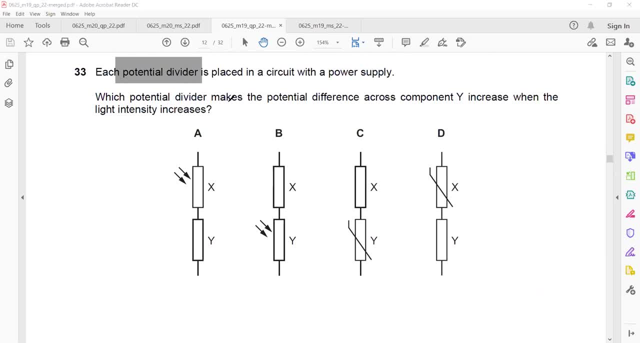 voltage supply there which potential divider make the potential difference across the component y increase when the light intensity increase so basically it should work with light so c and d cannot be an answer why c and d cannot be an answer you can see it's a thermistor thermistor it only work with temperature it does not work with light now what happened yesterday we discussed for ldr what happened when the light intensity increases when there is more light the resistance will decrease it is inversely proportional and we want so what happened if there is more light intensity then the resistance will decrease so here the resistance decrease in comparison this component will have more resistance so where the voltage will be higher at x or at y for x or at y at y the voltage will be higher and that's a question only that which potential makes which potential divider make the potential difference across the y increases 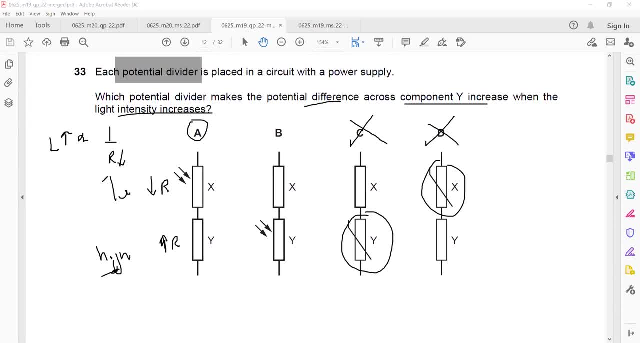 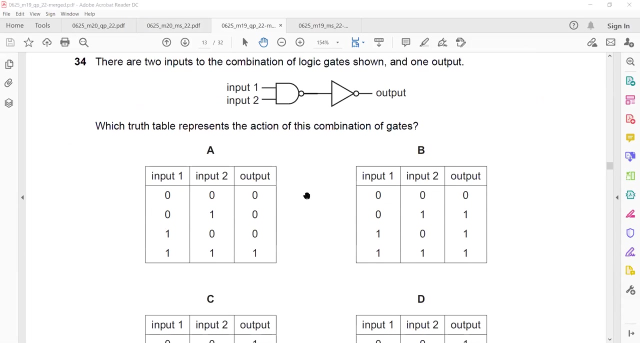 so a is the right answer why b is not correct answer because if more light intensity smaller resistance less resistance here in comparison more resistance so more voltage across x and less voltage across y but in the question we need more voltage across y that's why a is a correct answer 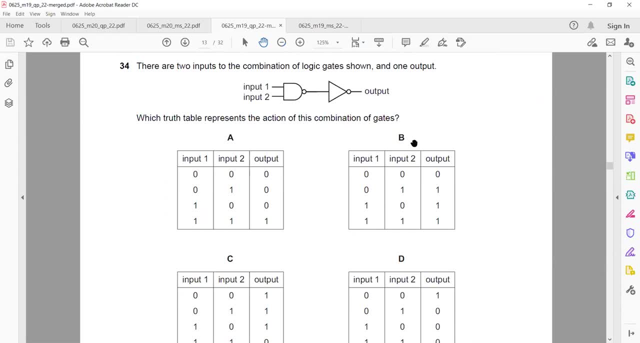 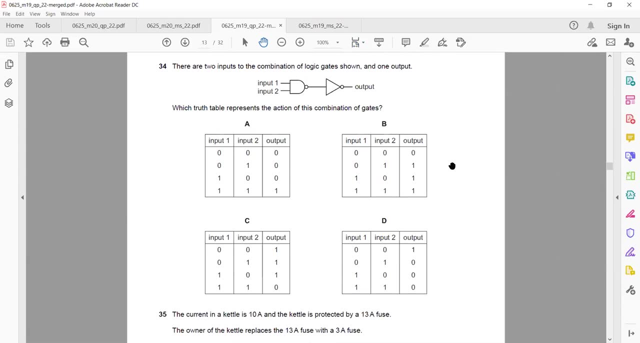 there are two inputs to the combination of a logic as shown and one output which truth table represent the action of this combination can you identify from the circuit which truth table is correct 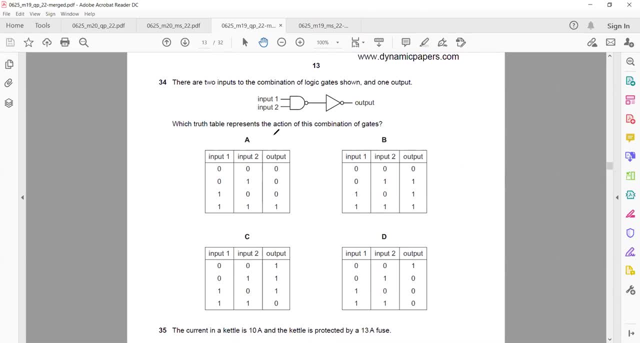 the way if you want to identify how you will identify you will check the table like zero zero what should be the output of nand gate 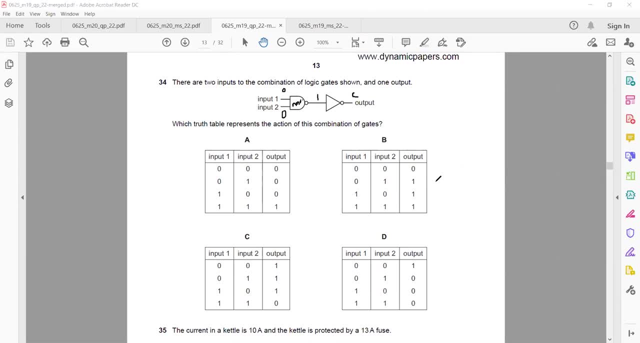 it should be one and then passes through inverter so it make it zero 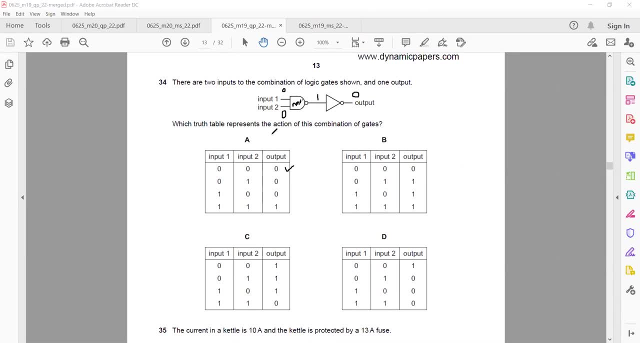 so first combination is right but i have to check all so first combination is right but i have to check all so first combination is right but i have to check all because it's not necessary that all of the combination so if it is zero one the output of this will be one and passes through inverter make it zero 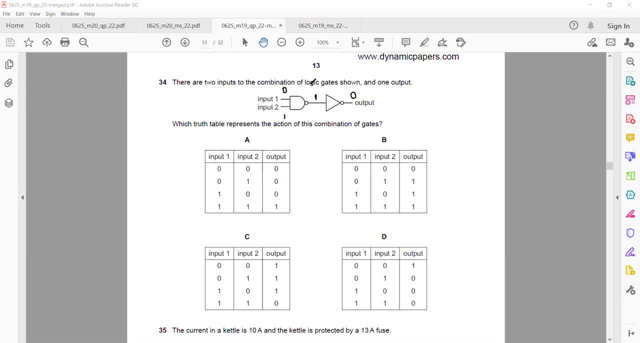 one zero it will also be but when we say one one when in both in one one is one but this is an and gate make it zero and zero will make it one so which logic gate is which table is correct so which logic gate is which table is correct 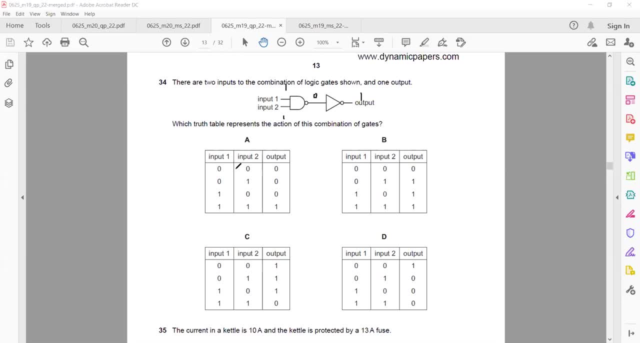 which of the truth table is according to the circuit look input a and the input two are when this one is zero this output means this one okay and the two inputs are there when both inputs are zero zero zero for nan gate for and gate it is zero but it's a nan it will 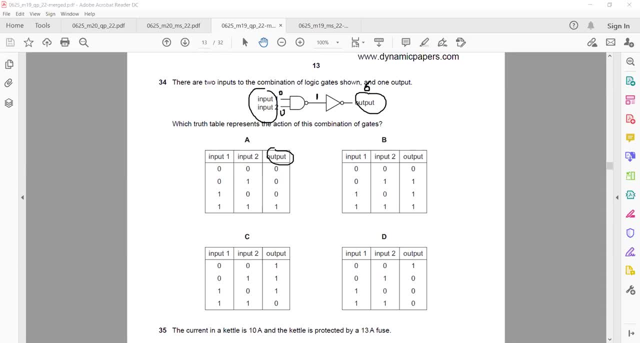 make it one and that one passes through inverter so that make it zero so when both inputs are zero 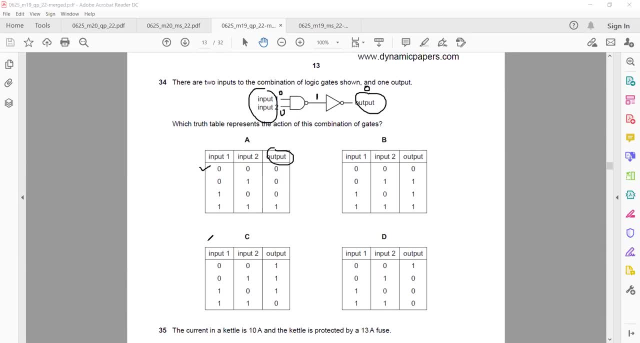 the final output is zero so first statement is correct now 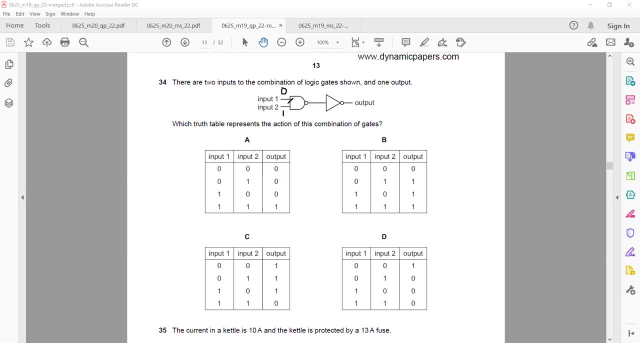 when you check the second statement zero and one zero and one zero and one is zero for nan gate zero for and gate but one for one for nan gate and that passes through inverter so it make it zero 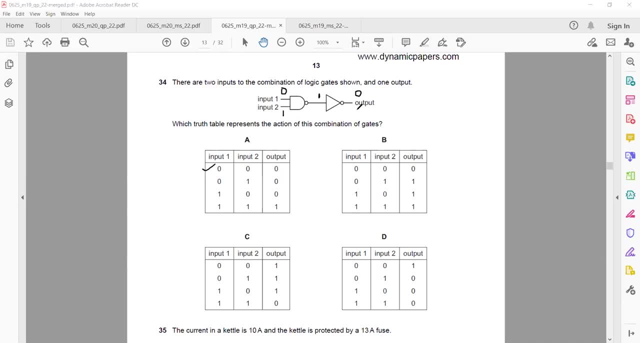 so when in input one is zero and input two is one the output is zero so second statement is also correct 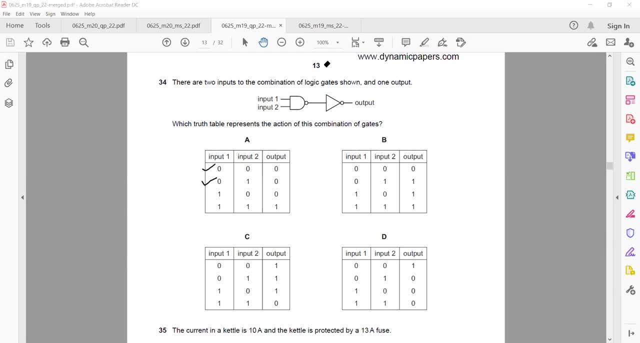 when you check the third one you check the third one it is one and zero one zero is zero for and gate but passes through this 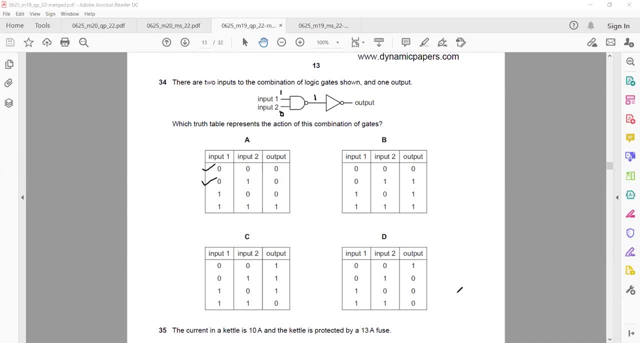 nan so it will make it one and one passes through the inverter so it will make it zero so the third statement is also correct 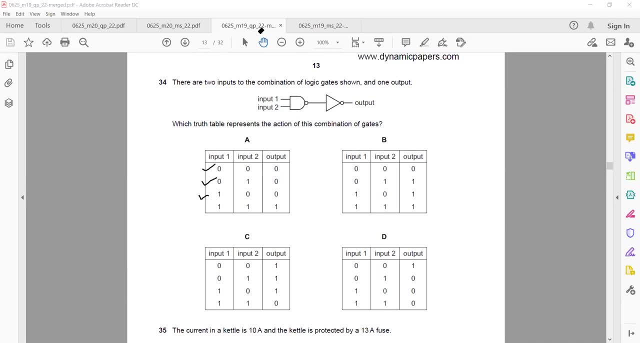 when you check the fourth statement one and one output of and is one but because it's a nan so it will make it zero and zero passes to the inverter it will make it one 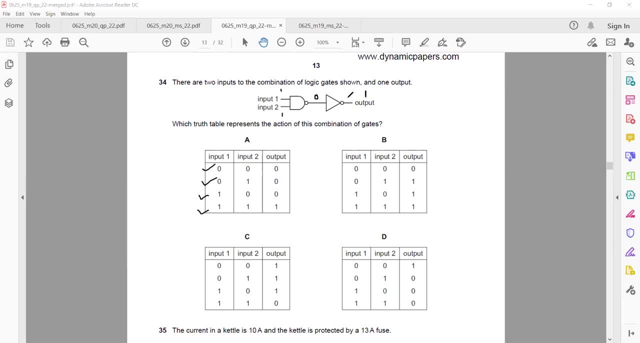 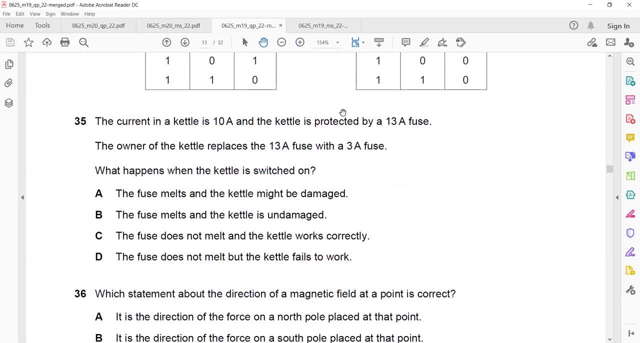 means truth table a is a right answer the other truth table are not correct because one of them is the right answer so you check when both inputs are there and the final output this is matched with the combination of this circuit 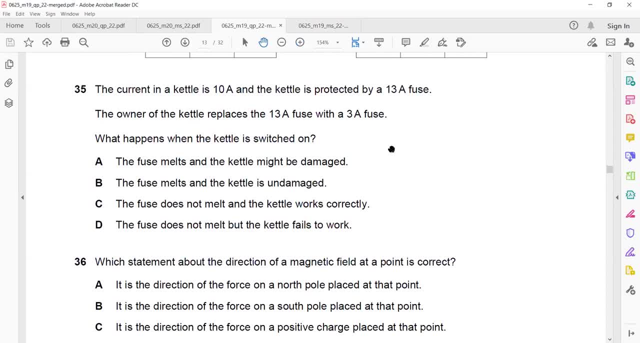 yesterday we discussed the fuse the current in the kettle is 10 ampere and the kettle is protected by a fuse of 13 ampere the owner of the kettle replaced the 13 ampere fuse with a 3 ampere fuse what happened when the kettle is switched on so 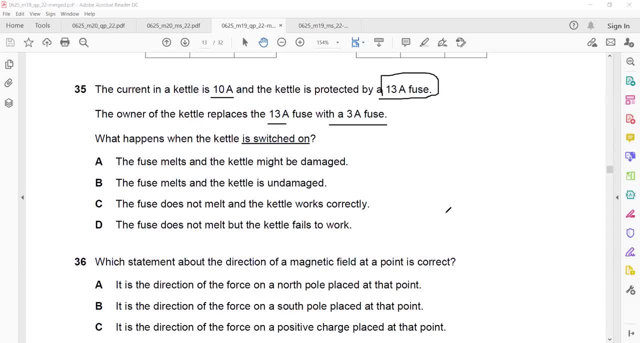 how the kettle will be damaged if the fuse below fuse is used to protect so a kettle the current is there 10 ampere that's and the kettle is protected by a 13 ampere so it means 13 ampere is enough the kettle can work with 13 ampere so yeah that's right basically the this is a like this is not a useful fuse because when we say it is protected by a 13 ampere fuse it means a kettle can work with 13 ampere but what happened if you just place a fuse of 3 ampere the fuse will melt and the kettle will remain undamaged 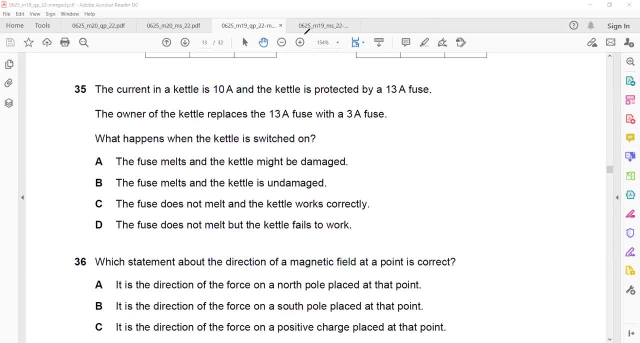 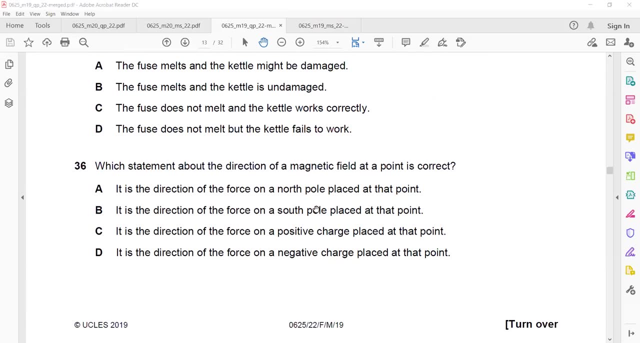 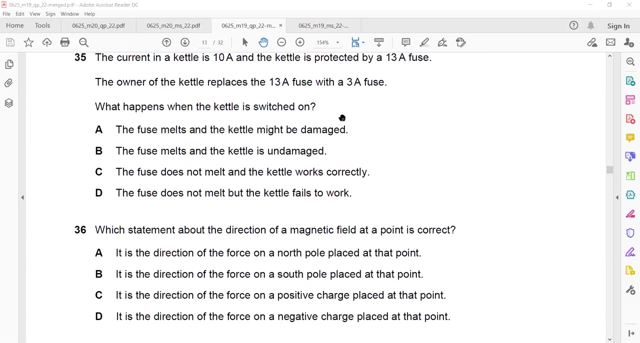 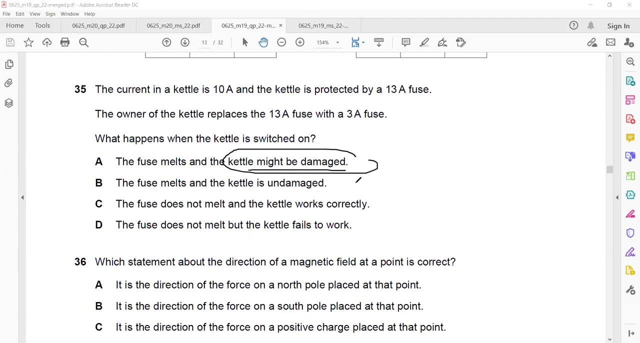 it cannot damage because 3 amp 13 ampere fuse is used to protect the kettle so it means the kettle can work with 13 ampere so if even a current is lower than 13 ampere the kettle will not be damaged even it might the reason is it might be damaged this this is showing a possibility that the kettle might be damaged because the kettle is not able to use power the fuse is the fuse melt so the current even is not able to enter the kettle so that's why it is there's there's no current in the kettle so it's not possible 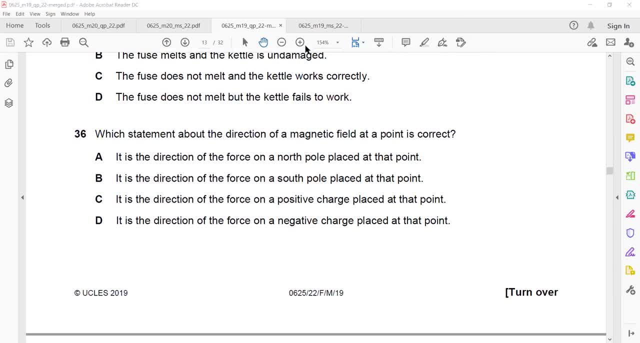 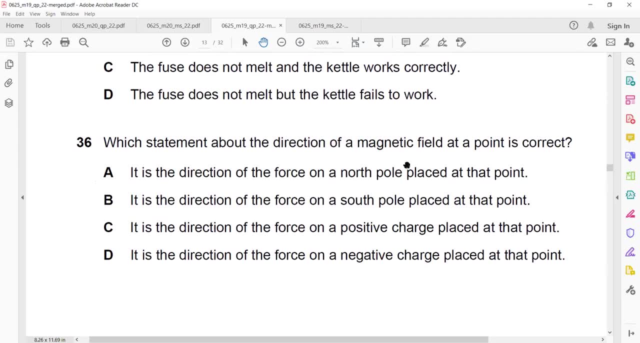 to damage the kettle like even there's no possibility that the kettle might be damaged at which statement about a oppose both gamer's challenge I makes sense I mean sounds like someone abi's question right at the channel says if you really don't care about it outside the meeting maybe this will occur thebreathing issues will happen if you keep this thing on for a long time exactly the future may play a huge role it will happen in case any news so this was my favorite tweet so that's a true discussion so thank you. 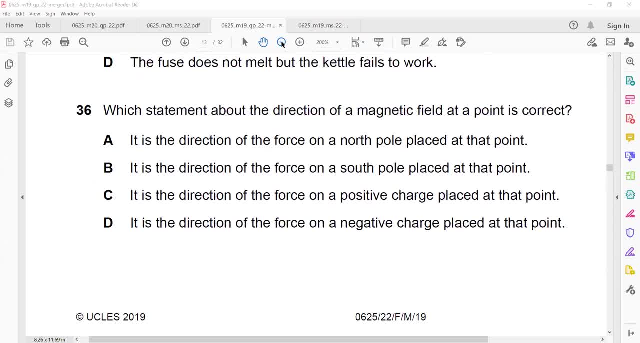 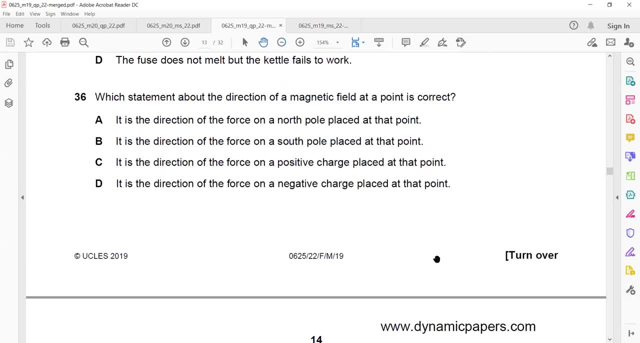 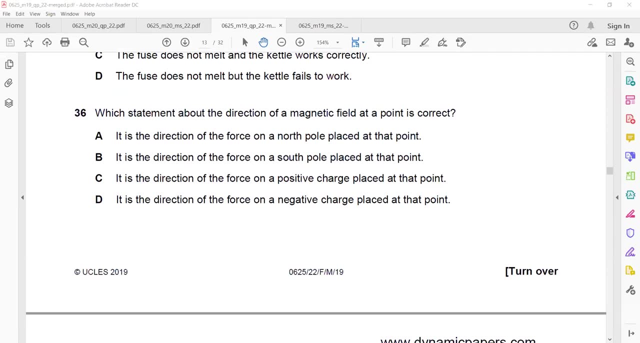 statement about the direction of magnetic field at a point is correct. What's the direction of the magnetic field? The magnetic field it is a direction of the force on a south pole place as at this point that's because the magnetic field it is a direction of the force on a south pole place as at this point that's because The direction in which the south pole and it is a direction of the force on a North Pole place at this at that point. 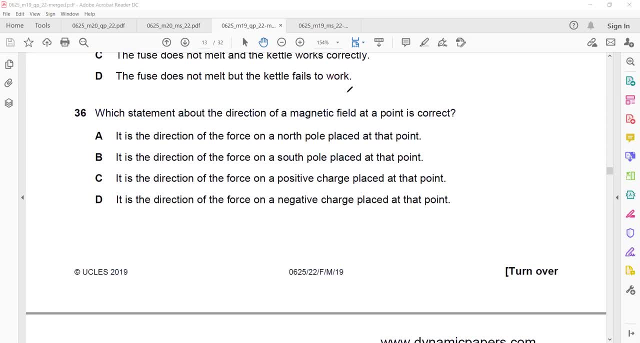 Not a rule. You don't have to use a Fleming the Fleming's left-hand rule is used to find the force on the charge in a magnetic field. But what they mean here in the question they are asking 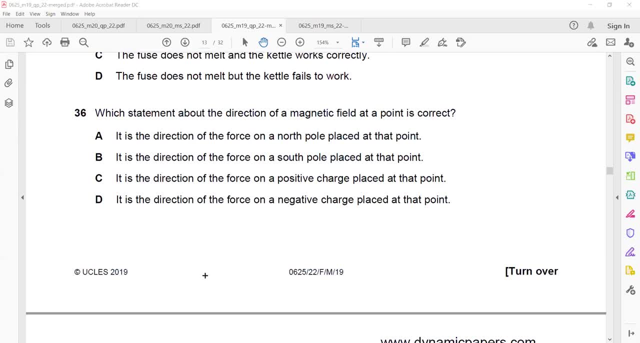 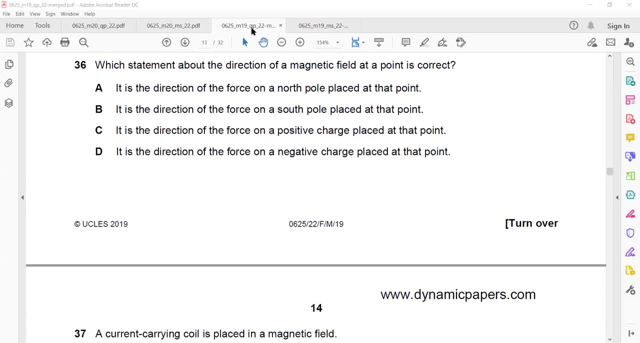 direction of the magnetic field for example if you have have if you're making a ma if you have a magnet so this is a magnet which is having magnetic pole north and south we used to the what is the direction of the magnetic field we say the direction of the magnetic field is from north to south okay now how we can work out the direction of the magnetic field so the 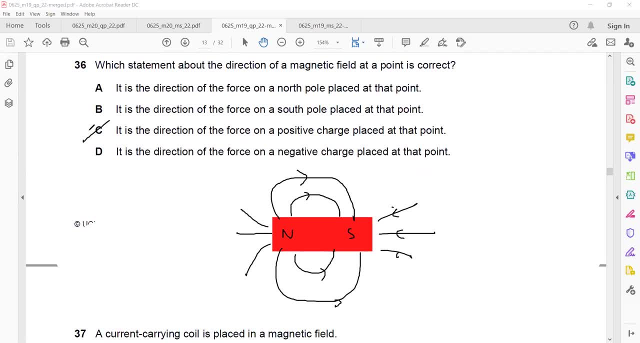 two options c and d cannot be an answer that's about the electric field so a and b can be answered now which one of them c and d is about the electric field not about magnetic 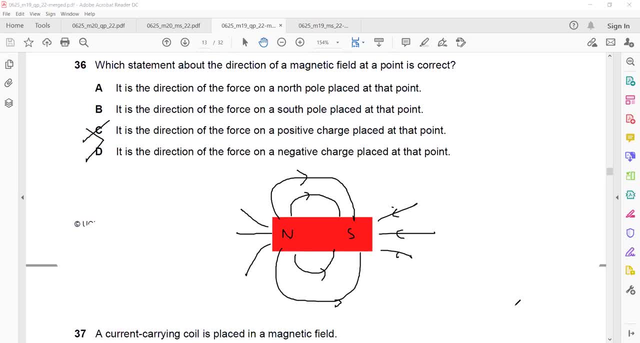 field because the charged particle xp will have electric field so c and d cannot be an answer 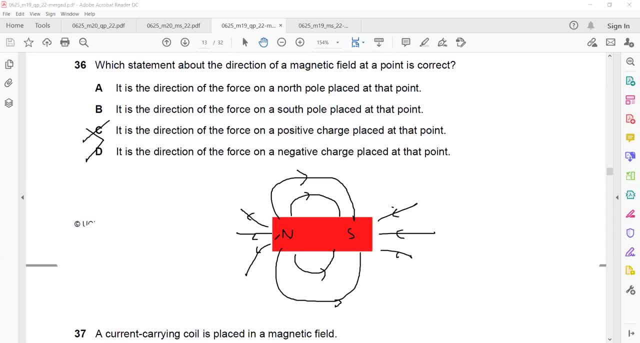 you're left with a and b now in statement a they're saying it is a direction of the force on a north pole place at that point like example if i place a north pole here 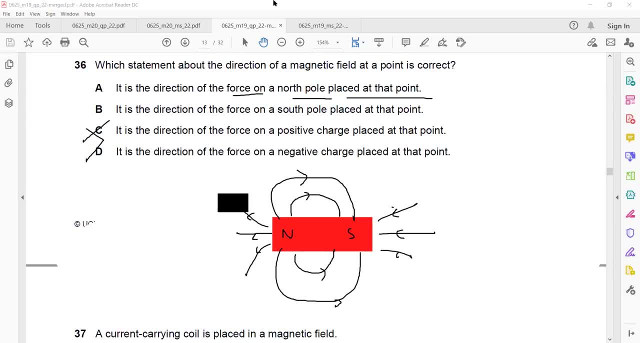 which direction this north pole will move inward or outward 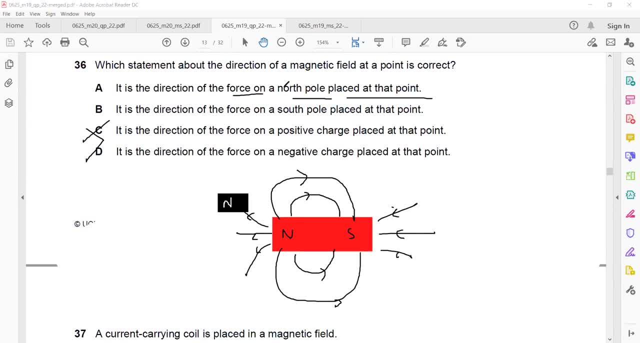 so it will move same as the direction of the magnetic field the north pole will move same as the direction of magnetic field outward and same thing if i place some north pole here so which direction this north pole will move 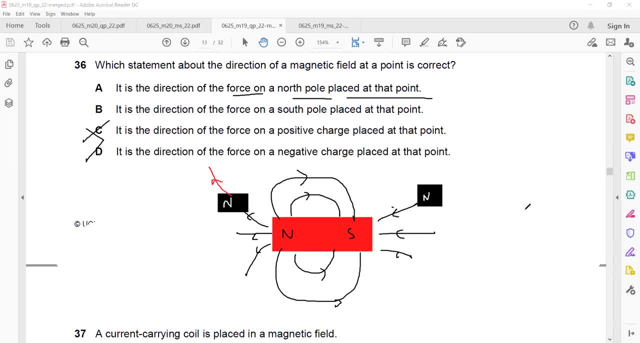 so it will move toward the south so basically the north pole will move same as the direction of the magnetic field so the which statement is correct it is a direction of the force on the north pole place at that point like when we place 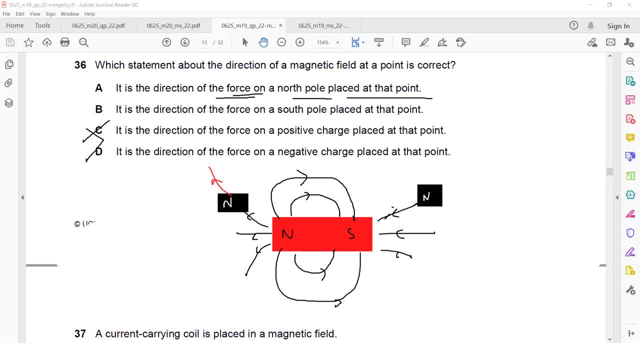 the north pole at any point in the magnetic field it will move same as the direction of the magnetic field so a is a right answer is it clear 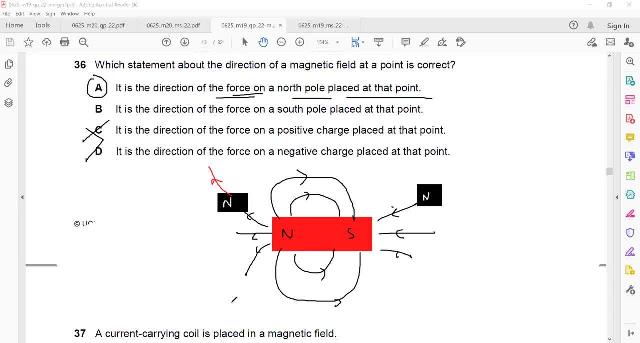 why statement b is not correct because if i place a south pole here so the south pole will move opposite to direction of the magnetic field 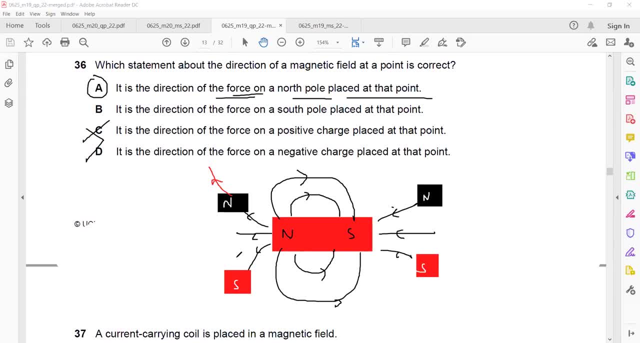 in this case the south pole will move towards and here the south pole will move away so the south pole is actually moving opposite to the direction of the magnetic field 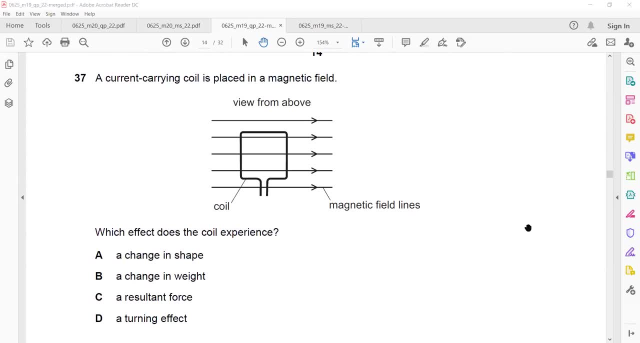 you can see it is short and now we will notice that the north pole will move toward the south pole which direction out for there is a right answer b is the direction of the N method 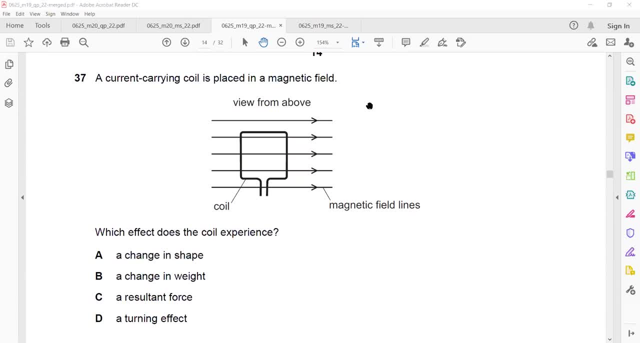 the north pole is located in a the left side so same one time is represented in the middle of the house so the features of both front and rear will not switch so it is just a general statement like very simple so it is just a general statement